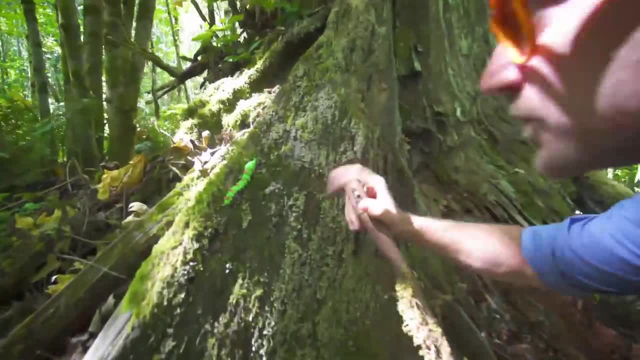 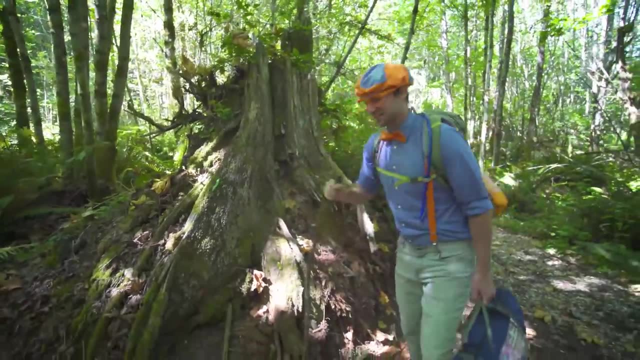 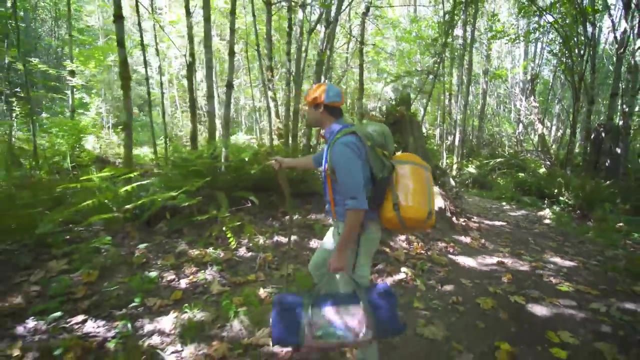 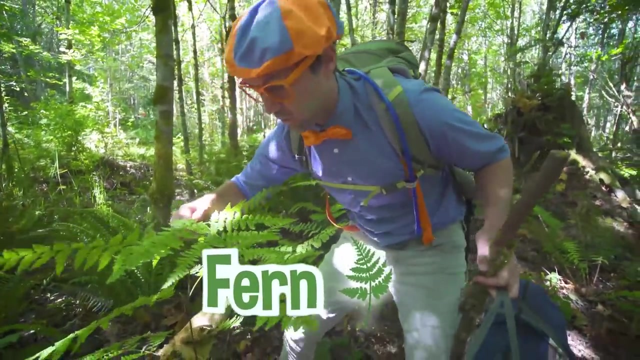 Whoa, Look at this, An insect That looks like a caterpillar. Whoa, Hello, caterpillar. All right, We should probably keep going so we can get to our campsite before dark. Hey, Look at this beautiful plant. See this, This is a fern. Wow, Look at it. It's the color green. 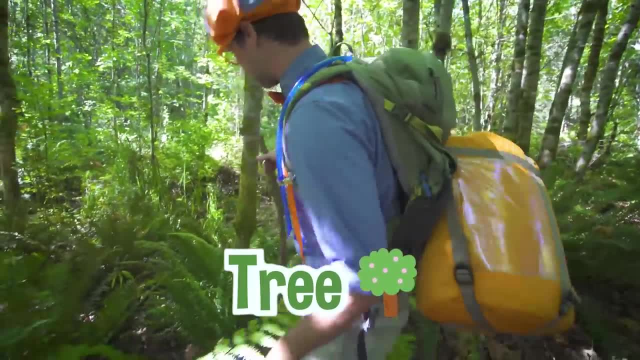 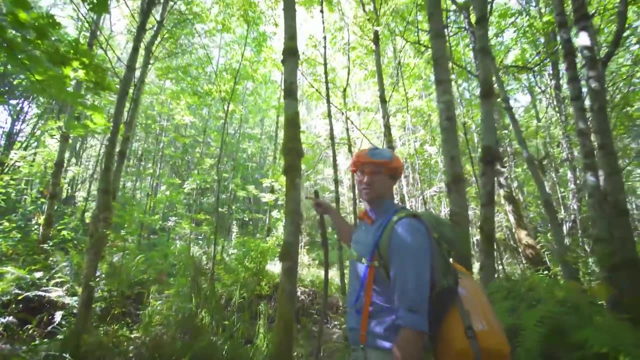 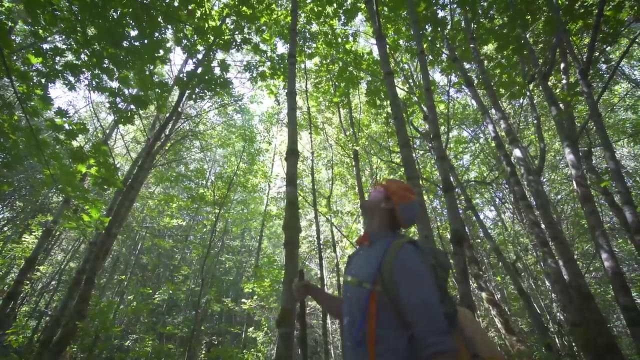 Hey, Here's a tree back here. Oh, excuse me, fern, Look right here, This is a tree. Yeah, you know what a tree is. There's some bark on it and also some moss. Look how tall the tree is. It's a lot taller than me, huh. 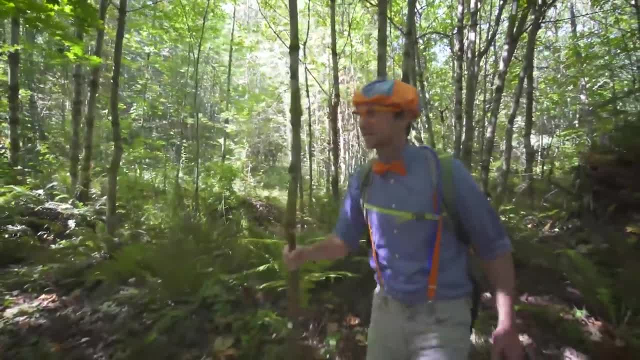 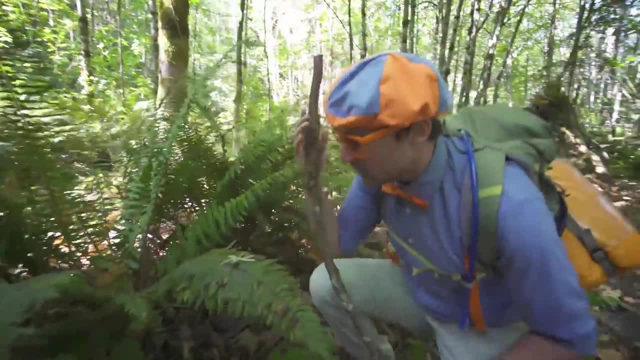 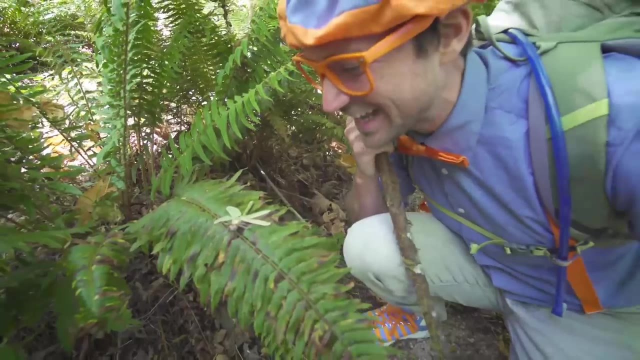 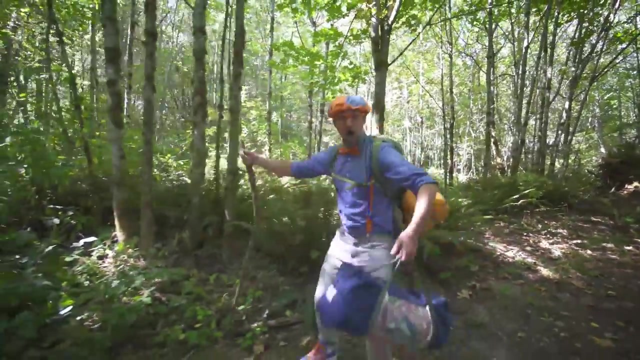 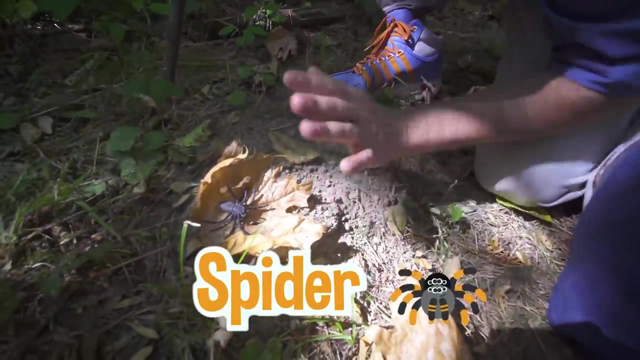 All right, Let's see what else we can find here. Wow, Hey Look Another insect. Hello, That looks like a dragonfly. Hello, dragonfly. How are you doing today? Okay, Let's continue on. Oh Look A spider, Hey spider. Are you having a good day? 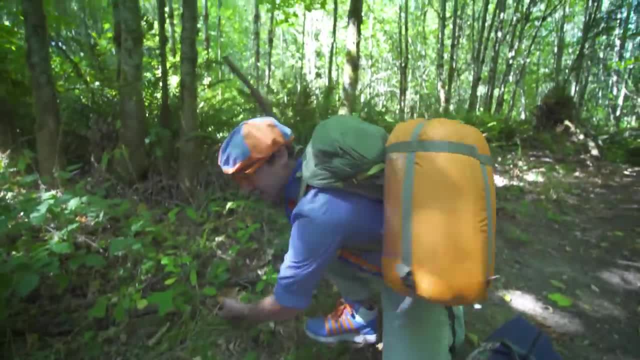 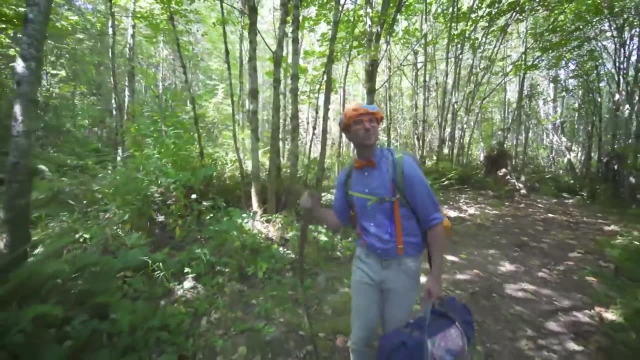 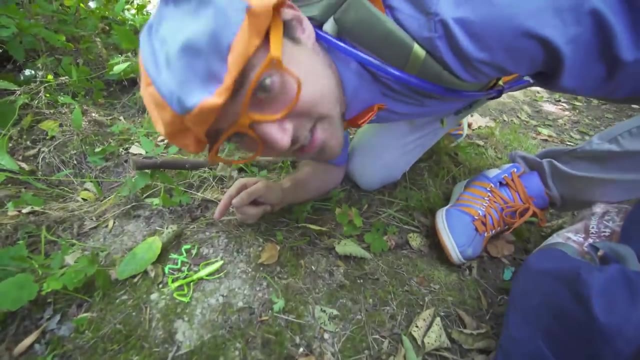 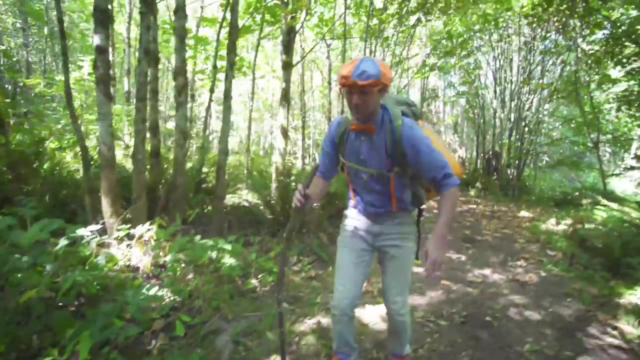 Hey, Here, I'm going to move you right over here, so then I don't step on you. All right, Here we go. Wait a second, We have some more insects. What kind of insects are these? These are praying mantises. Wow, They're so cool. Look, This is what they look like. 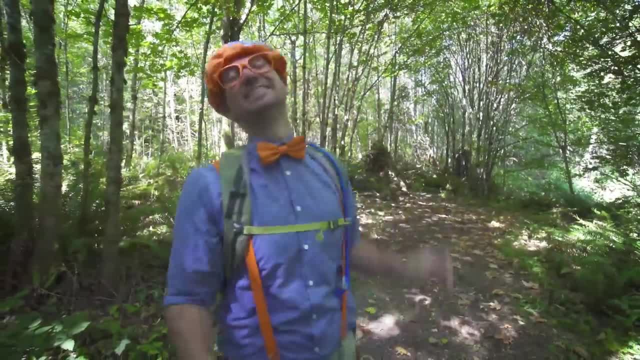 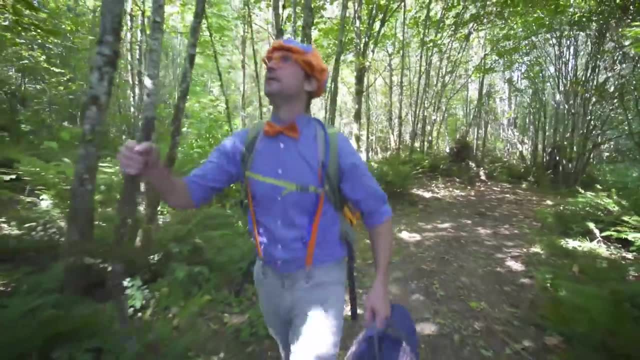 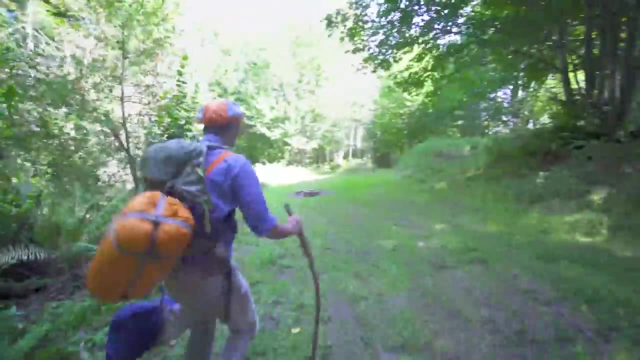 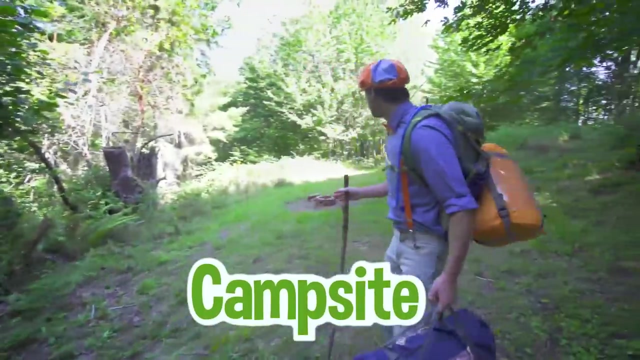 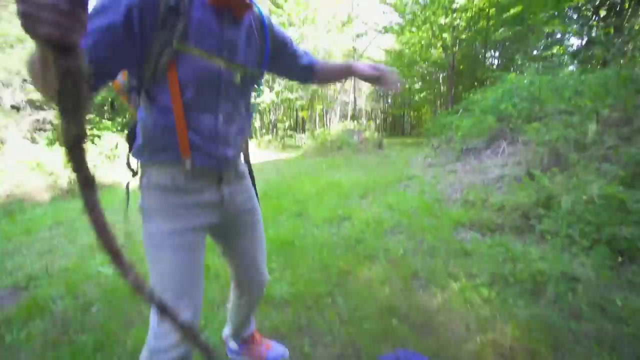 Hello, I'm a praying mantis. Hi, Okay, I think we're almost there. I'm getting a little tired. Whoa, Check it out. This looks like the perfect campsite. Wow, All right, Let's go over here and then take off all of our equipment. 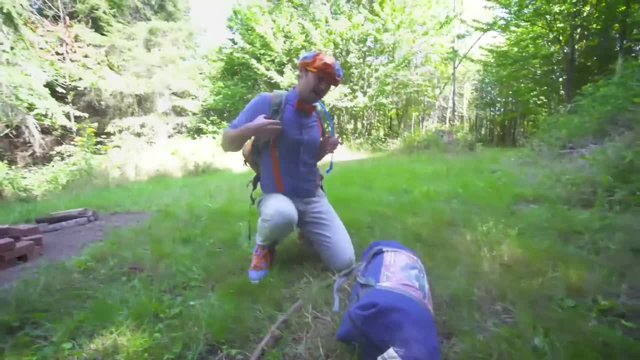 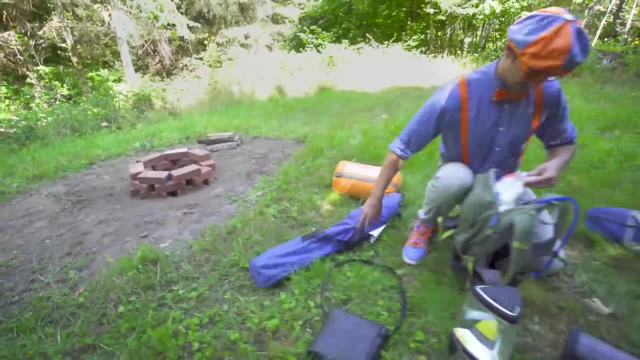 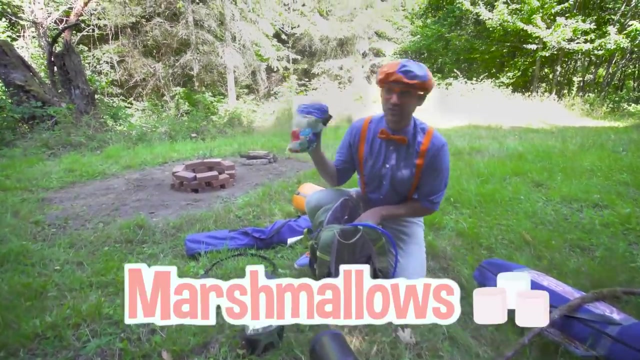 There we go. There we go. Oh, I think I need some water. Ha ha ha. Hmm, All right, I'm just unpacking all of my camping gear. Yeah, Oh, can't forget the marshmallows. Yeah, this is for the s'mores later. 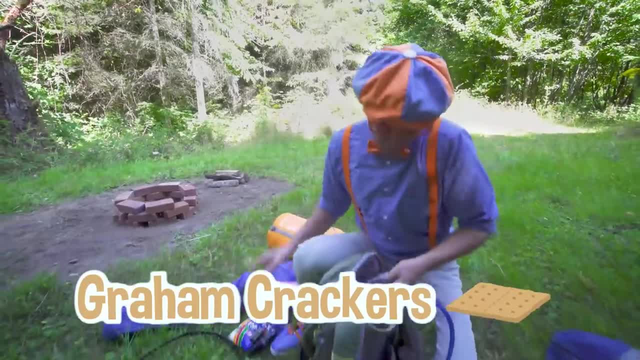 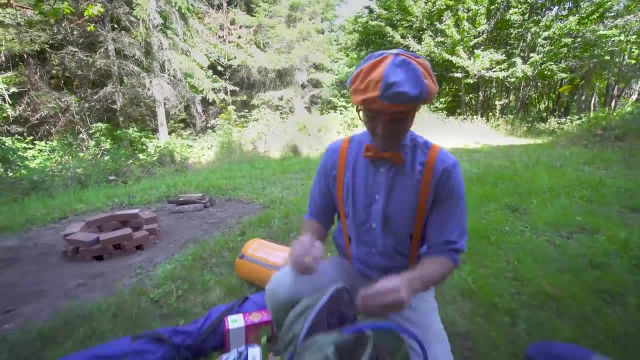 Ooh And the graham crackers. Ooh And the chocolate. Have you ever had a s'more before? S'more before, That rhymes, That's silly. Ooh And my s'more roaster. Ha ha, Ooh And my coloring book. 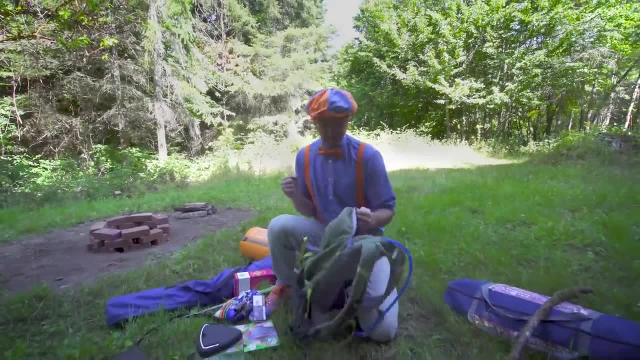 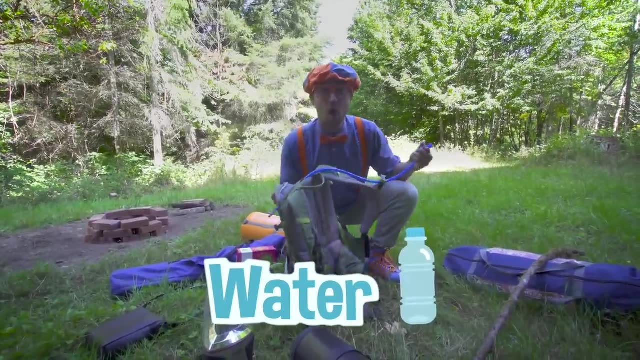 So then I can color in the tent later. This is going to be fun, All right. What else do we have here? Well, we have our water right here. You definitely need to bring water, Yeah, So then you can hydrate. 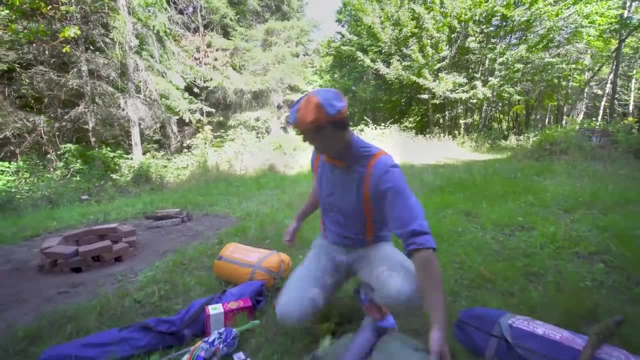 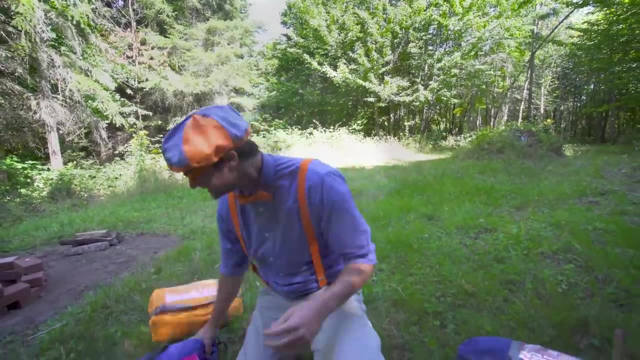 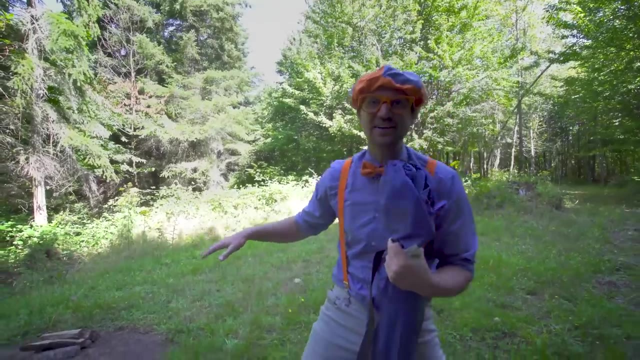 Hmm, Yum, I love water. Ooh, I have my orange sleeping bag- This is going to be so cozy- Ooh- And a blue chair. I'm going to set this up later next to the fire, so then I can enjoy watching the fire. 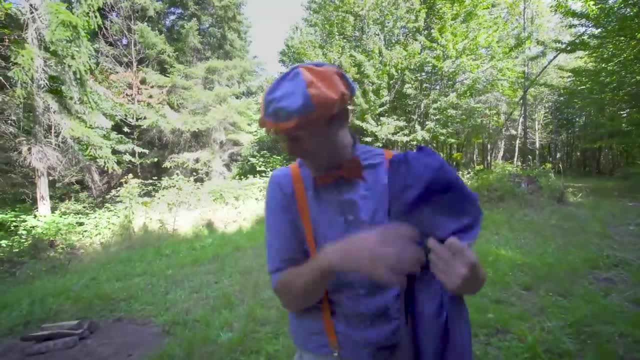 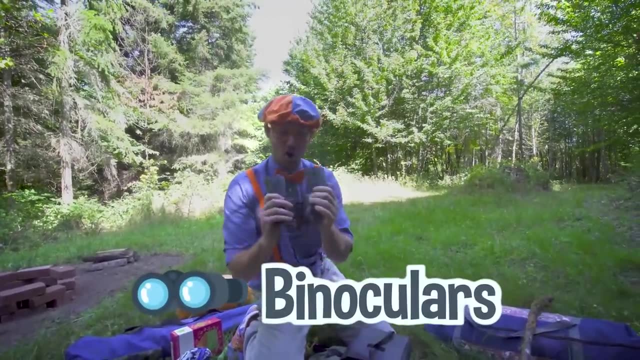 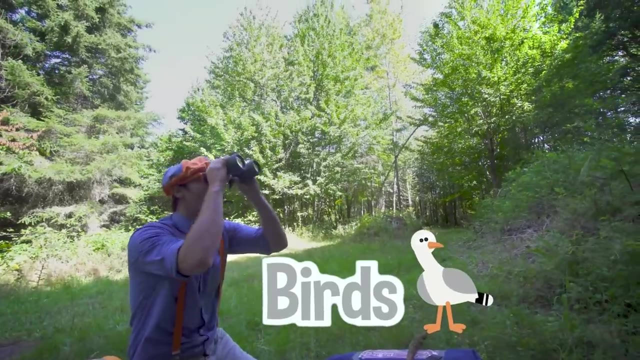 And so I can roast my s'mores. Ha ha ha. Okay, All right, We have a pair of binoculars. Whoa, Look at them. This is so. then you can see things from far away, like birds. Whoa, There's one right there. 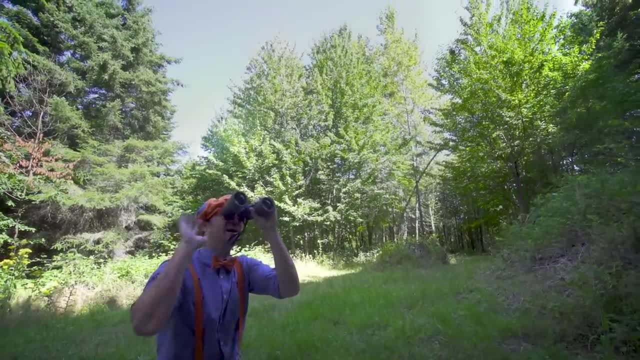 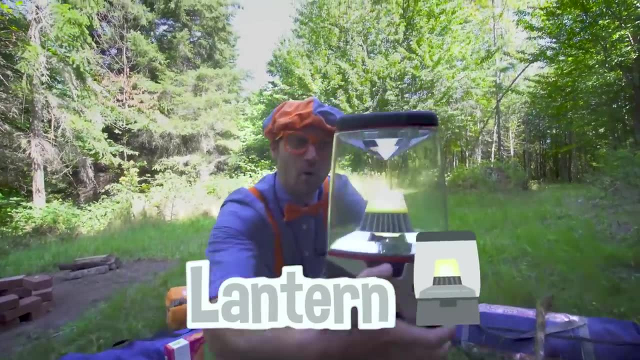 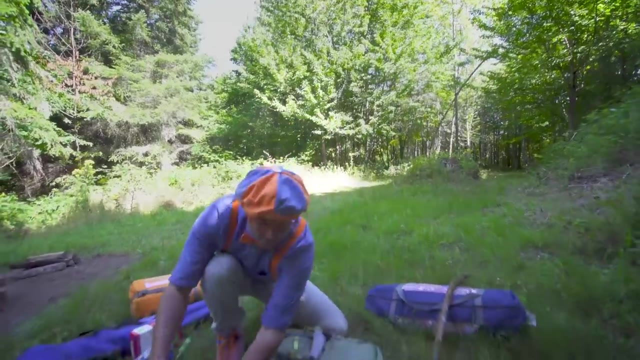 Ha ha ha, Hello birdie, Hello, All right, Set those down right here. Ooh, And a lantern, Check this out. Whoa, It's a really bright light. So then at night you can see when it gets dark. 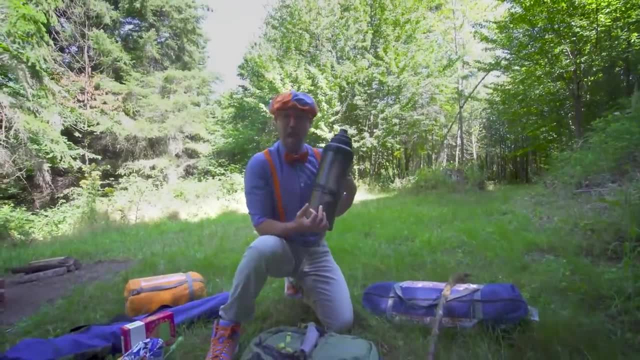 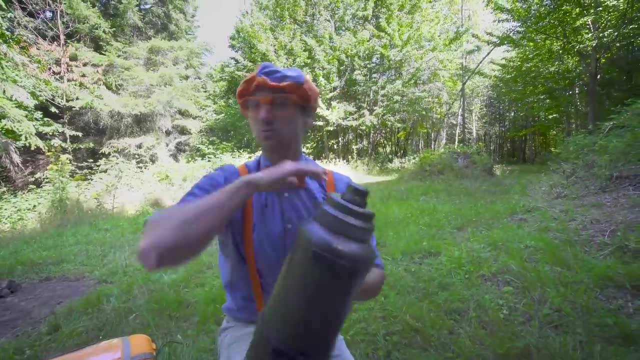 And a giant one-gallon thing of water. So then, when I'm ready to go to bed, I can put it on the fire. So then we don't start any forest fires. That would be really bad. Oh yep, My camping stick. 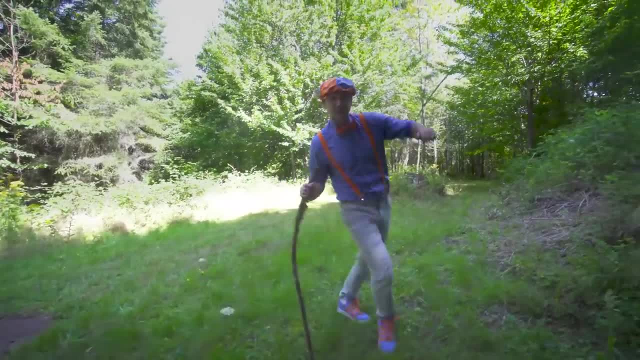 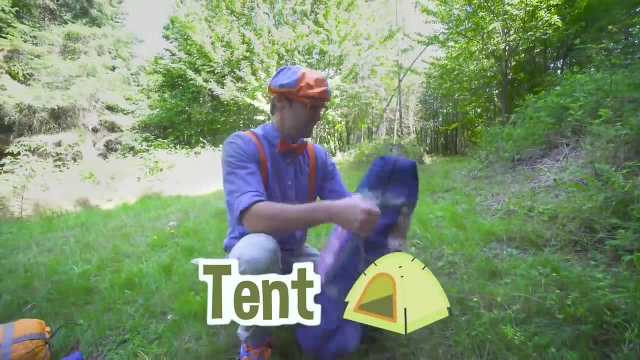 Ha ha. Yep, You saw that later Helps me with my balance while I'm walking through the trails. And, last but not least, my tent. Yeah, It's like your house, But when you're in the wilderness, yeah, you need a place to sleep, right. 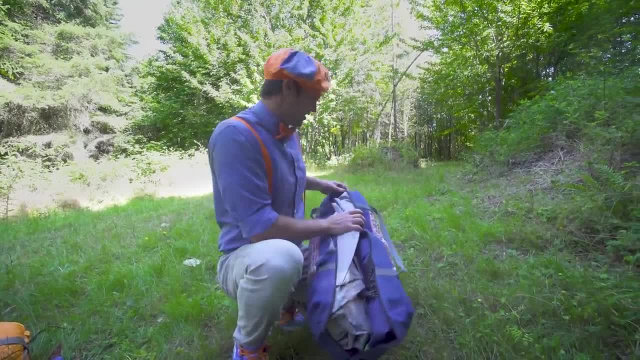 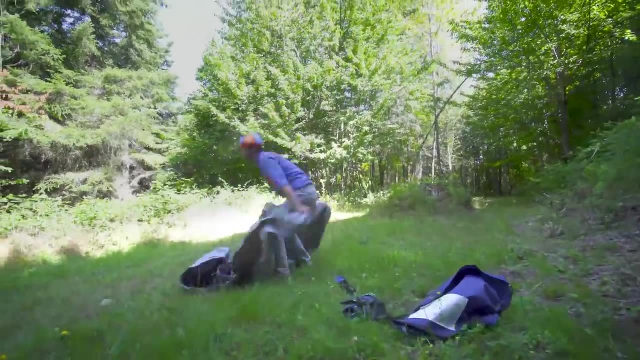 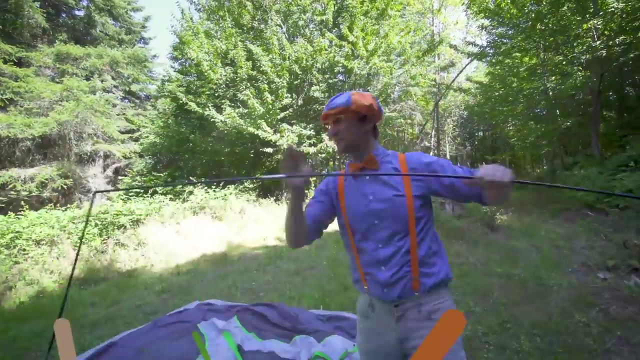 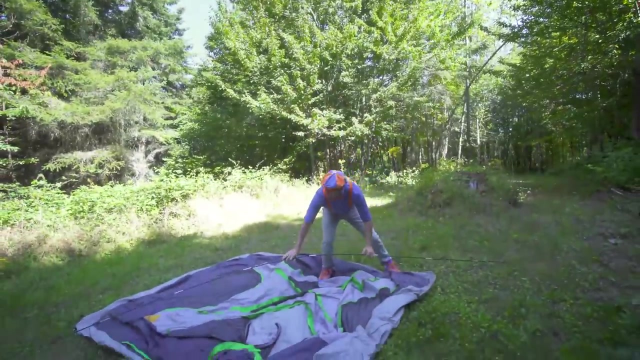 Yeah, All right, Let's open it up. I think I should pitch the tent. All right, Here we go, Here we go. It's like a puzzle, Whoa. This goes from one end to the other, And then I have another one of these. 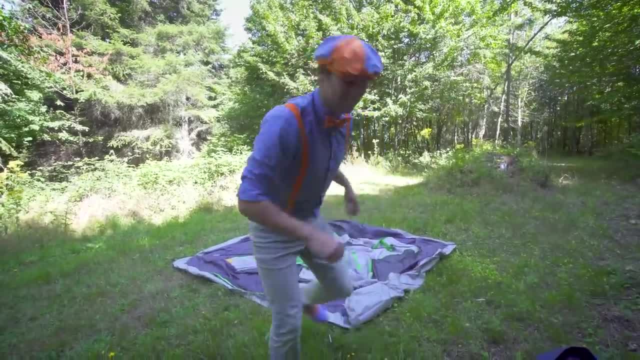 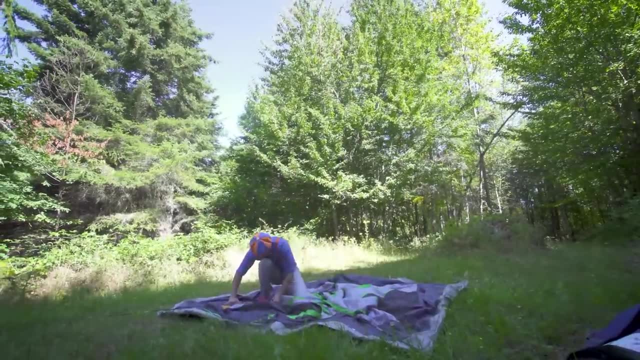 Now for the fun part. You raise the tent. I can't get the rest of the tent. I can't get the rest of the tent. I can't get the rest of the tent. This is my favorite thing about camping. It's a home base. 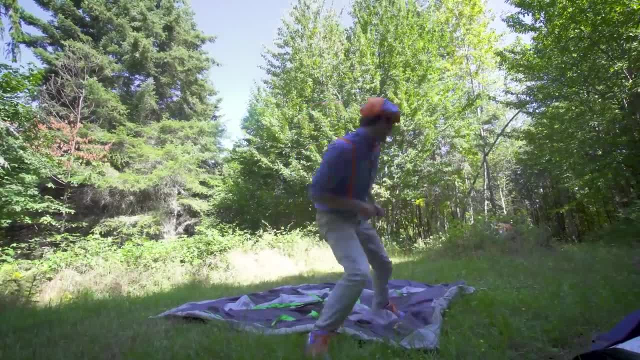 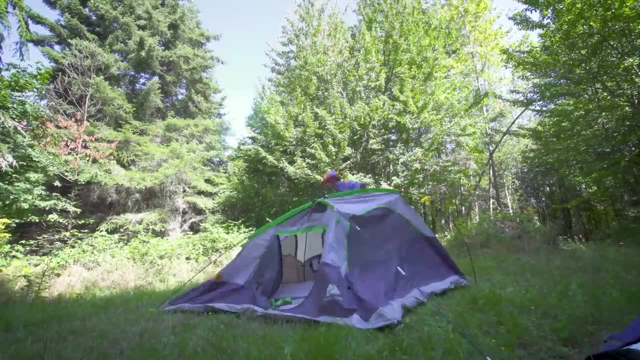 It's not really a tent, But it's a home base. Let's go. Dad, did you get the tent? Yeah, I did. All right, Let's put the tent down. Okay, All right, Let's put it down. 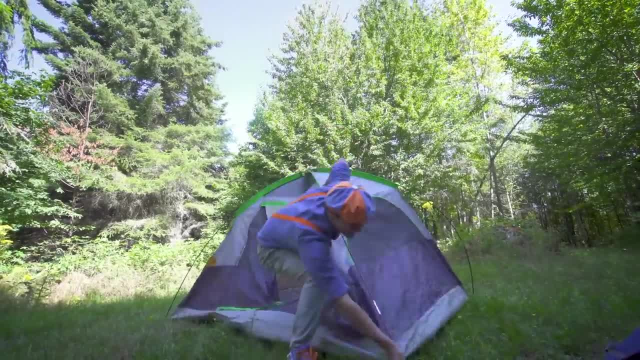 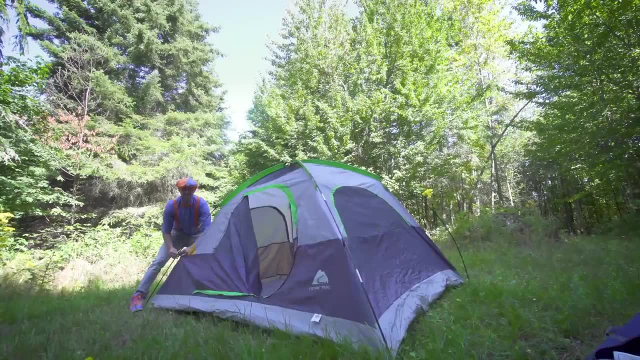 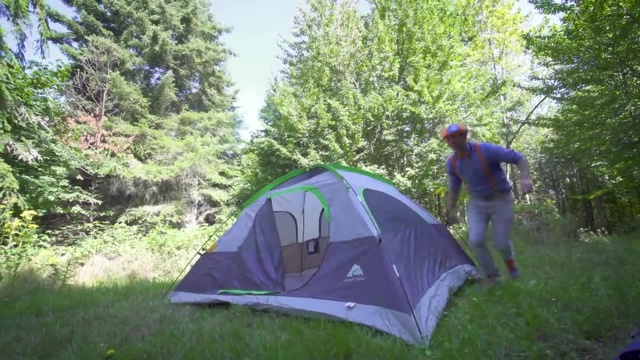 All right. So I'm going to add a tent, But you guys can do it. All right, I'm going to put the rest of the tent down. How does it look? Looks really good, huh Ta-da. Now we can sleep inside. 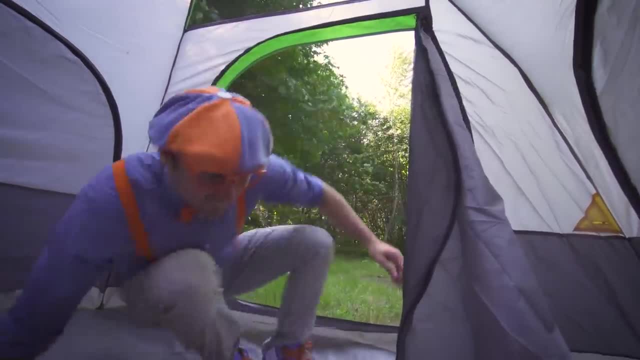 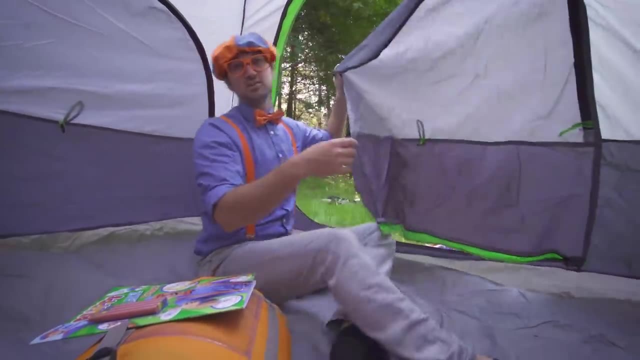 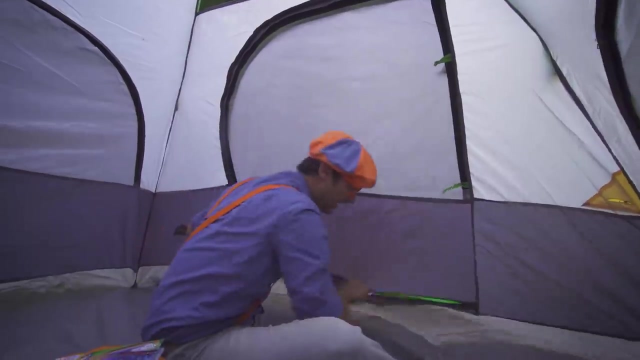 Whoa, I forgot to take off my shoes. Yeah, you take off your shoes before you get in the tent, So then you don't track in any dirt. All right, let's zip it up. Whoa, this is so much fun. 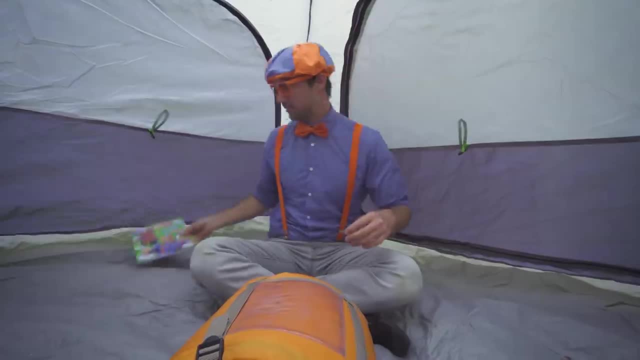 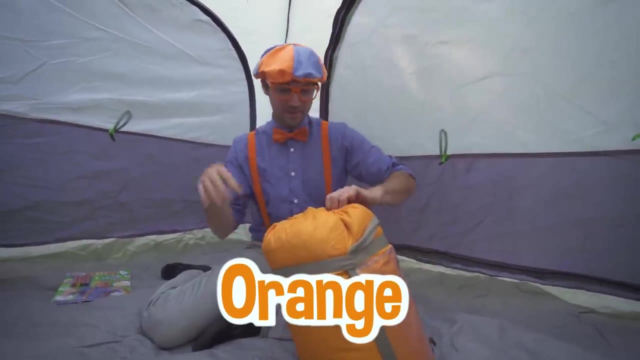 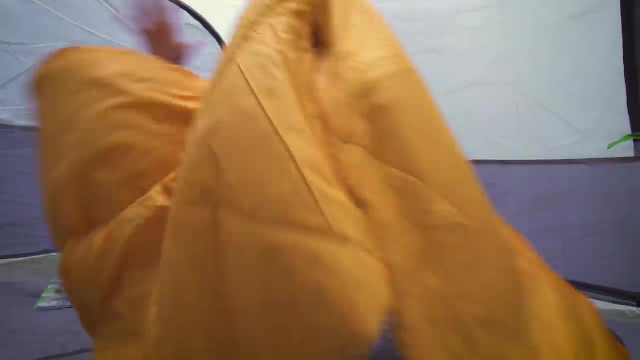 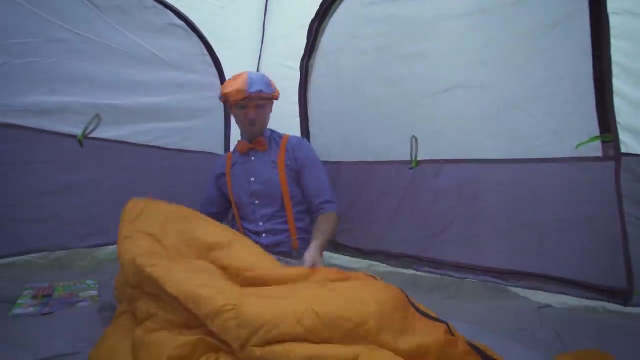 Okay, coloring book I'll put right here. First I need to take out my sleeping bag. Yeah, my orange sleeping bag. Whoa, Whoa, Whoa, Whoa, Whoa, Whoa, Whoa. Okay, put that right over there, and then here we go. 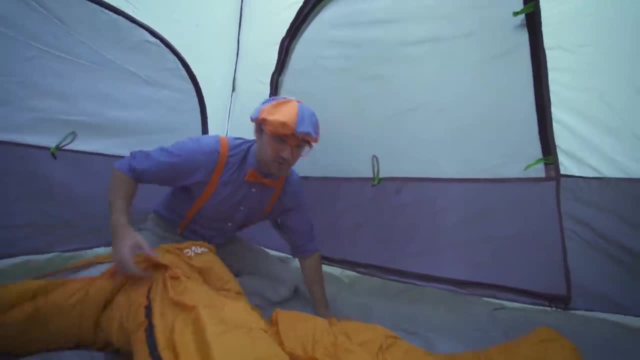 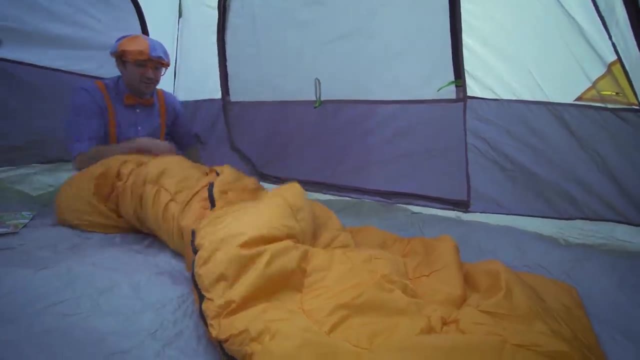 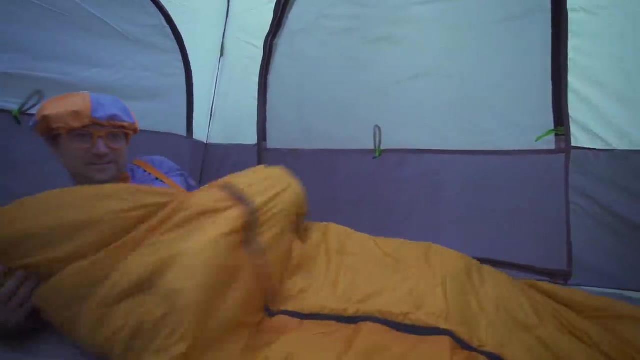 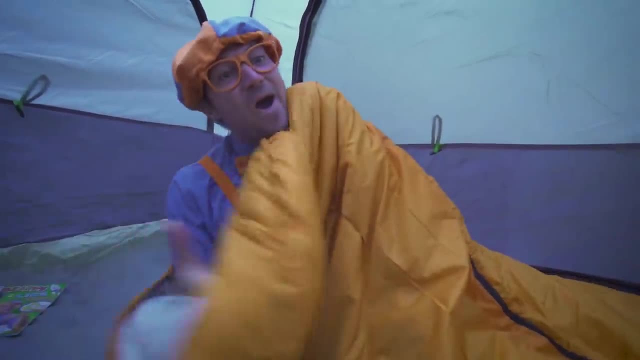 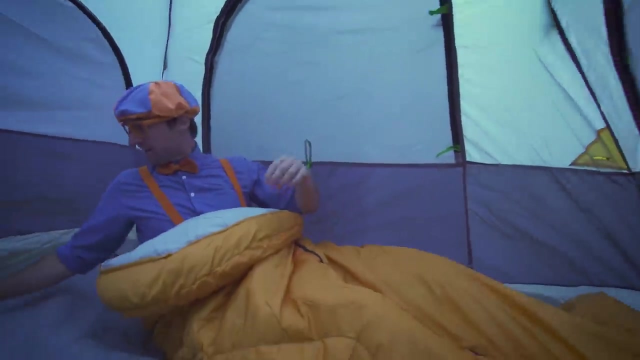 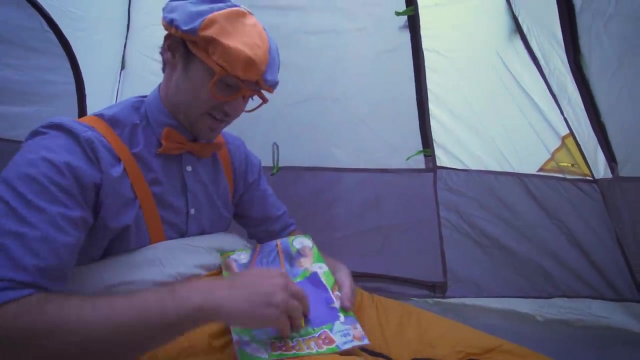 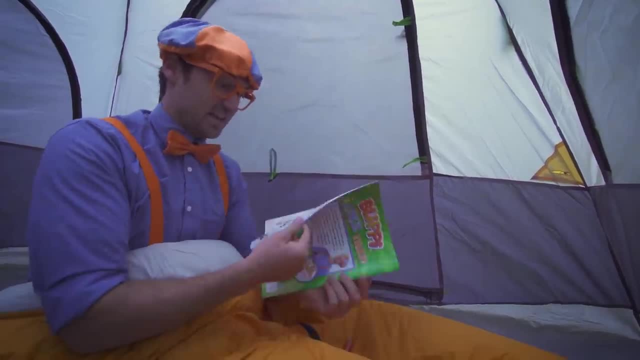 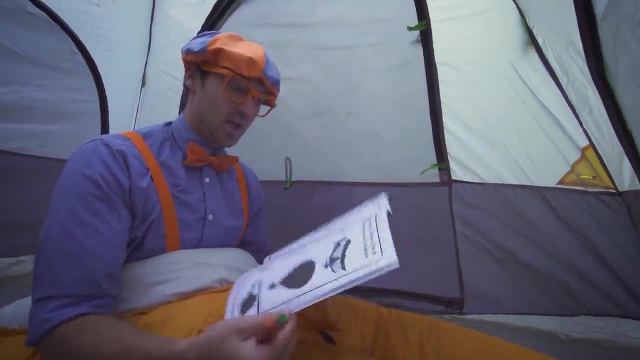 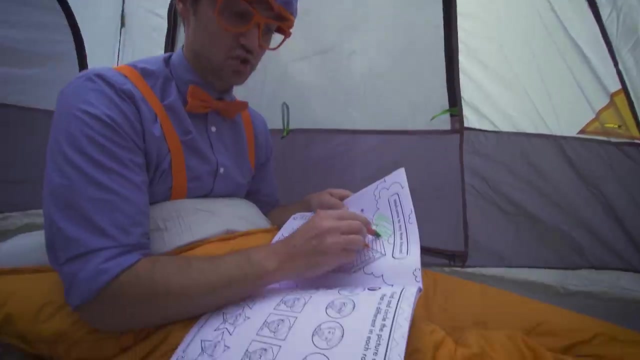 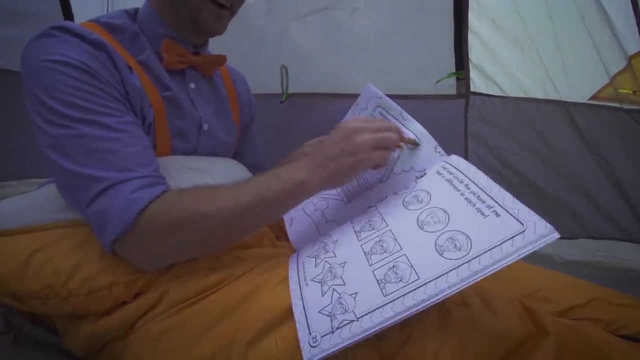 I love coloring when I go camping, because coloring is something fun that you can do, because it's creative. It's really great. Have you ever colored? Yeah, what about drew something original? because this, you can color this tree. yeah, look blippy. welcome to my tree house. oh, there we go. yeah, you can color something that's already there. 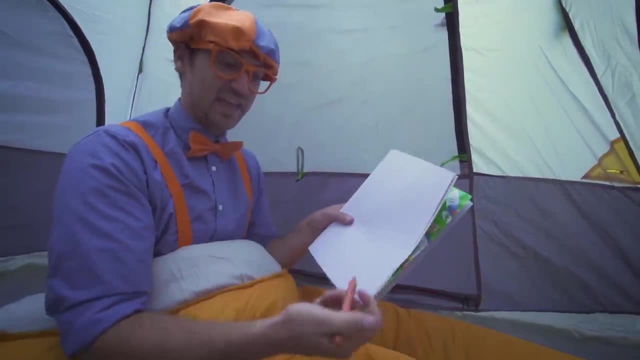 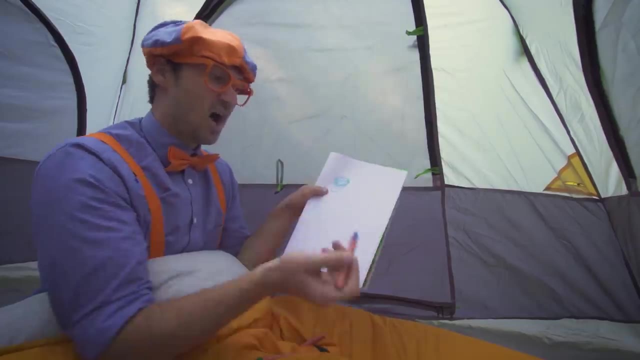 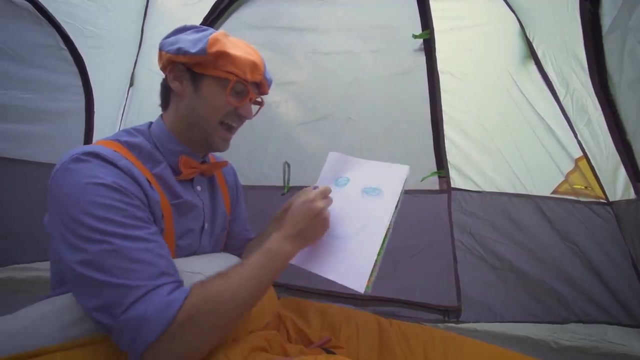 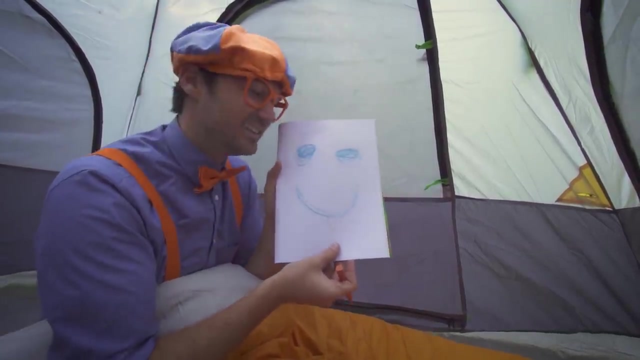 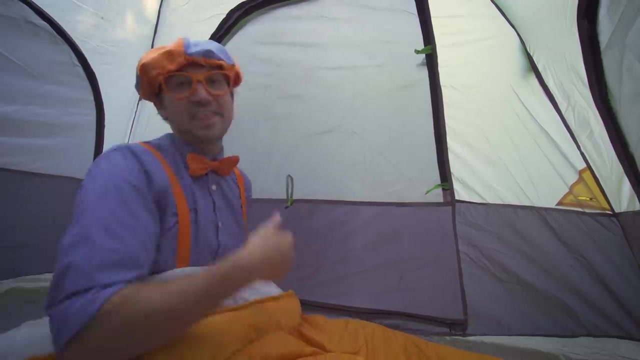 or you can find a blank page and then you can draw something original like blue one, two circles and a smiley face with a tongue. okay, well, what are we doing in here? we're camping. there's so much fun things to do outside. i think we should go outside and play some hide and seek. what do you say? 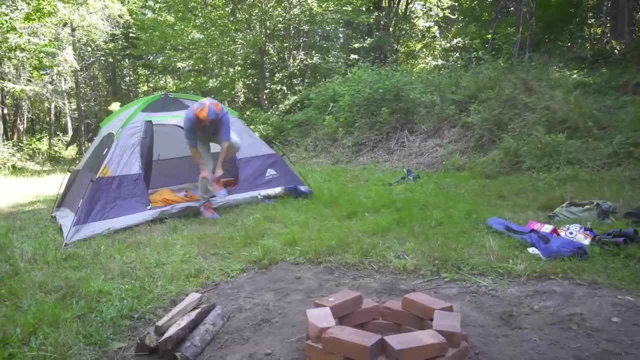 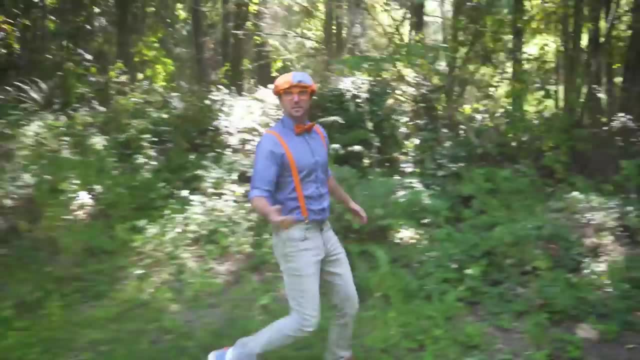 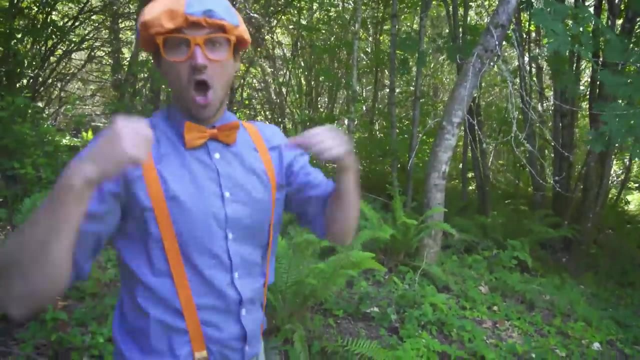 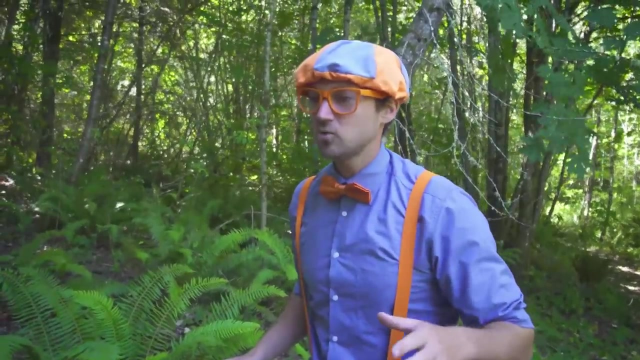 oh, i love playing hide and seek. okay, to play hide and seek. one of us needs to hide and one of us needs to seek. yeah, okay, i'll hide and you seek, all right. so, uh, all right, ready, let's uh count to five and close your eyes. ready, one, two. 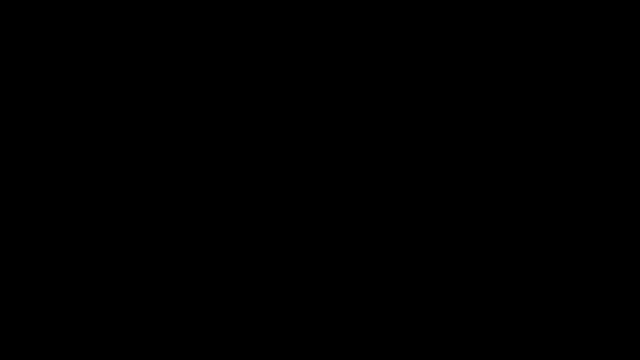 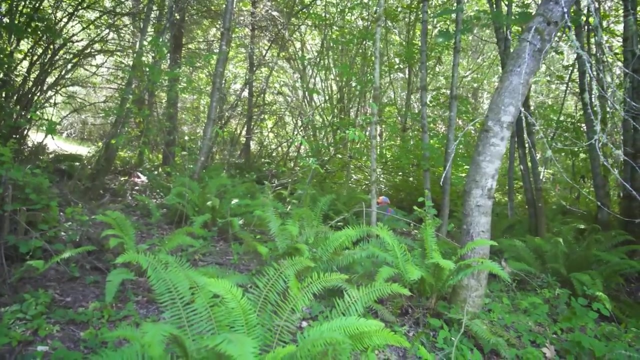 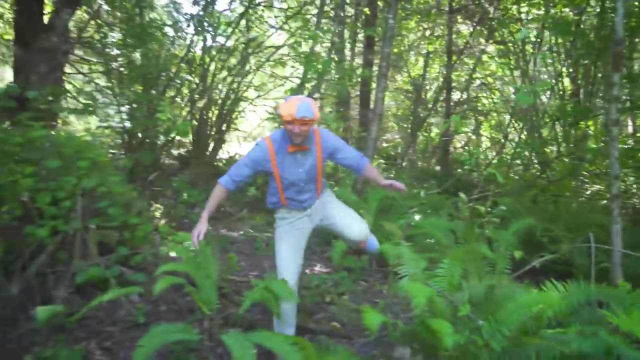 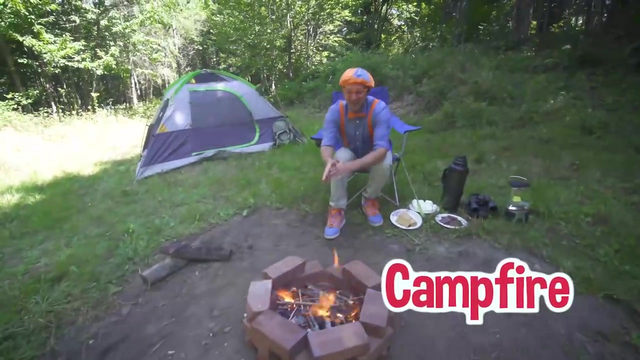 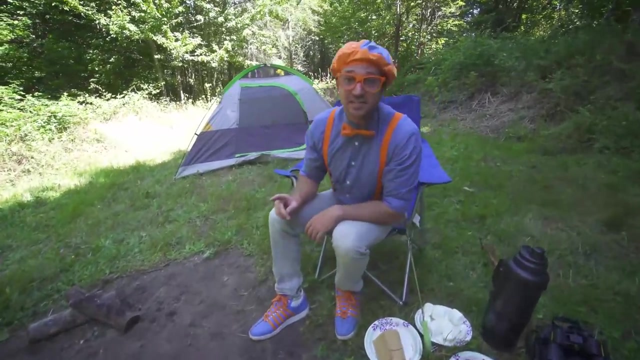 three, four, five, hello. do you see me? do you see me? yeah, hey, i'm right here. good job, that was so much fun. this campfire is so nice. well, anytime there's a campfire, you need to be very safe on your own, for where? yeah, i made this campfire and i'm actually a grown up, if you didn't know. 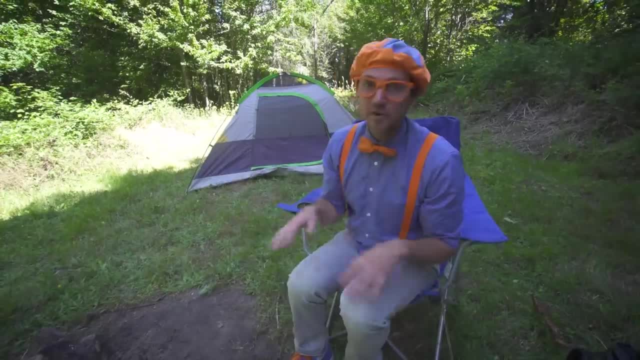 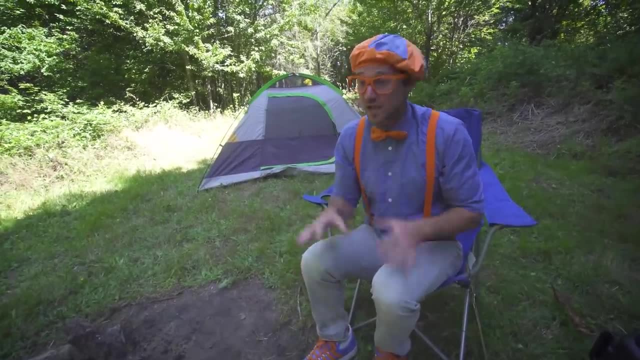 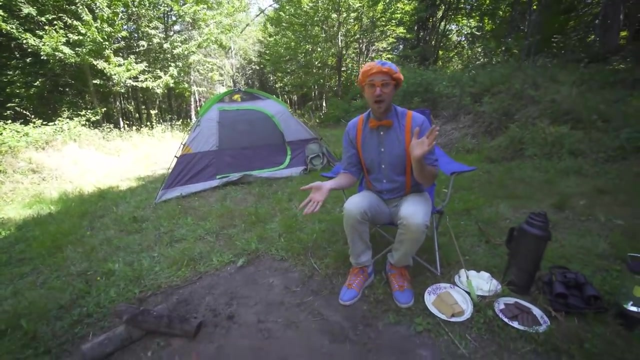 actually a grown-up if you didn't know. children should never make their own campfire, and if there is a campfire, you should always have a grown-up around you. if they're not there, you should tell someone: hey, grownups, someone should come near the campfire. 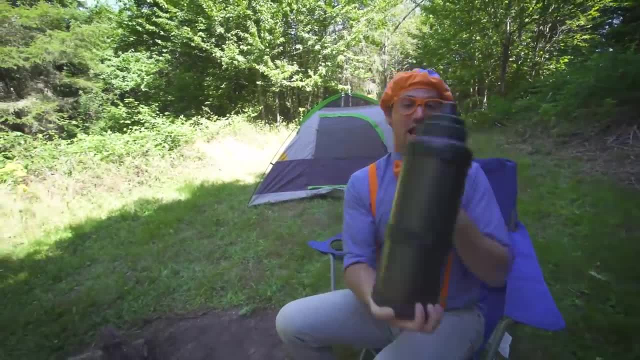 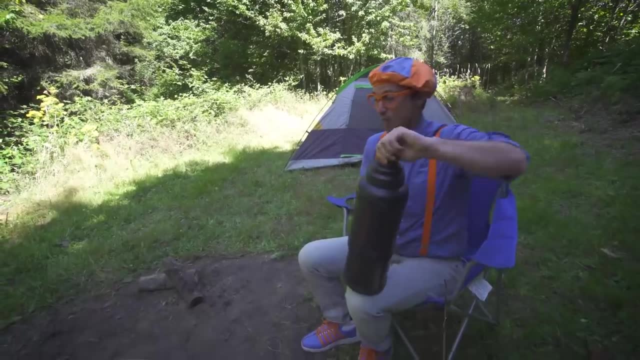 and hey, speaking of near the campfire, remember earlier i had this gallon of gallon of water. Yeah, it's about 3.8 liters. Yeah, you want to make sure you have water near a campfire, just in case, if it gets out of control, you can pour some water on the. 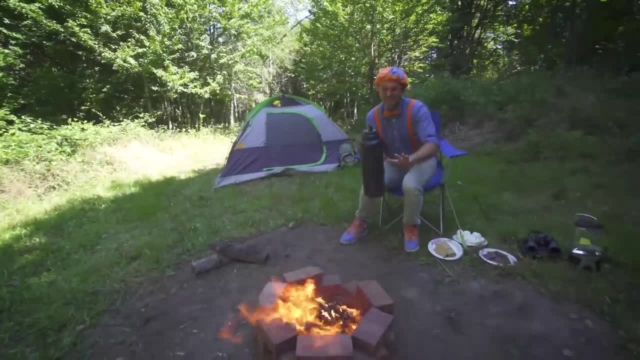 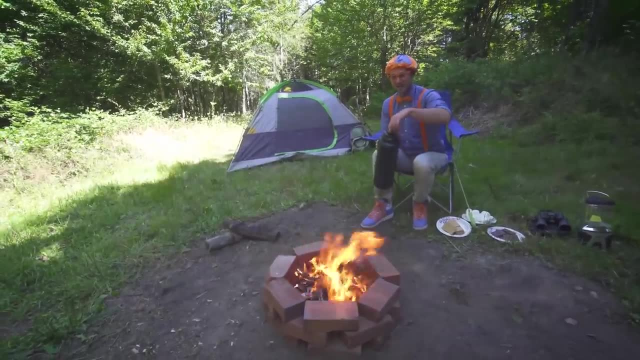 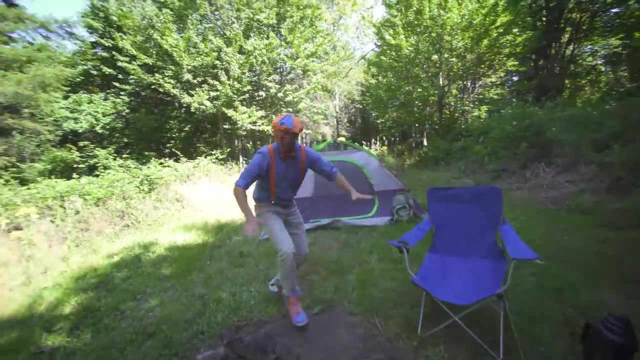 fire and put it out, But it's actually in a controlled environment. See this fire pit that I made it in. Yeah, yeah, it's not going to catch anything on fire. And that's another thing: You want to make sure there's no branches or leaves or anything above it or around it. 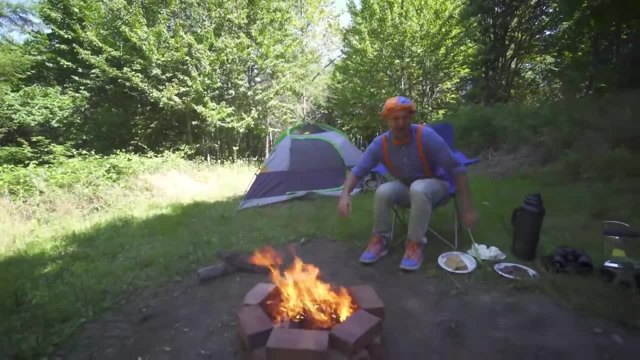 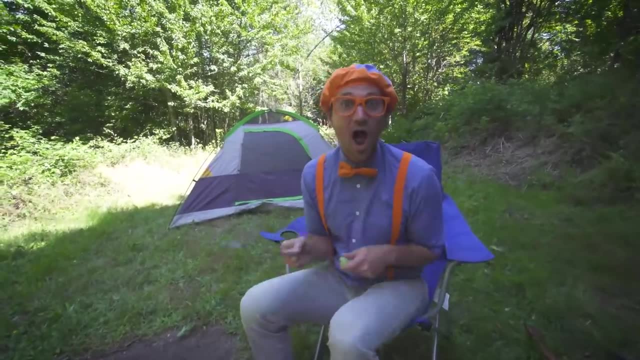 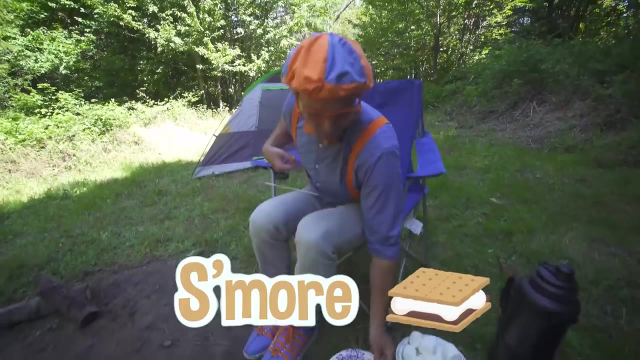 Yeah. So now that we have a safe campfire, I think it's a perfect time to make some s'mores. Have you ever had a s'more before? They're so yummy. After a good, healthy dinner, you can have a s'more Here. check it out. So we got some graham crackers, Yeah, and this. 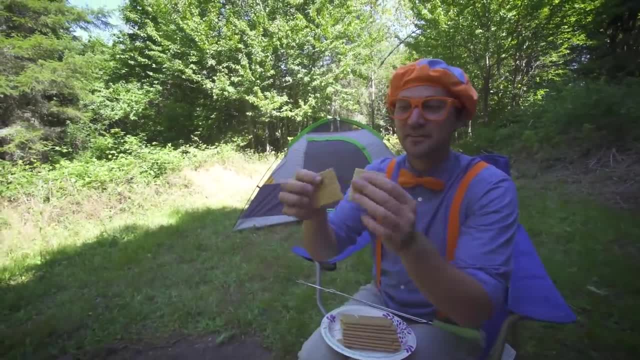 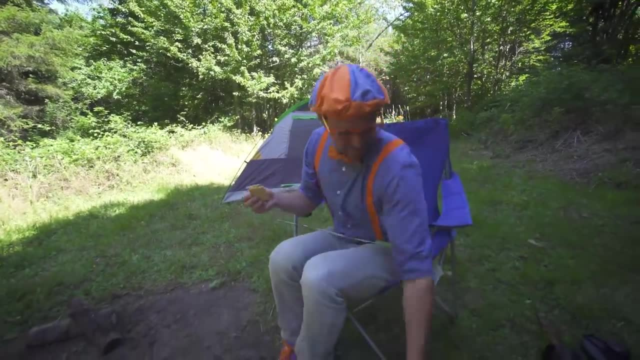 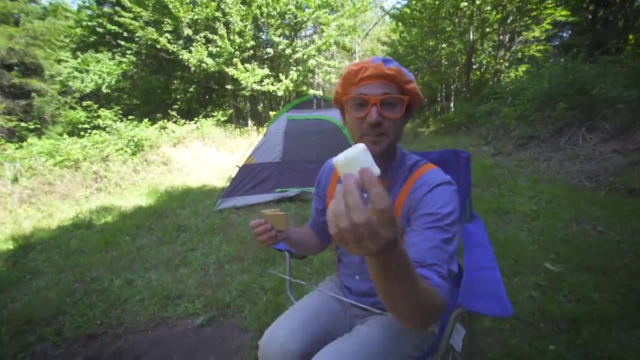 is a rectangle, But you split it in half And now you have two squares. Yum, Okay. And then you also have a cylinder. Yeah, that is a cylinder. See that shape? But that's not what it's called. 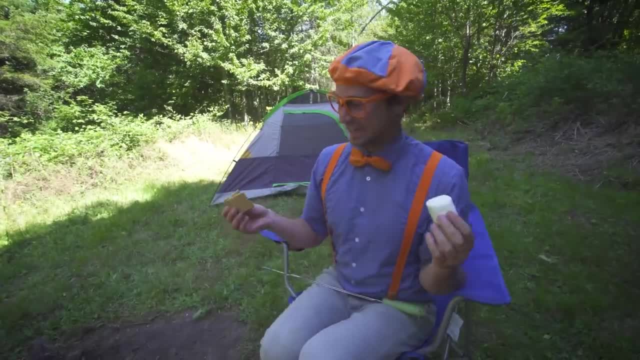 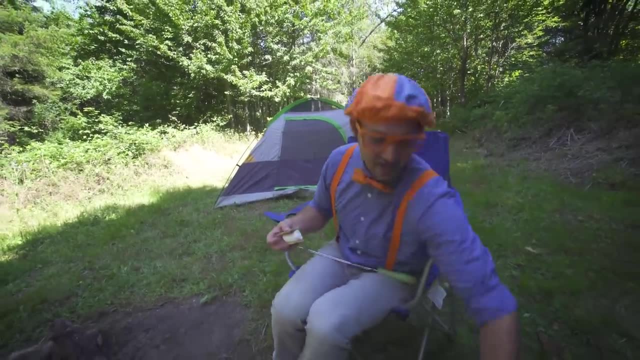 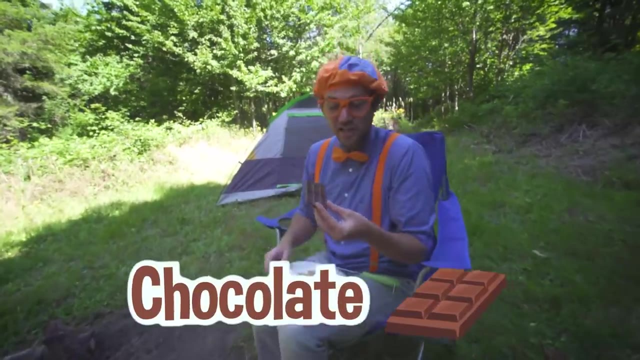 This is a marshmallow And they're so yummy. Okay, I'll put that right there for now. Okay, Actually, you know what? I should probably be a little bit more organized With this round white plate. All right, Then see this yummy chocolate. All right, That's. 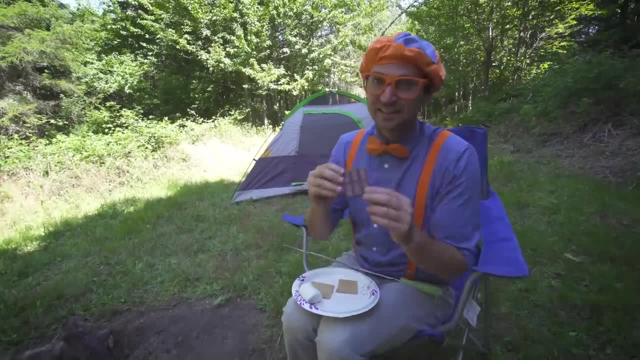 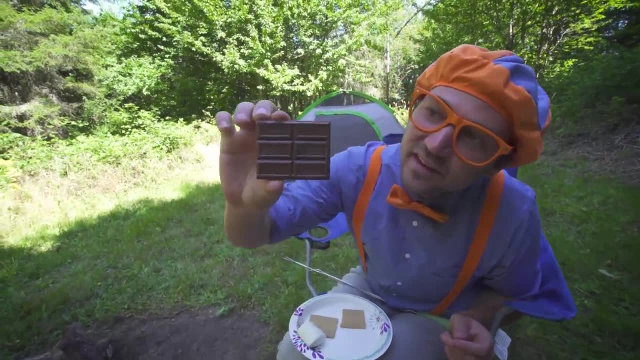 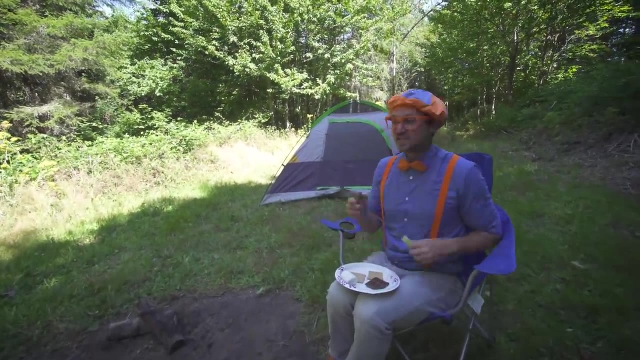 the third and final ingredient of s'mores. I love chocolate, Yeah, And there's actually small rectangles. Do you see them? Yeah, small rectangles, And it actually makes a bigger rectangle when they're all connected. All right, The first thing you need to do is put your 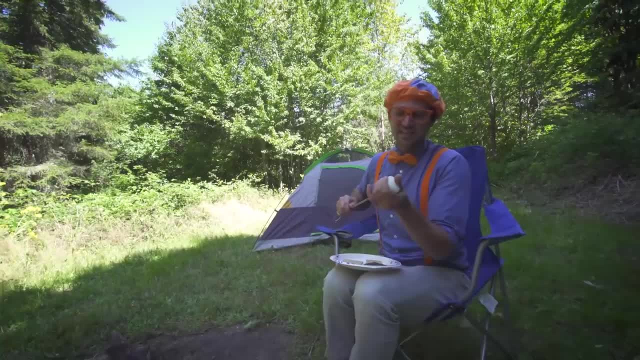 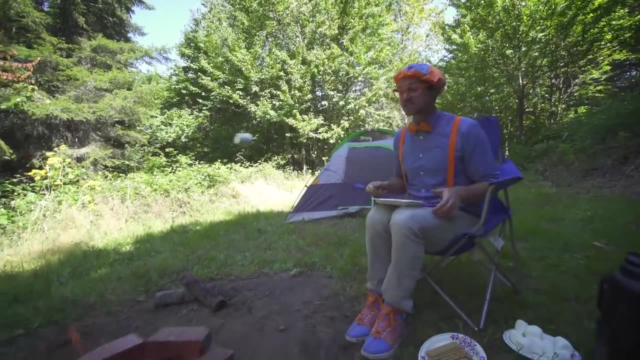 malo in your marshmallow. Okay, You get your marshmallow on your stick, So then you do not hold it next to the fire. That would be really bad. You want to stay a safe distance away from the fire? Yeah, Perfect. 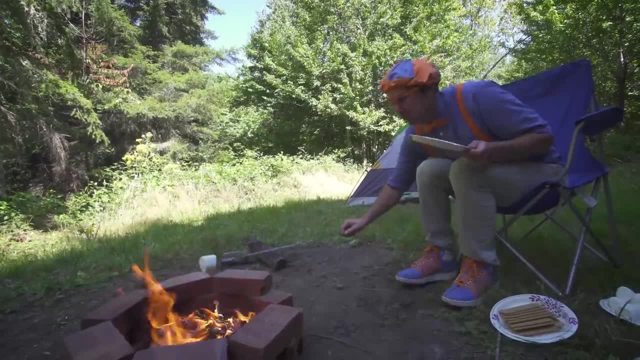 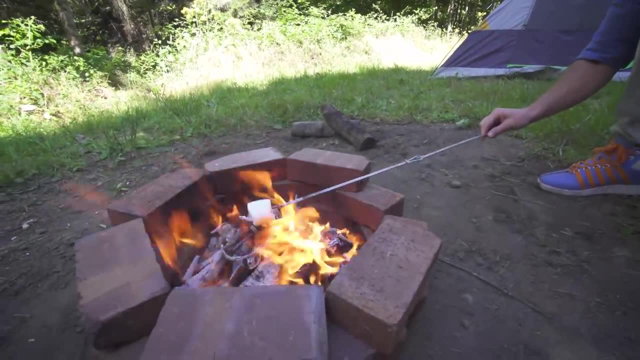 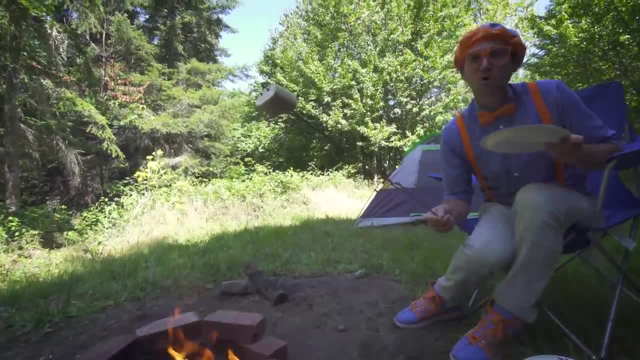 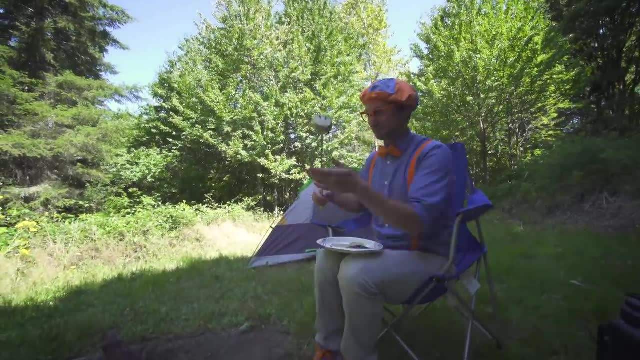 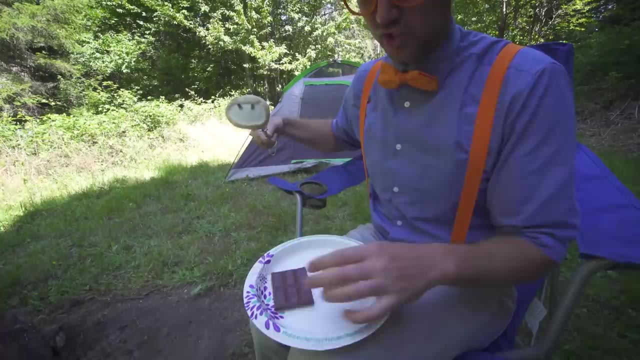 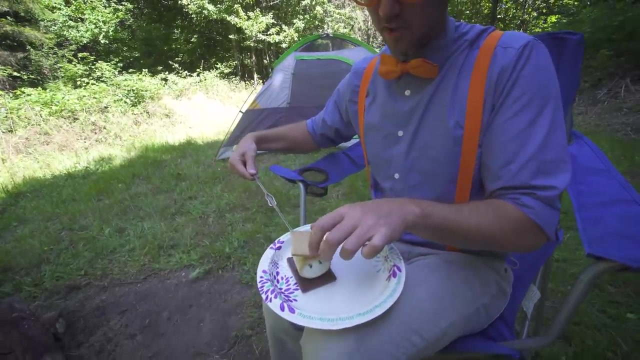 Whoa, That is looking so great. Do you see that? Whoa, Perfect, This is going to be so yummy. Alright, let's put it right on top of the chocolate, which the chocolate is on the gram, and then the mallow. 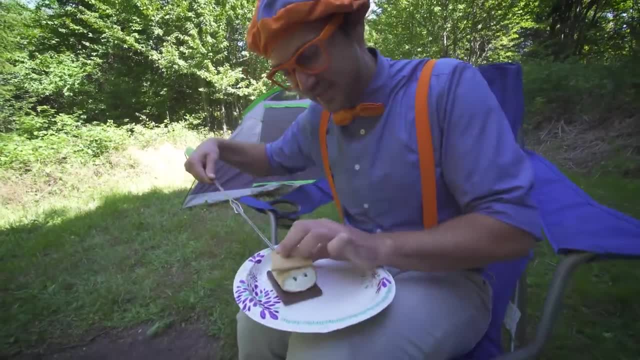 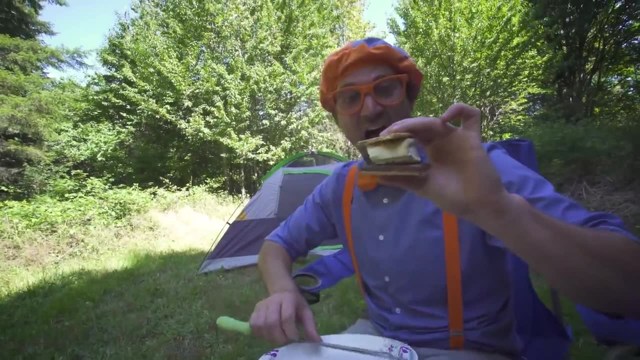 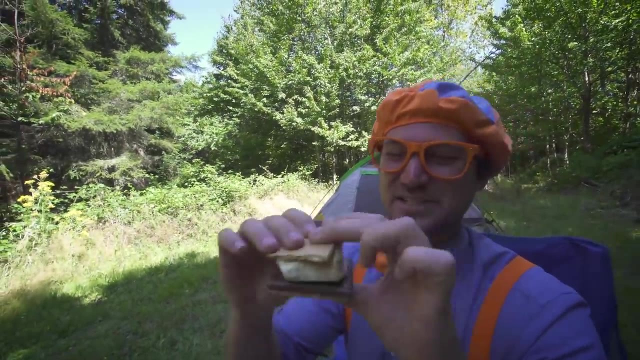 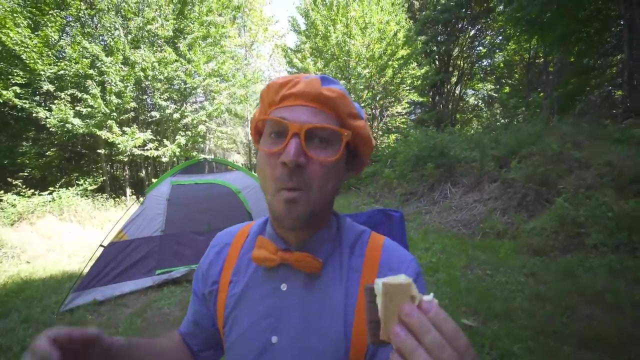 and then another gram, Slide it out, Whoa Perfect. Do you see that I call this yummy, yummy, yummy s'more dessert? Nom, nom, nom, Ready, Mmm, Mmm, Mmm, Yum. 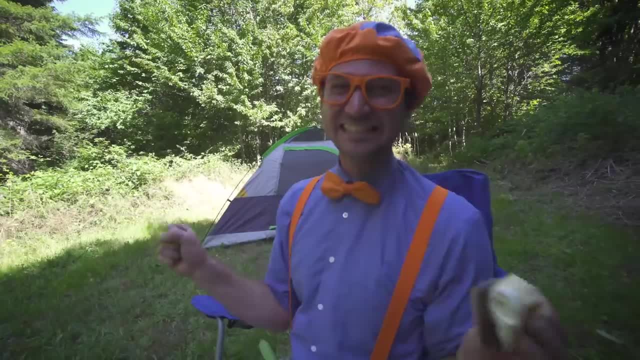 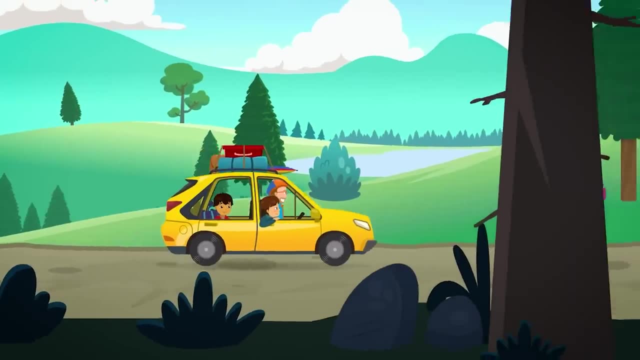 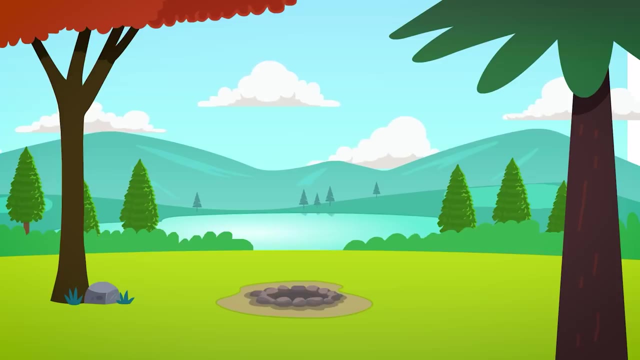 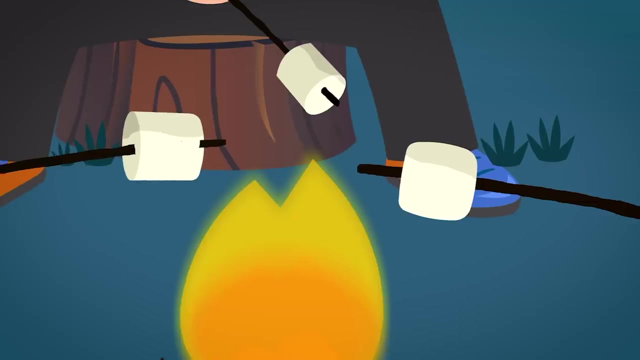 I think this is the perfect time for the camping song Here. it is the perfect place to pitch our tent, Beneath the stars in the mighty wilderness. We'll start a fire, make some s'mores and sing some songs. Hey, I know one: It's the camping song. 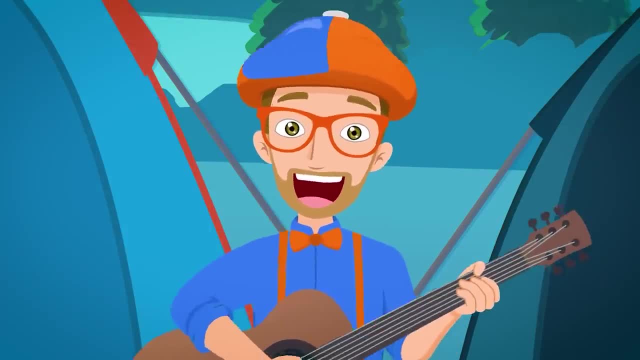 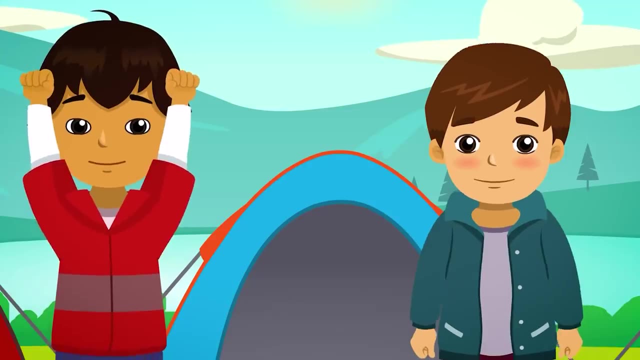 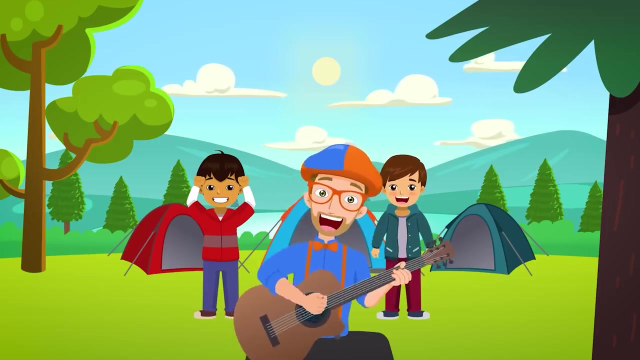 Let's go camping. It's so much fun. We'll learn so many things like how to fish and hunt. Let's go camping and get some sun. Let's go camping, cause it's so much fun. We'll go hiking and see all of nature's sights. 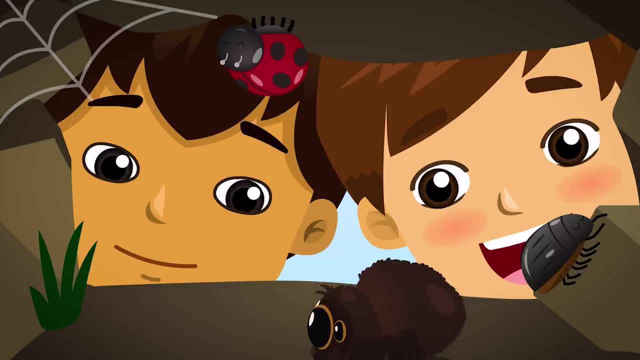 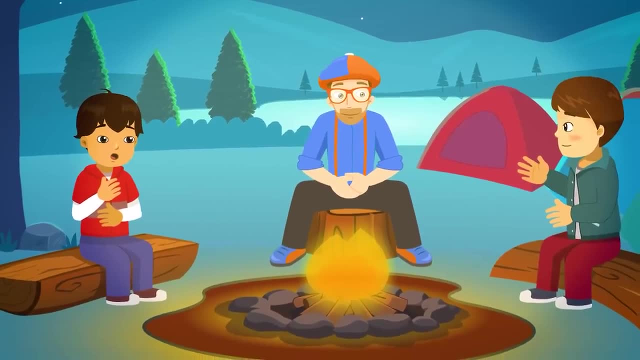 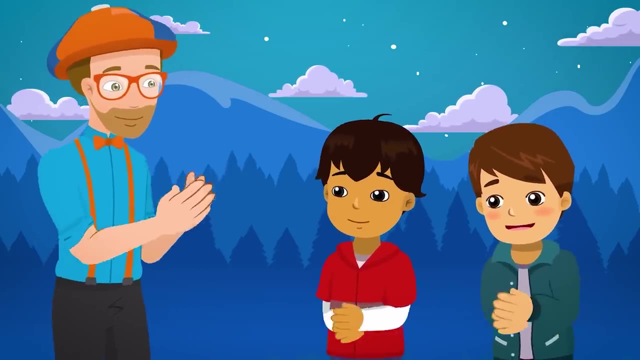 We'll see some animals and bugs of every kind, And we'll sit around the fire telling stories one by one. That's why camping is so much fun. Let's go camping. It's so much fun. We'll learn so many things like how to fish and hunt. 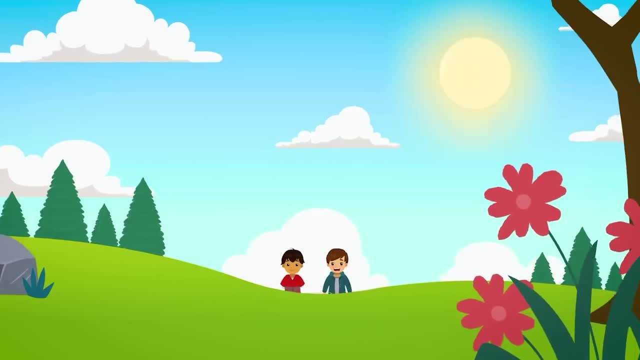 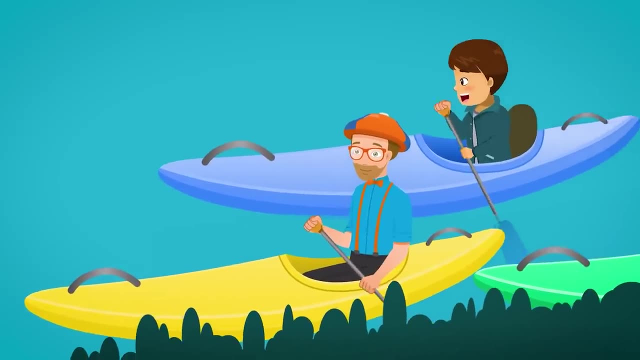 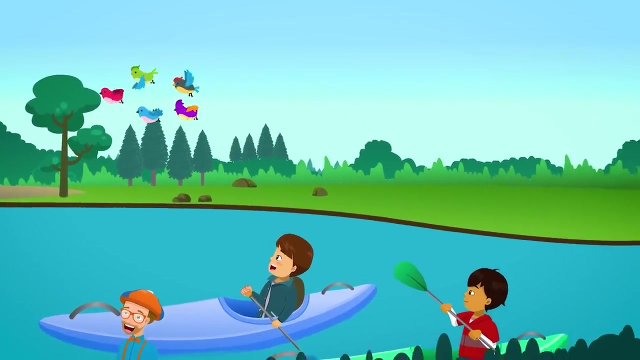 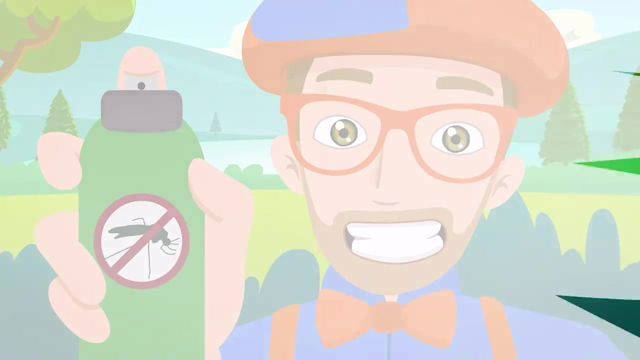 Let's go camping and get some sun. Let's go camping cause it's so much fun. We can go canoeing down the river stream, We can watch the birds fly above the trees- So much fun we can have throughout the day. But don't forget your mosquito spray. 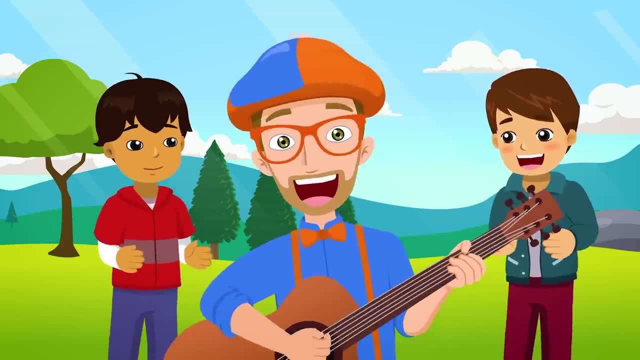 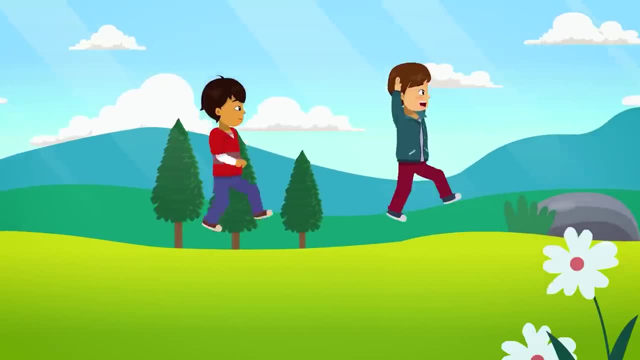 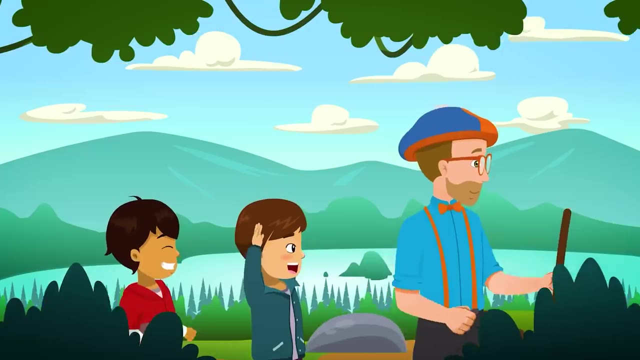 Let's go camping. It's so much fun. We'll learn so many things like how to fish and hunt. Let's go camping and get some sun. Let's go camping cause it's so much fun. Let's go camping, It's so much fun. 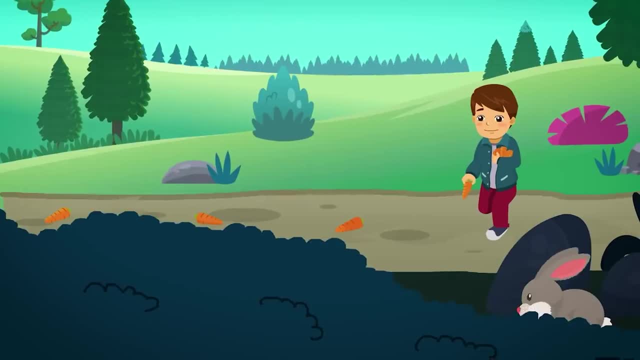 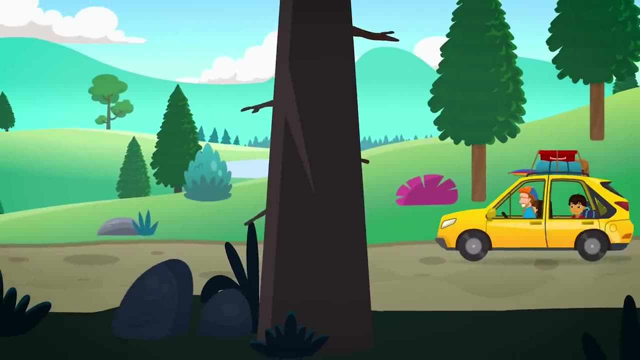 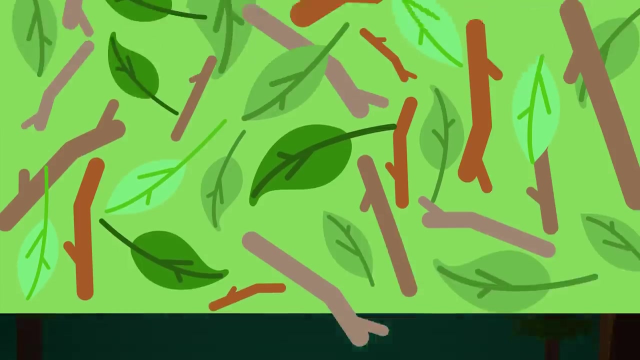 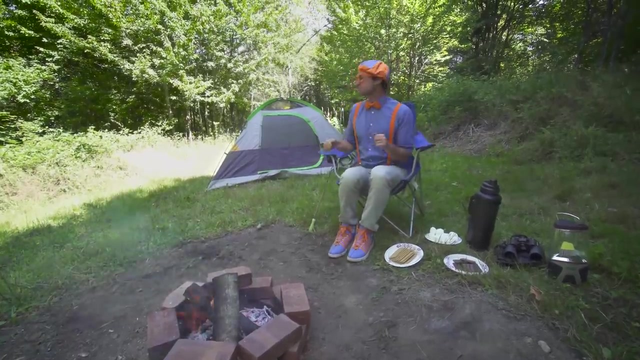 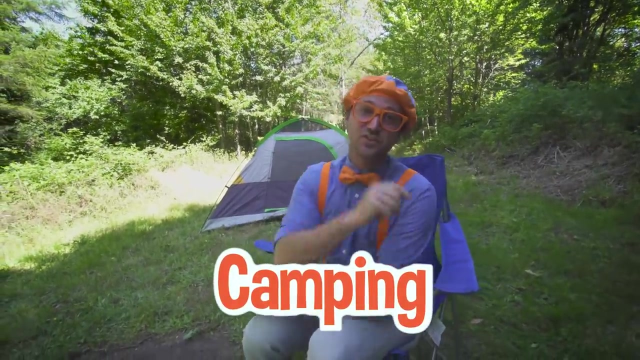 We'll learn so many things like how to fish and hunt. Let's go camping and get some sun. Let's go camping cause it's so much fun. S'mores are so yummy And camping is so much fun. Did you have a good day with me today? 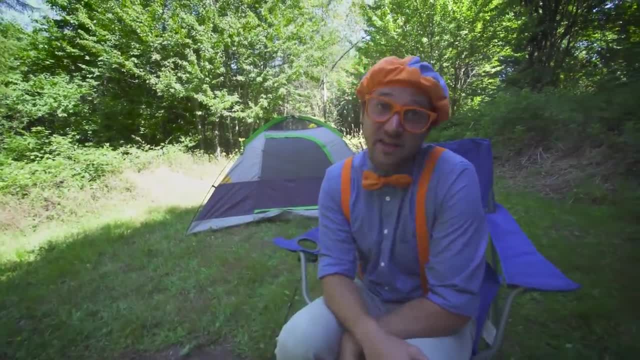 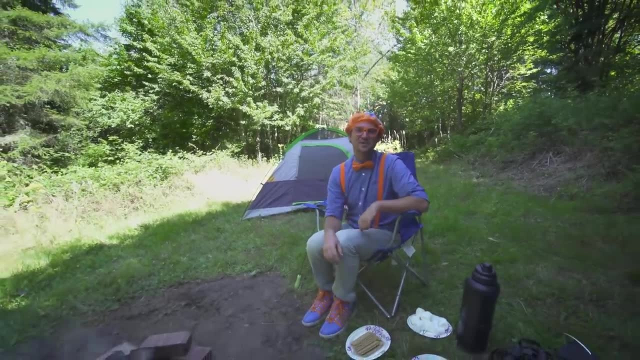 Yeah, Well, this is the end of this video, But if you want to watch more of my videos, All you have to do is search for my name. Will you spell my name with me? B-L-I-P-P-I, Blippi, Good job. 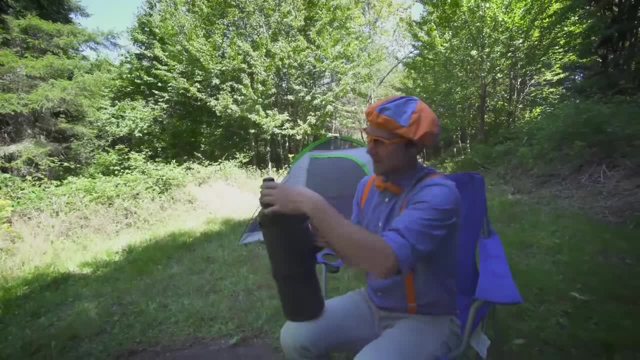 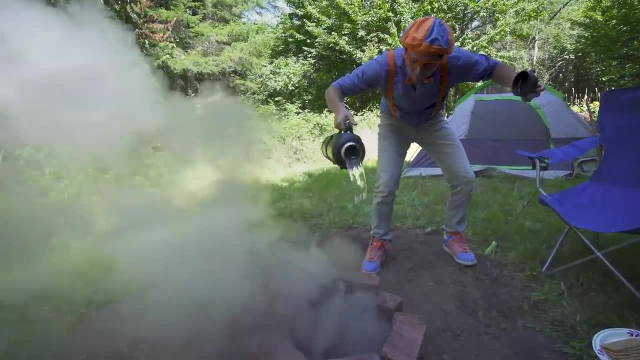 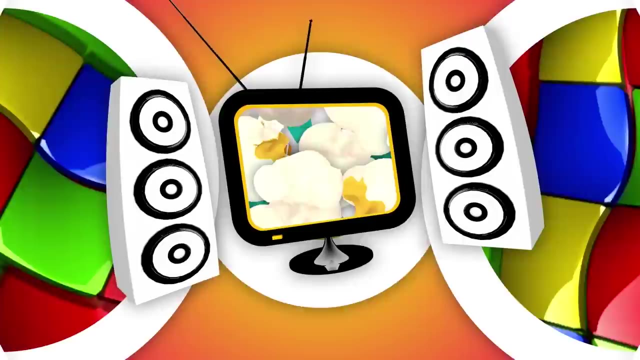 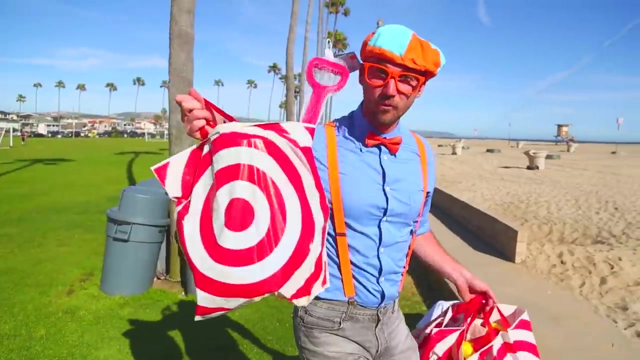 Alright, I should probably put out the fire right now. Yeah, here we go. So much to learn about. It'll make you want to shout Blippi. Hey, Look at what I have. Ooh, I have some bags of sand toys. 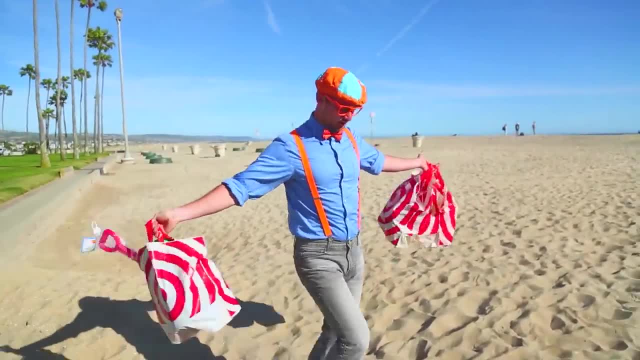 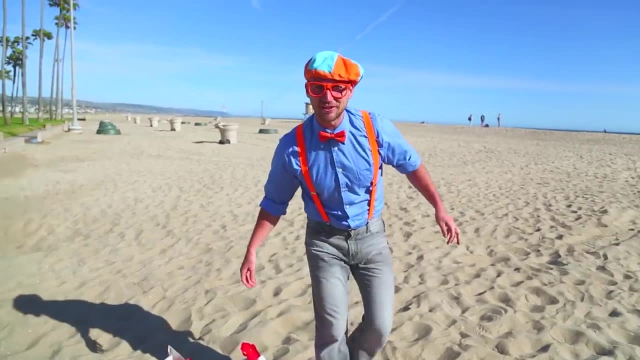 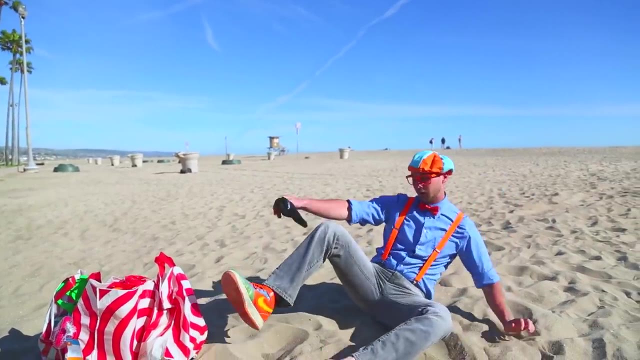 And today we are going to play in the sand. Whoa, Whoa. Okay, first things. first, Let's take off our shoes. The reason why I'm taking off my shoes, Whoa, Is because Sam feels so good on my feet. 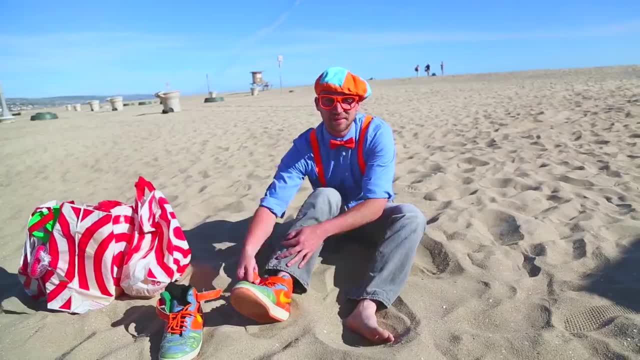 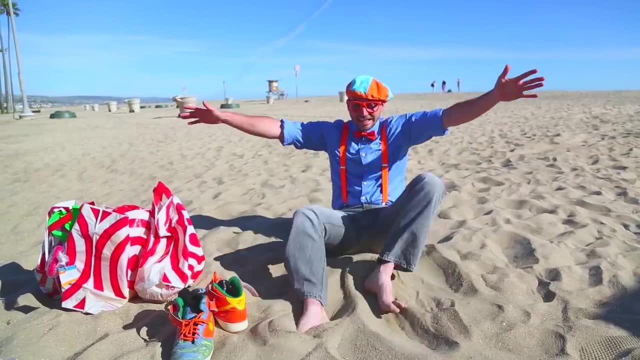 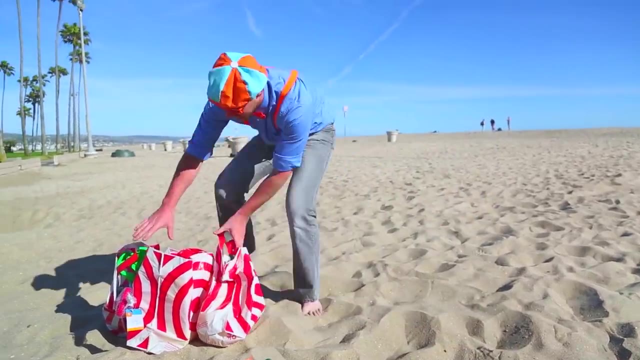 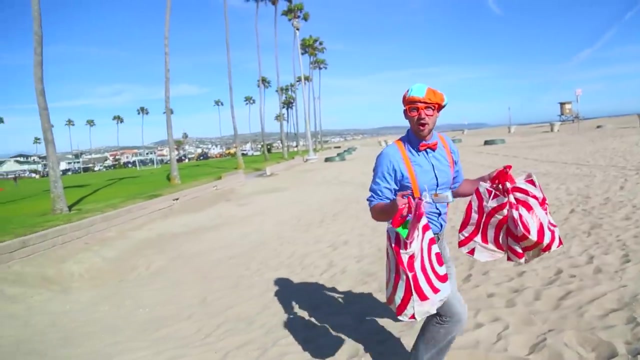 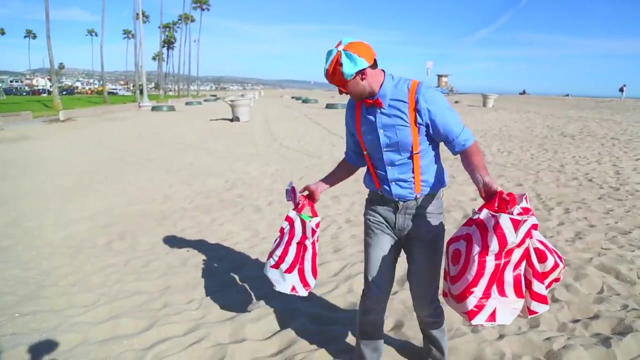 Whoa. Okay, now my other shoe. Yes, Okay, I'll leave my shoes right here And let me grab the bags And let's go out in the sand. I am so excited to show you all the sand toys that I have. Does this look like a good spot? 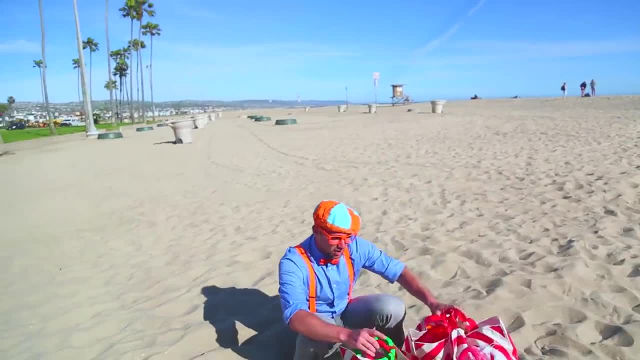 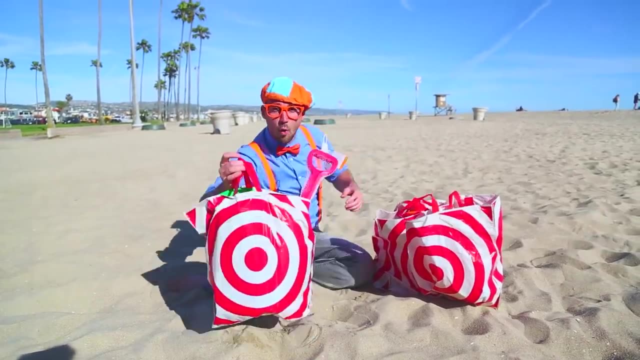 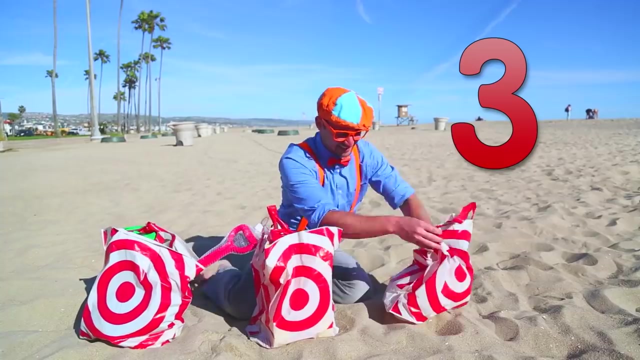 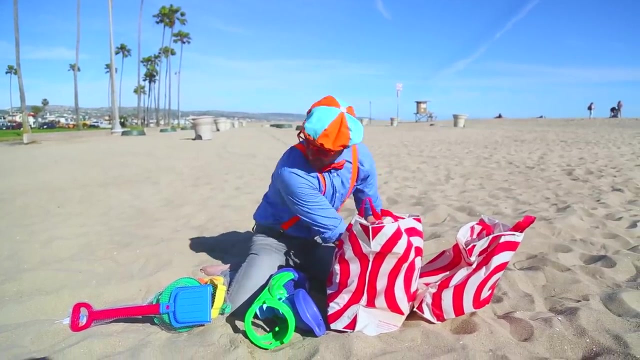 I think so. Okay, look Like I said, I feel so good on my feet. Okay, I have one bag, Two bags And three bags. Okay, let's see what we have in here. Okay, the first bag has A green and blue toy. 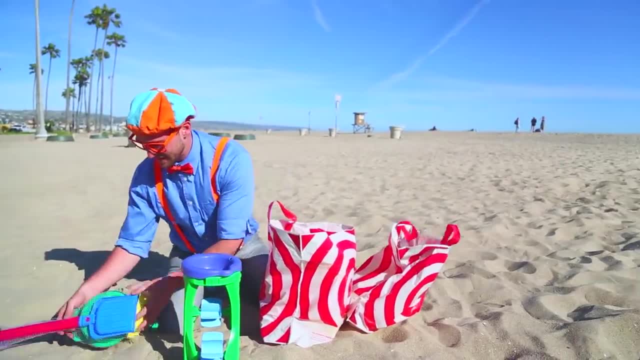 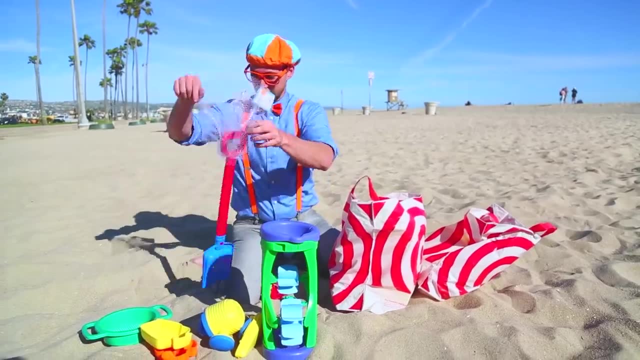 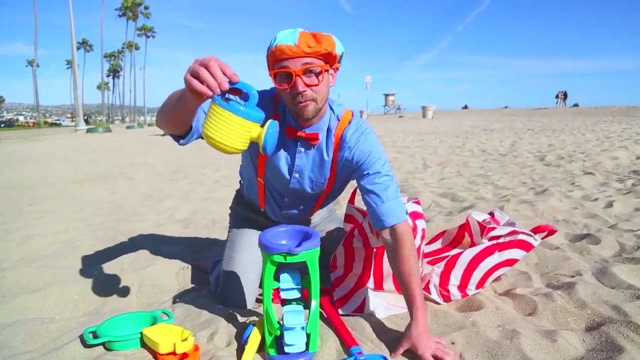 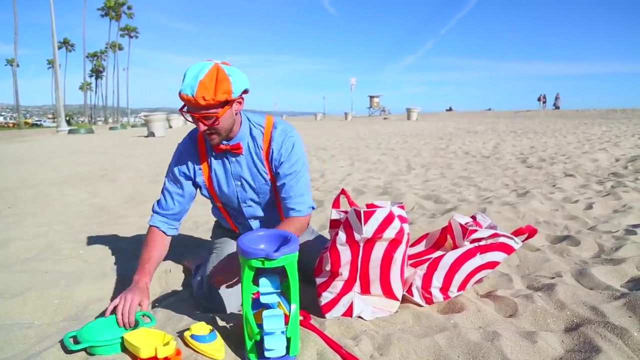 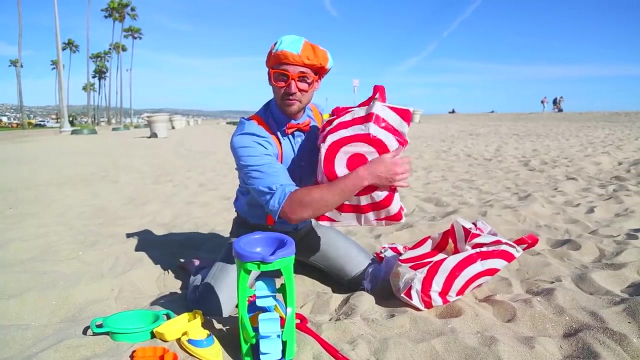 We'll play with that in just a little bit. And then, Whoa, This has so many other toys in it, Like the shovel And That toy, Ooh, a little boat And some other cool looking toys. Okay, alright, Let's see what bag number two has. 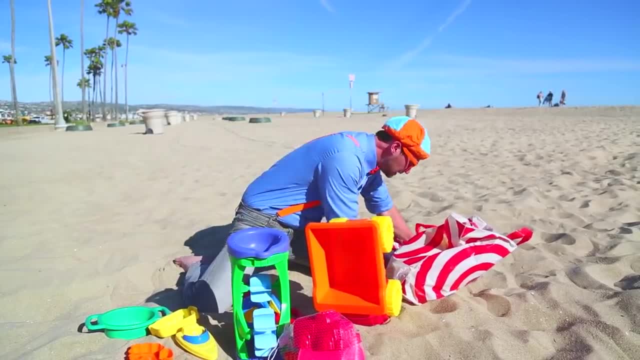 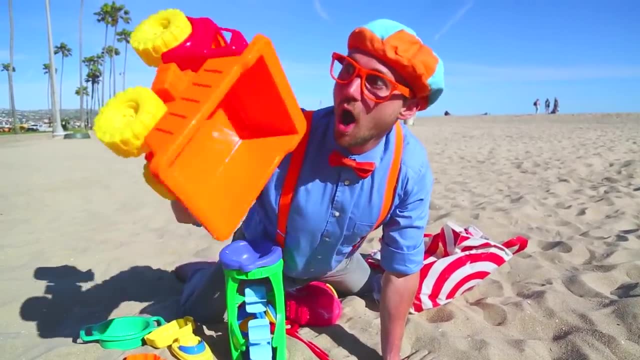 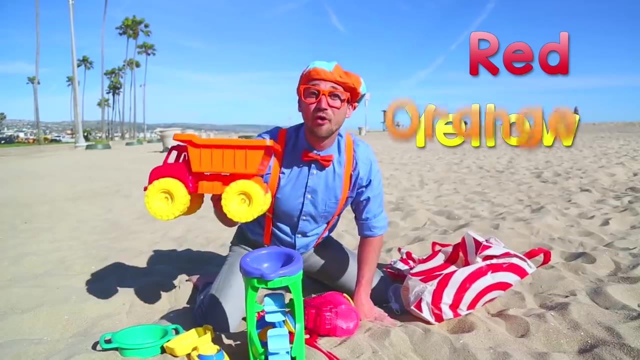 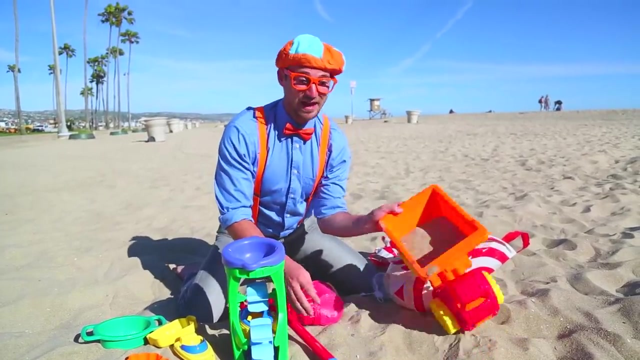 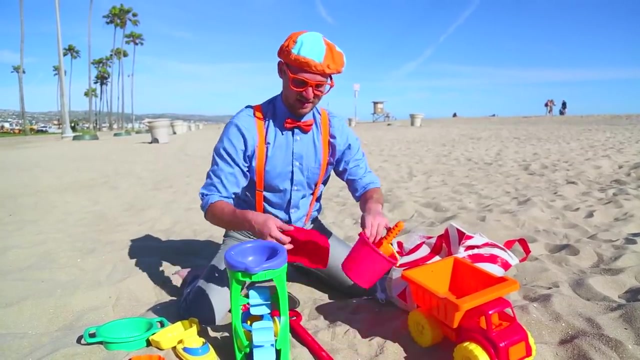 Whoa. Bag number two has A giant dump truck. Whoa, This dump truck is the color red, Yellow And orange. Okay, We're gonna put a bunch of sand In this later, Just like that, But a lot more of it, Okay, And A lot of other toys. 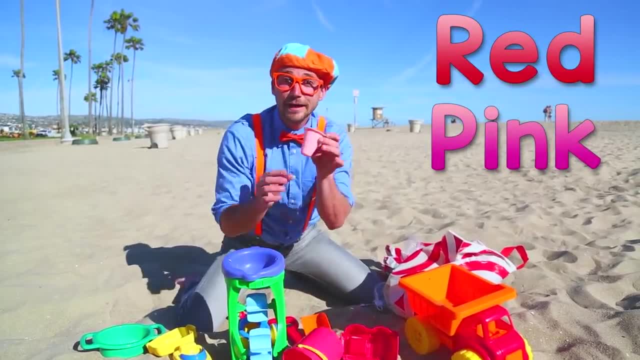 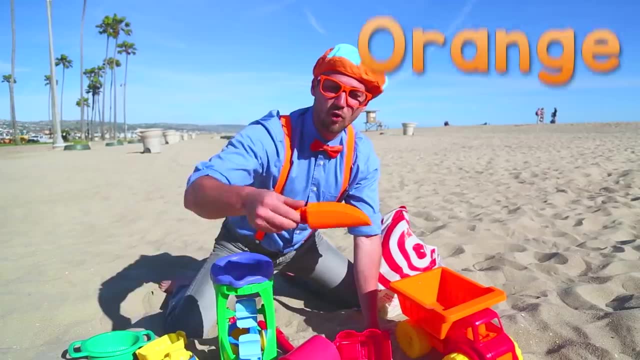 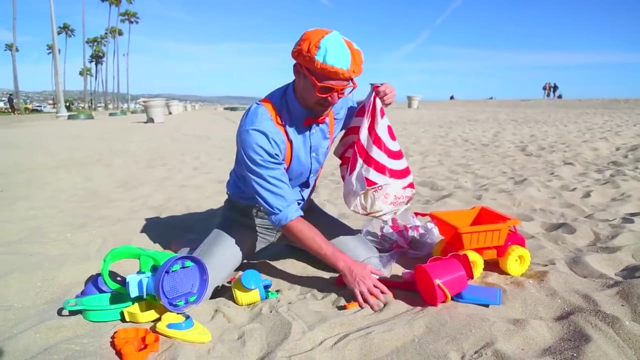 A red one And A pink one, An itty bitty one- Look Woo, That's funny. And a scooper. Look at this orange scooper. Okay, And the last bag has. I'm so excited to see what's in this bag. 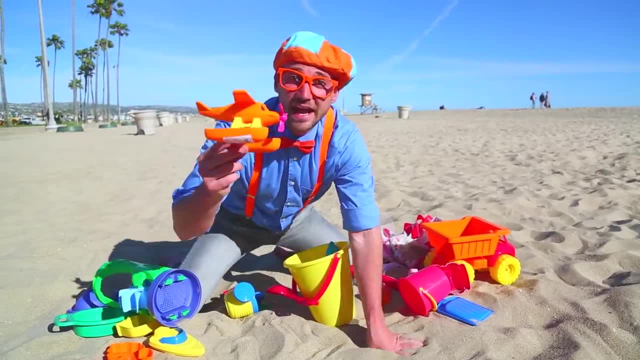 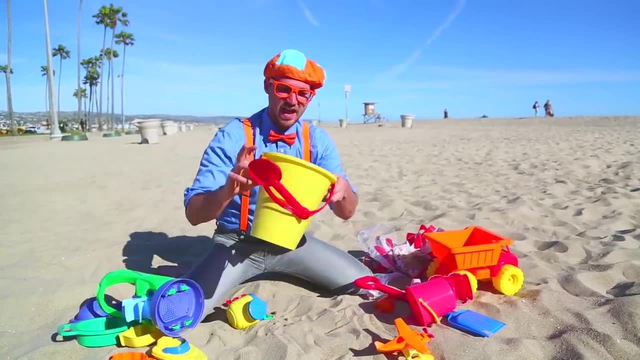 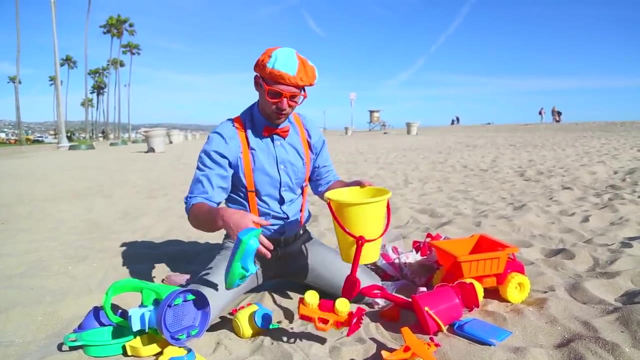 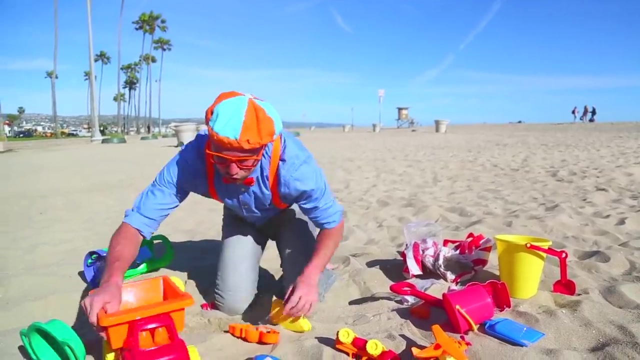 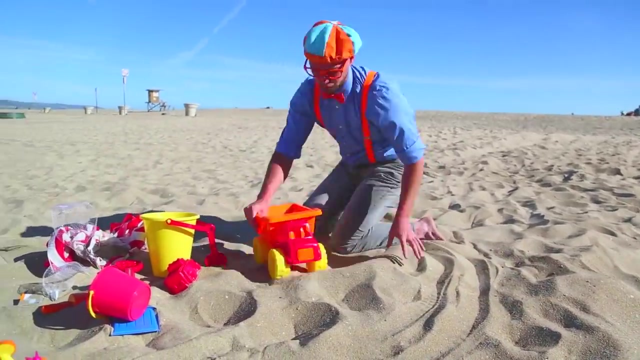 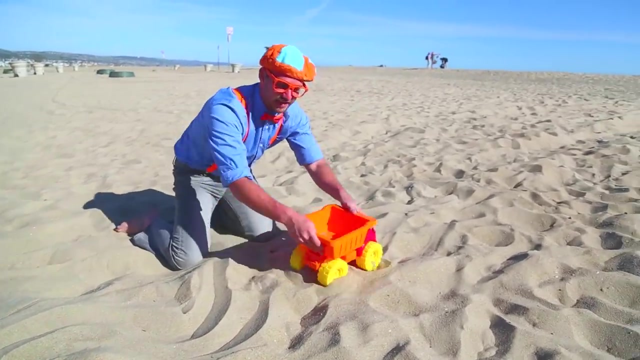 This bag has Whoa, An airplane, Whoa Oh, And A yellow bucket With a red scooper And some other toys. Okay, Okay, I think we should take the dump truck. Come over here, Come on, Okay, Let's put the dump truck right here. 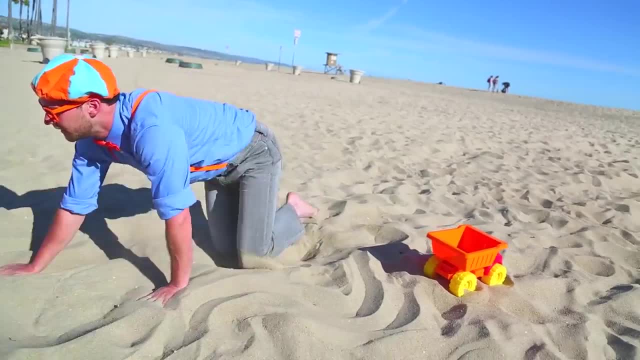 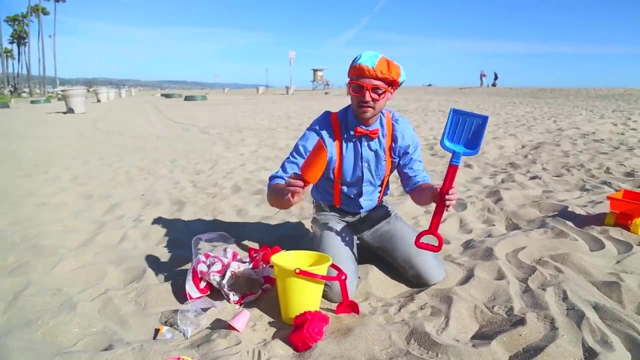 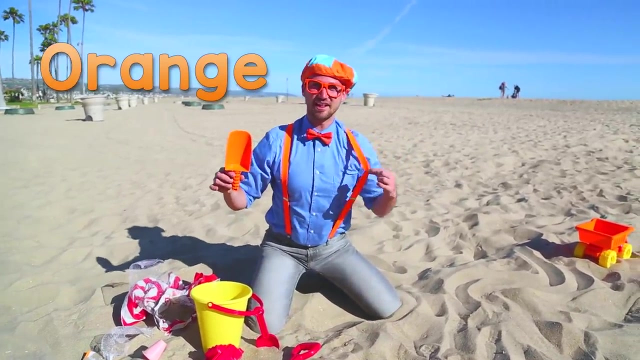 Okay, And I need a scooper. Come on Okay. Should we use this big shovel Or This orange hand shovel? Um, Let's use this orange one, Because it's the color of my suspenders And bow tie. Come on Oh. 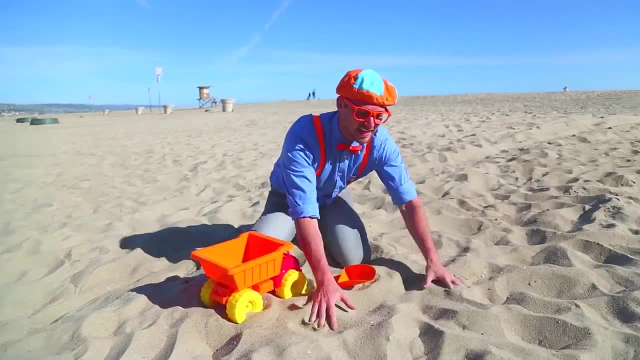 This sand feels so good in my hands. Get a close up. look at this. Whoa, Whoa, My hands and my feet Feels so good, Wow, Okay. Now let's Get a big scoop in the back of the dump truck. 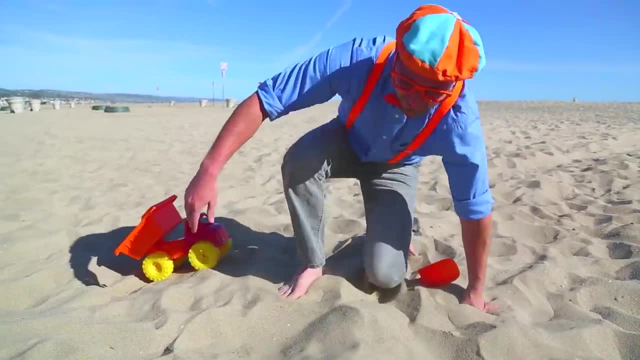 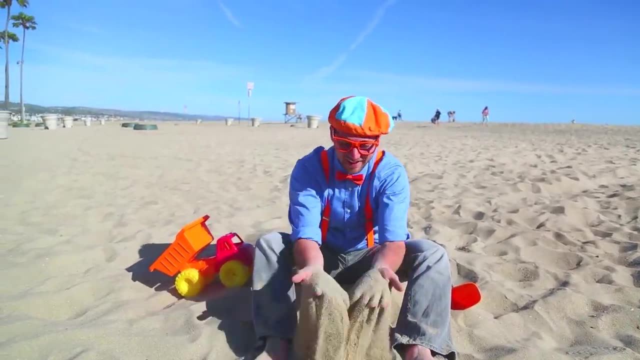 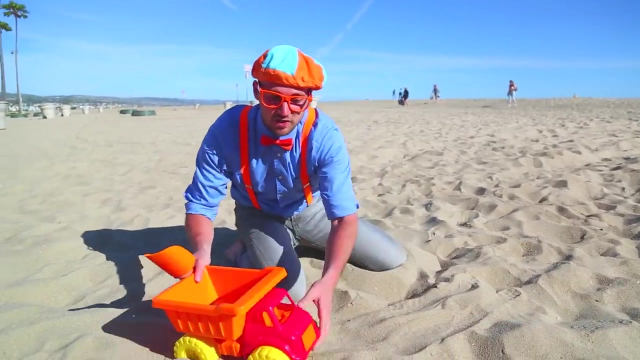 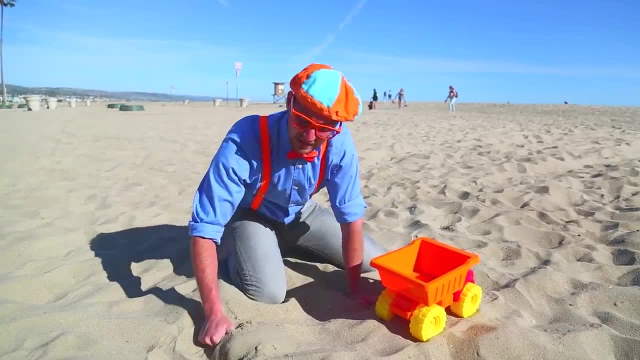 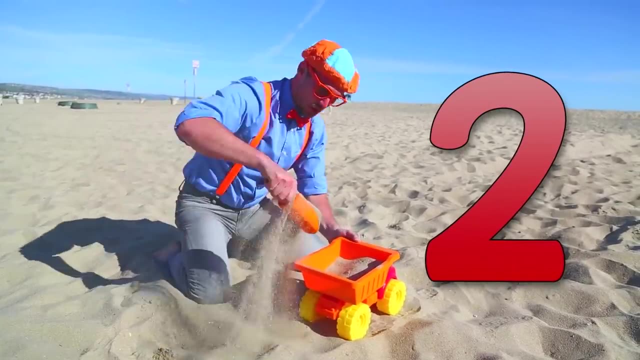 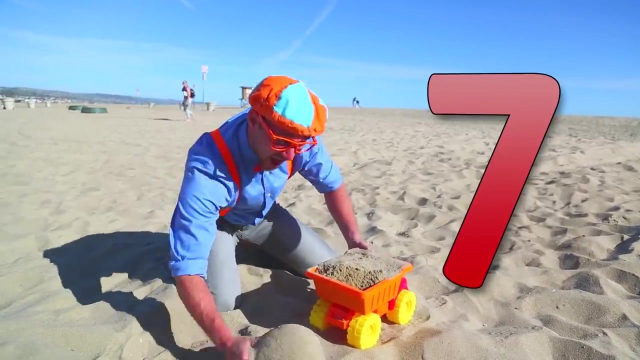 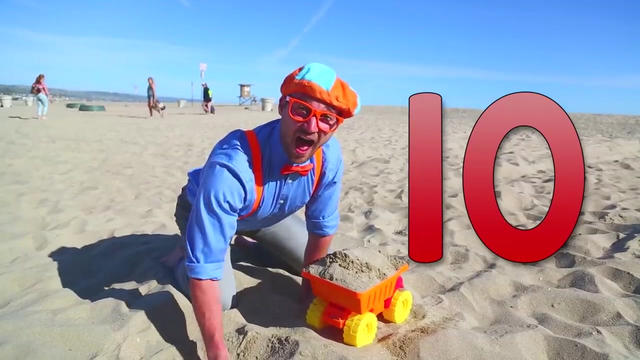 Vroom, Vroom, Vroom, Vroom, Vroom, Vroom. Okay, Let's count them together. Get it all empty: One, Two, Three, Four, Five, Six, Seven, Eight, Nine, Ten, One more Eleven. Oh Yeah, Look at that. 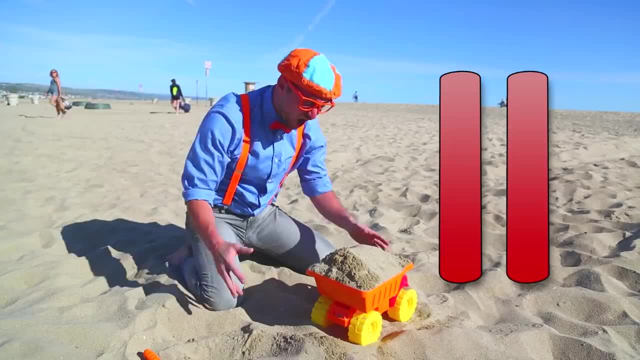 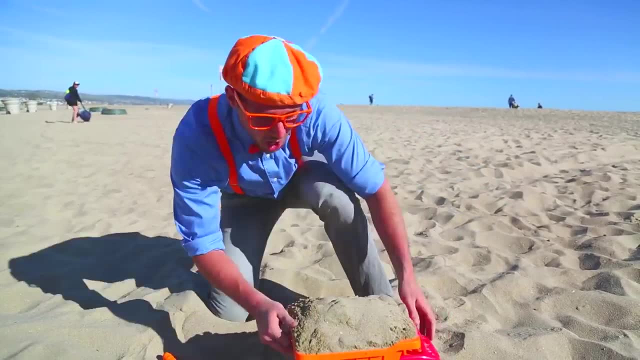 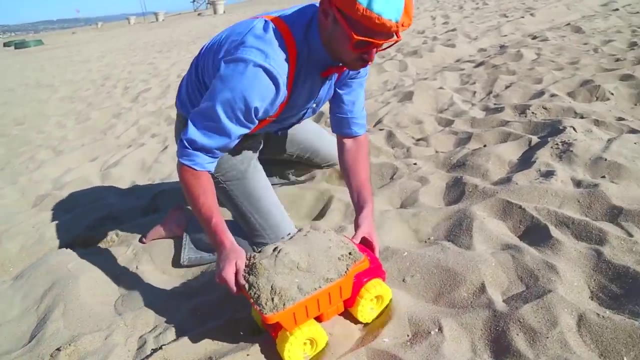 So fancy. Oh my gosh, I'm gonna go get started. So excited, I'm so excited, So heavy. wow, look at this giant. Oh, okay, Let's dump it out together. ready, come this way. Oh, how about right here? 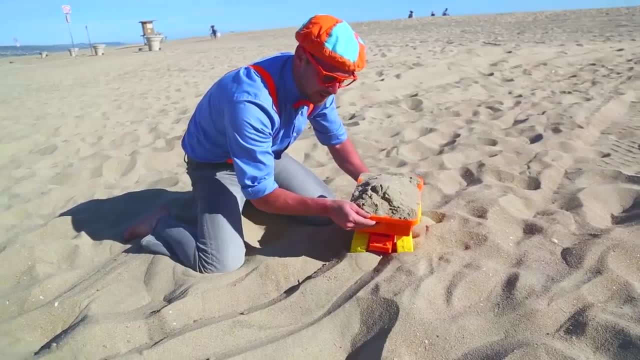 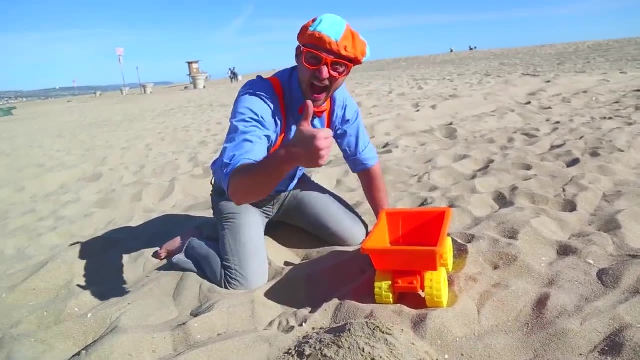 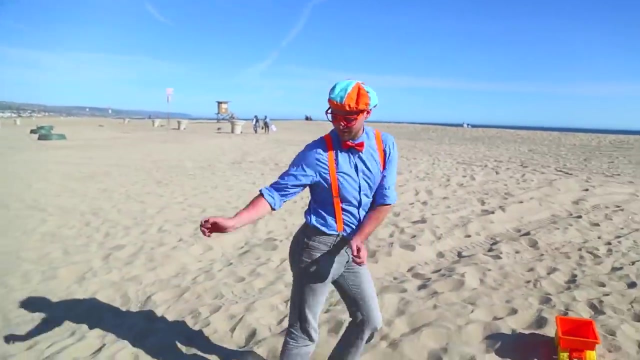 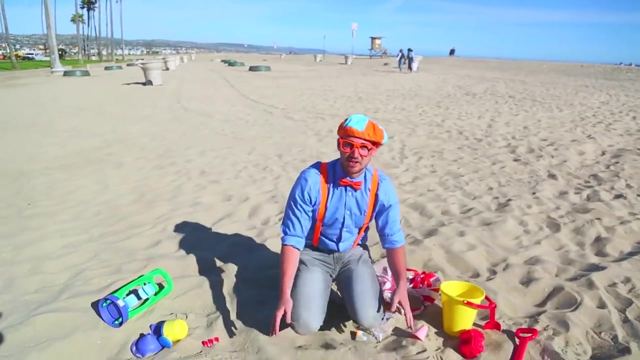 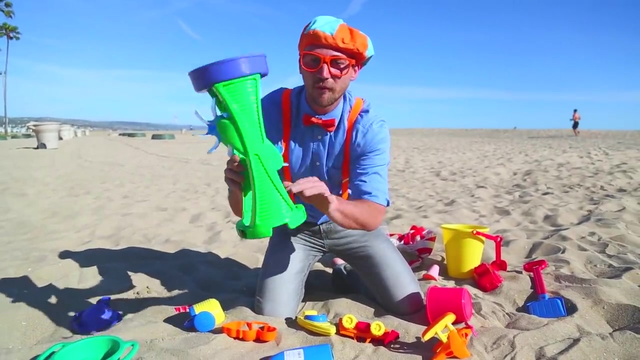 Okay, right here, ready. beep, beep, beep, beep, beep, beep, beep. Oh yeah, that was awesome. Let's go get some more toys come this way. Okay, look at all the toys. Let's see what other toys- whoa, Look at this toy. Whoa, like I said earlier, this toy is the color blue and green. 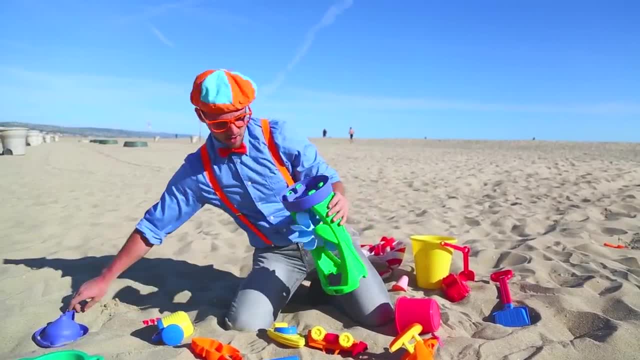 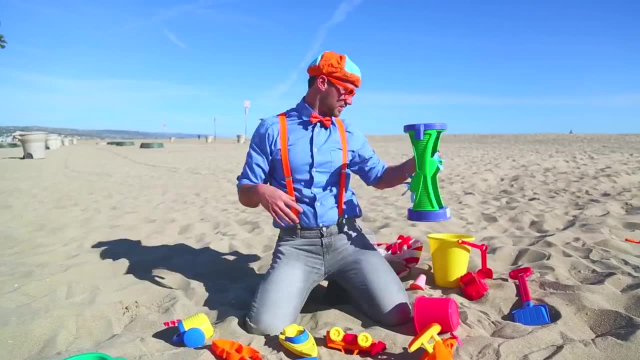 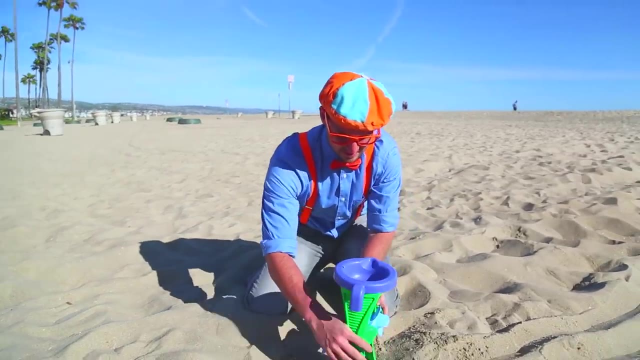 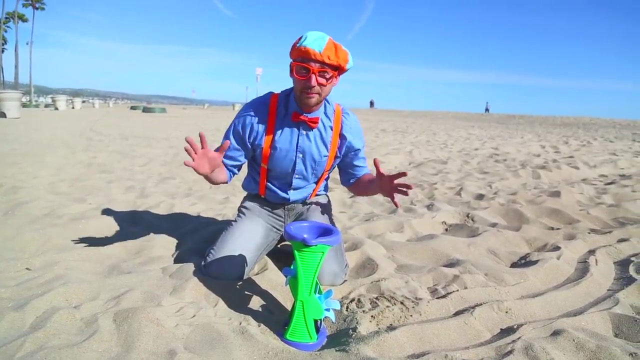 green. Okay, Let's see. Oh look, I think this goes on top. and then we put sand on top. come on, Let's put it right, Right, where this scooper was. Okay, You might have to get a close-up shot of this later, but let me grab that really big shovel from earlier. right, the shovel. 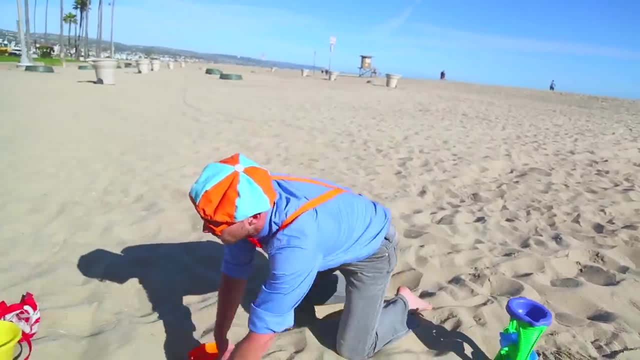 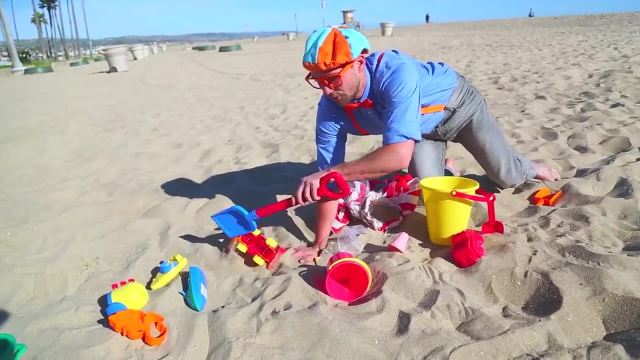 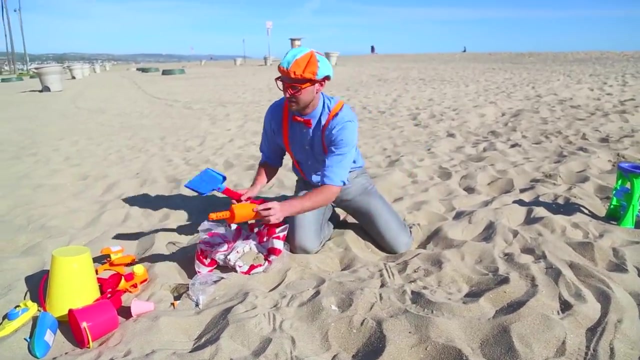 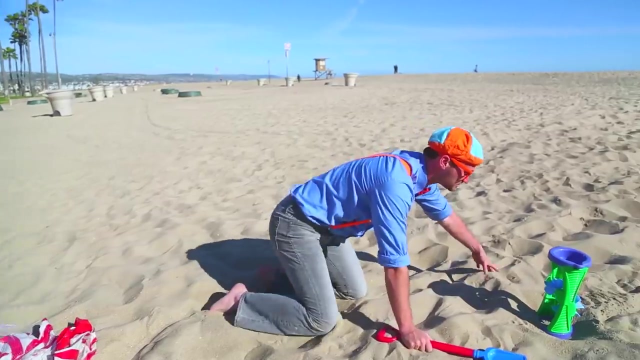 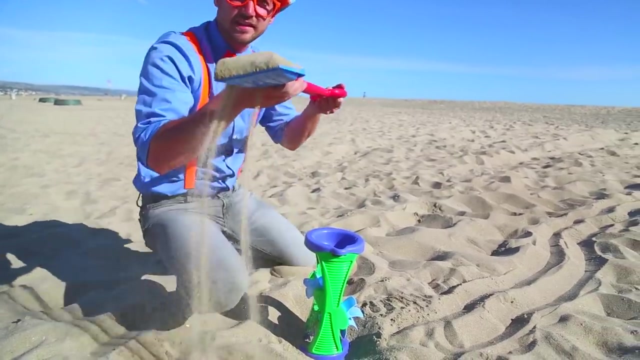 Yeah, okay, Come over here. Oh, Oh, Okay, You go over here. Move around here. toys, The shovels make it way. These are the bags from earlier. okay, Consolidation. Okay, great, now I have the shovel. Okay, let's shovel some sand. look at this. 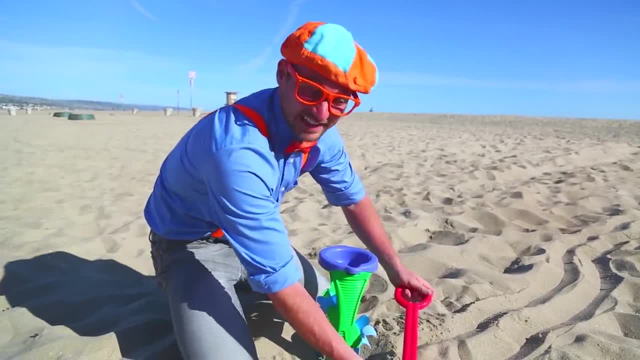 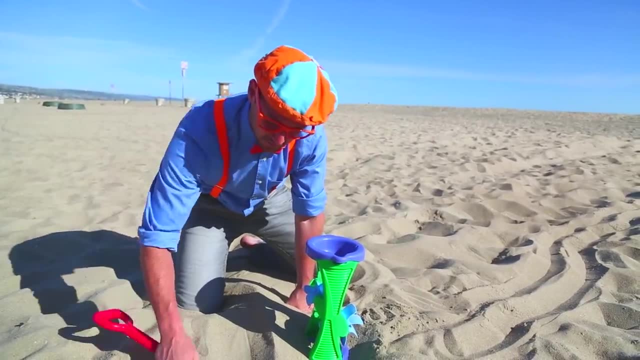 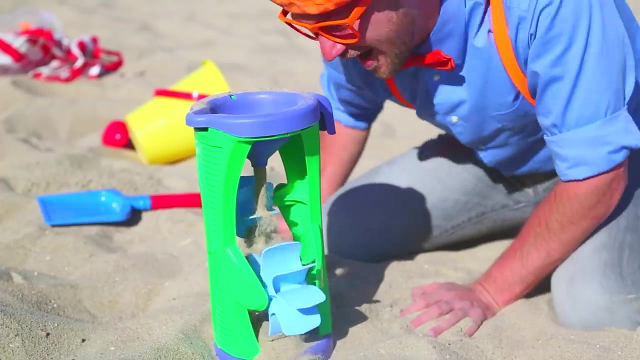 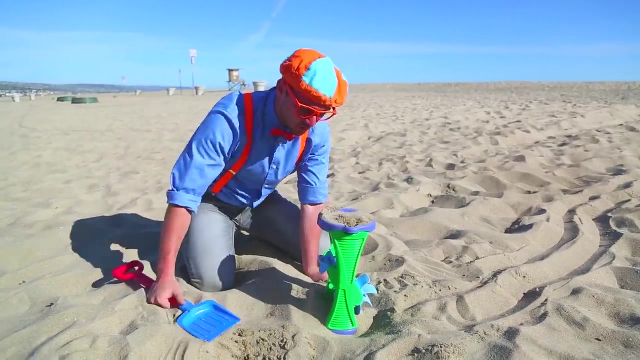 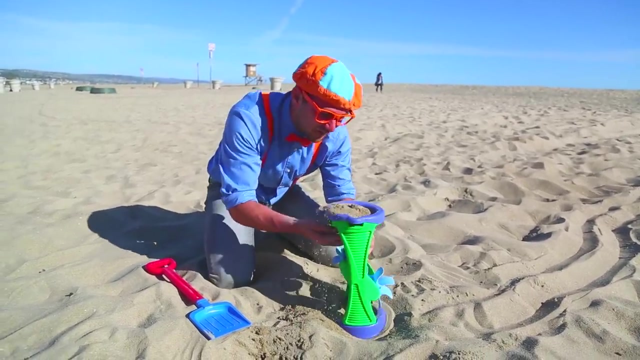 Wow, Wow, you want to see that again? Whoa, Okay, let's put some in here and then you can get a close-up shot ready. Whoa, Wow, did you see that one more time? Oh, Shake, shake, shake. Oh, come on, You can go. 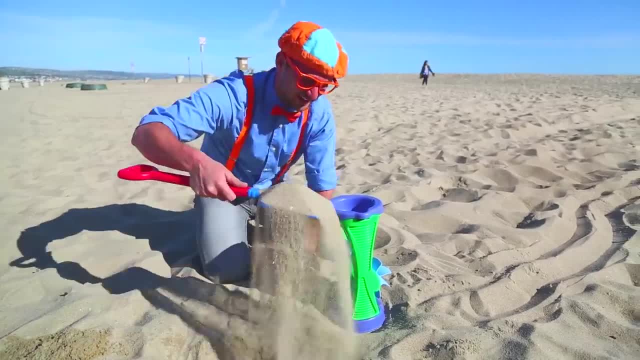 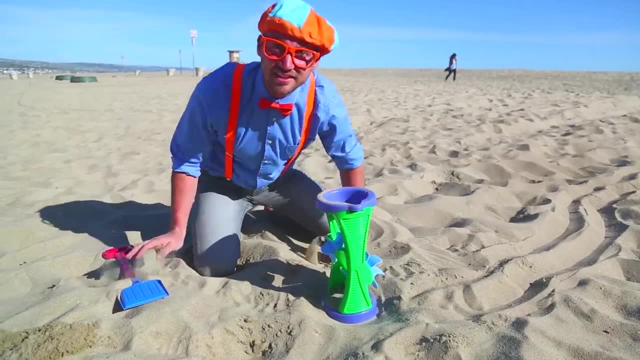 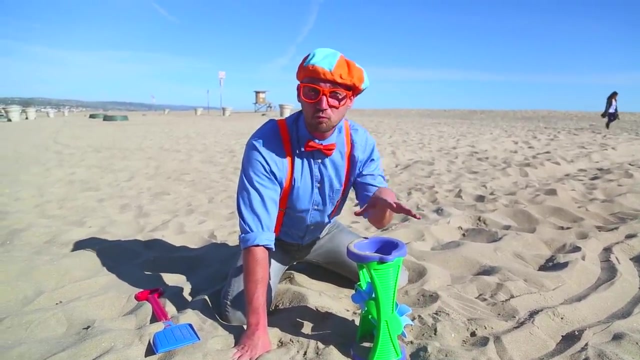 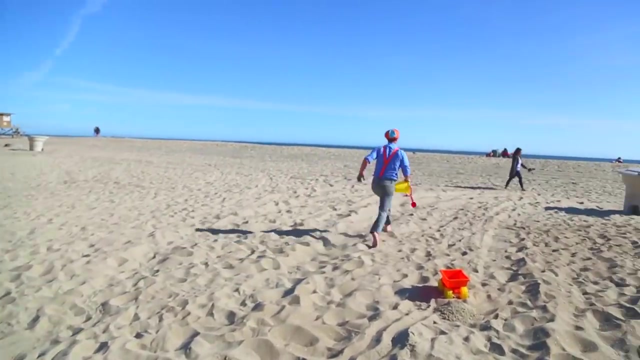 We might need drier sand. okay, here we go. Whoa, Did you see how fast that spun? now Let me go grab a bucket and go fill it up with water, and we'll try this again with water watch, Oh Look, we made it to the water. 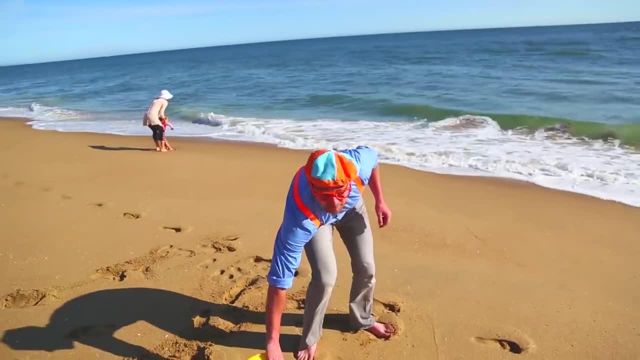 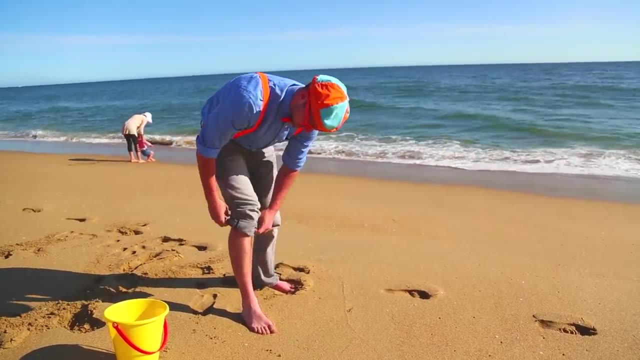 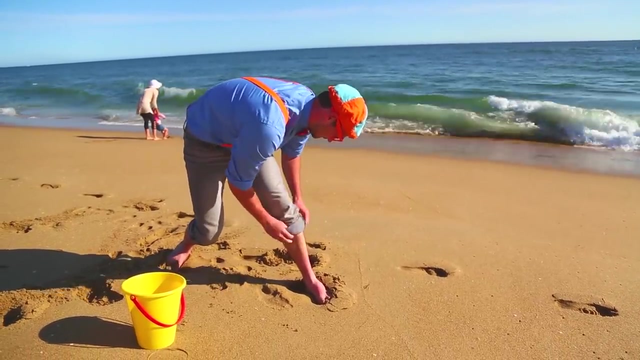 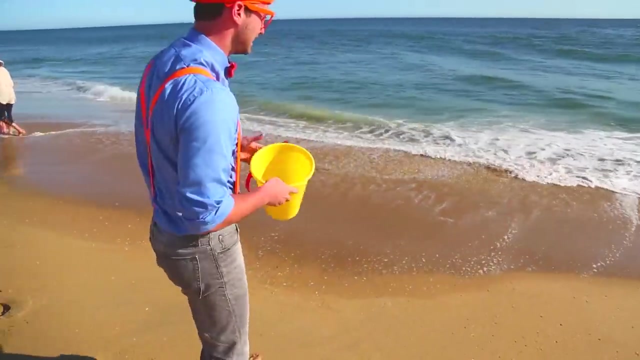 But I don't have my bathing suit on, so I'm gonna roll up my pants so they don't get wet. Just do a couple rolls up, just like this. Hey, This one as well. Okay, I'm ready to get us some water. Whoa, Get ready for a wave and I'll scoop up some water. 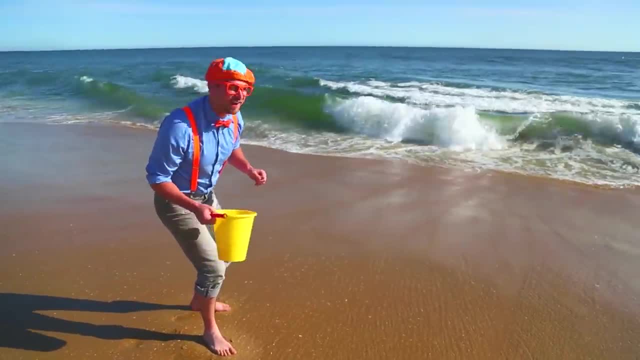 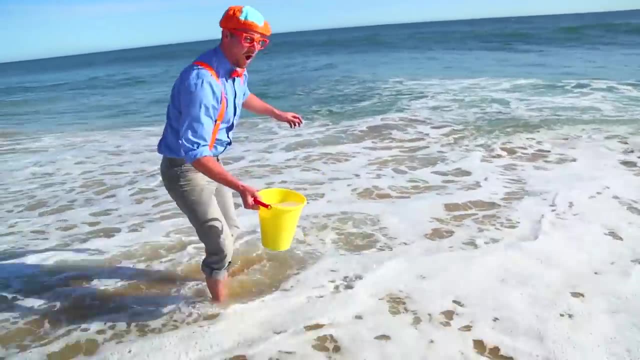 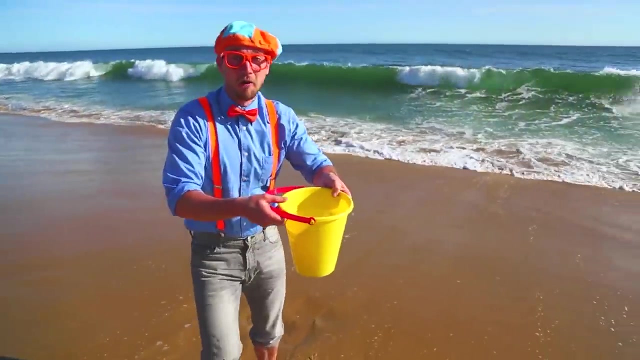 Whoa, Here comes the big one. I got some water. Look Whoa See Whee, I can't waste it. We gotta go put it in the toy, Come on. I got some water. Look Whoa See Whee, I can't waste it. We gotta go put it in the toy, Come on. 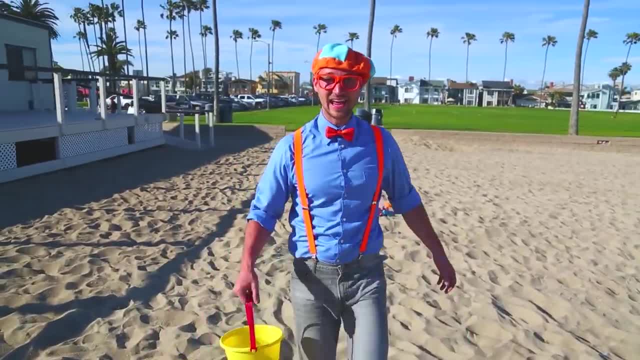 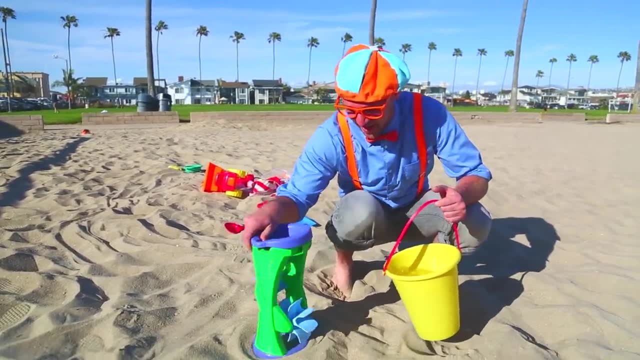 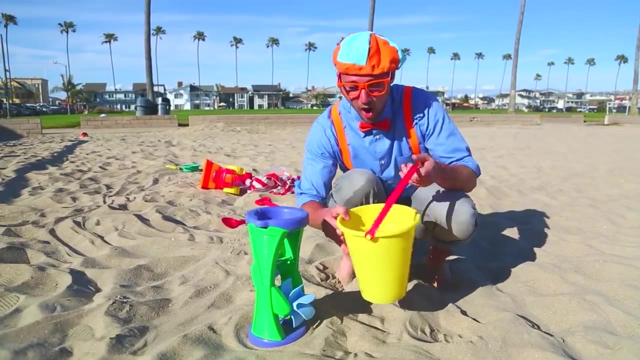 Okay, now that we have a full bucket of water, I kind of want to see what it's like pouring water in here. Okay, you know how these spin when we put sand in it. Yeah, let's see if we pour water that we got from the ocean in here, if they spin. 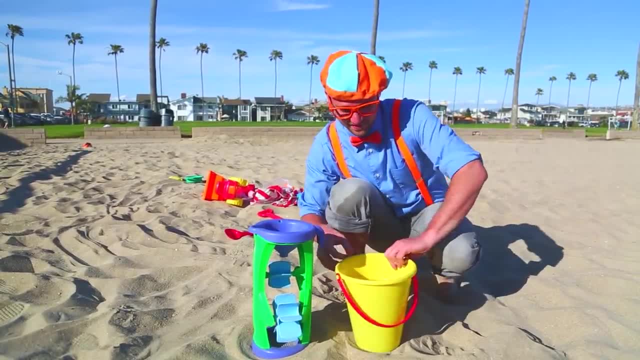 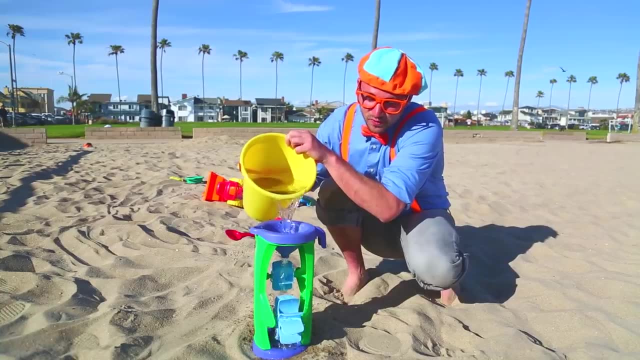 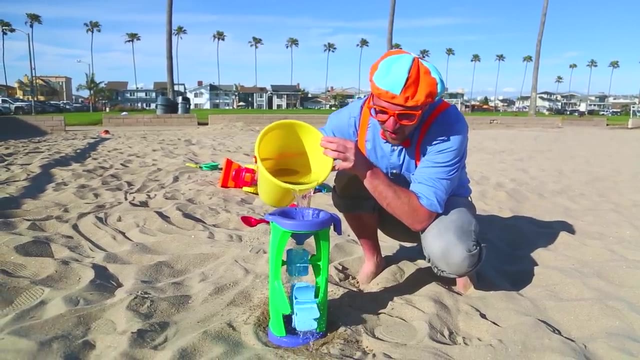 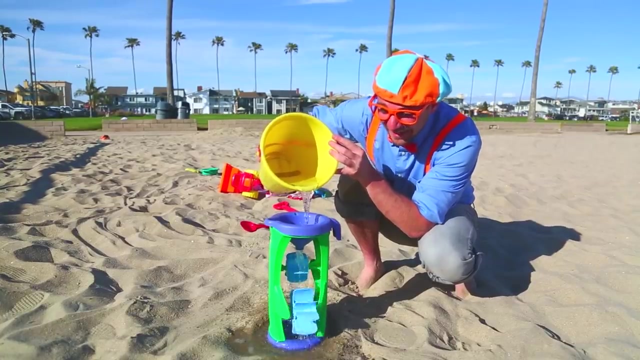 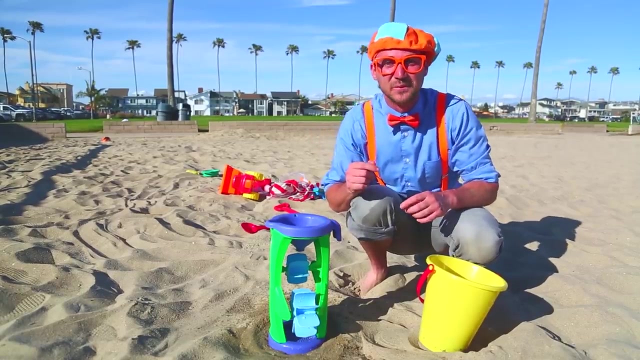 How does that look? Can you see them? Yeah, okay, Here we go. Whoa, it's working. Oh, okay, Let's fix this one. Okay, Ready, Okay, here we go. Yeah, Yeah, it's working. That was so much fun playing with these sand toys with you. 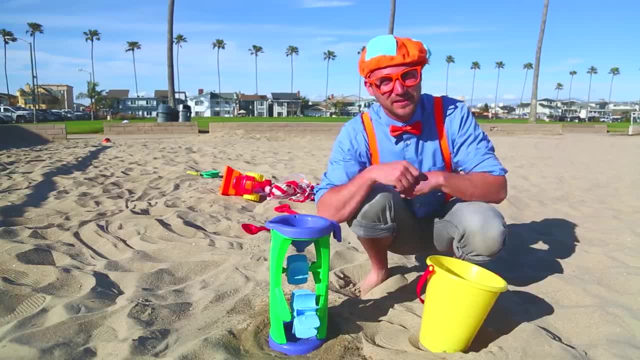 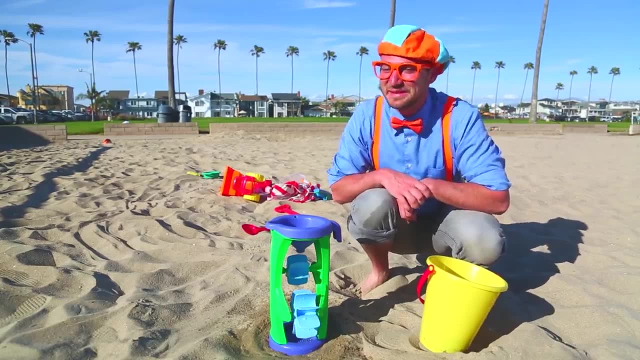 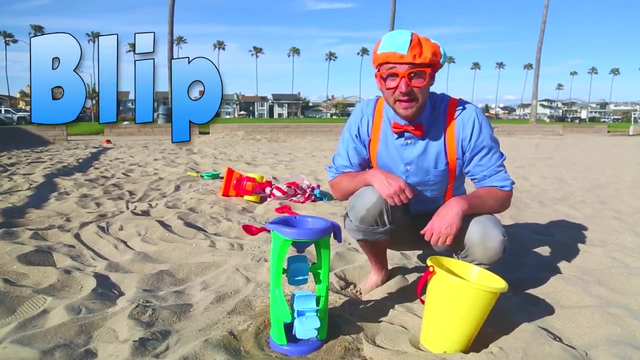 Well, if you want to watch more of my videos, you know what to do. Yep, Just search for my name. Do you know how to spell my name? Yeah, let's spell it together: Ready, B-L-I, P-P-I, Blippi. Yeah, That's my name. Good job, and see you again. Bye-bye. 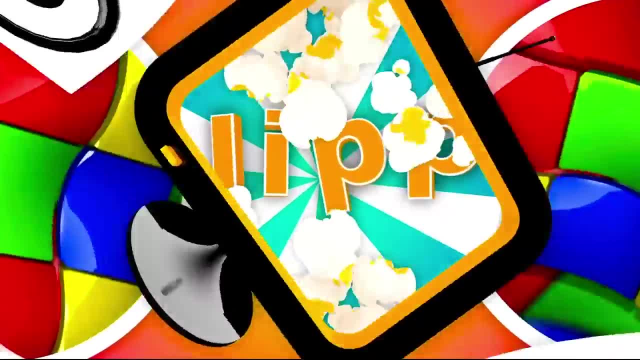 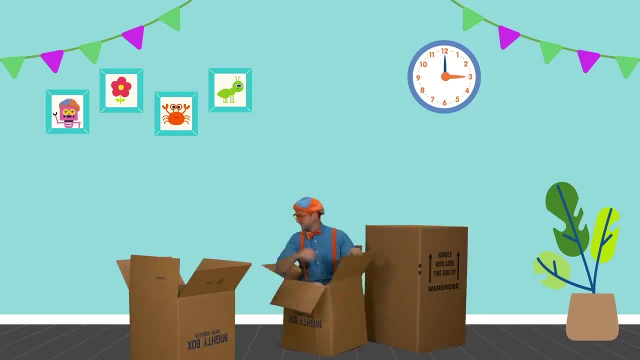 So much to learn about. it'll make you want to shout: Blippi, Blippi, Aw, Ha, ha, Ha, ha. Hey, It's me, Blippi, and I was just hanging out in this cardboard box. Check it out. 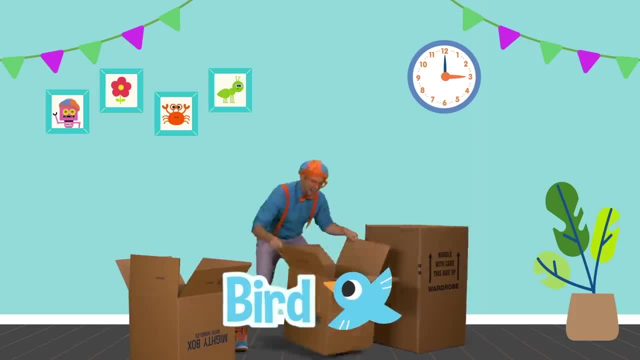 It's like a bird, Whee. Oh, I have so many cardboard boxes around here. What are we to do with them? Hmm, I have an idea. Why don't we take a few of these cardboard boxes and make something out of them? 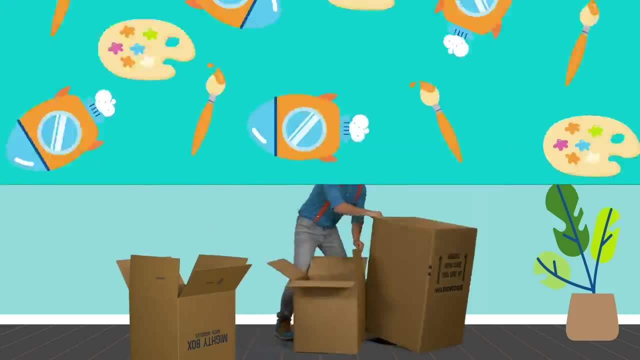 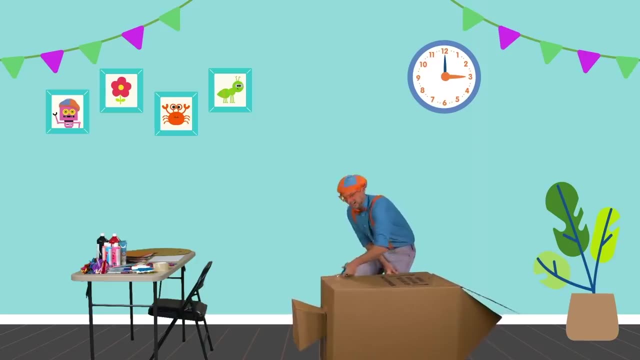 This is gonna be fun. Blippi, Blippi. Oh Hey, How are you doing? I'm just making a rocket ship out of these cardboard boxes. I am using these scissors, nice and safely, to cut a giant window out of it. 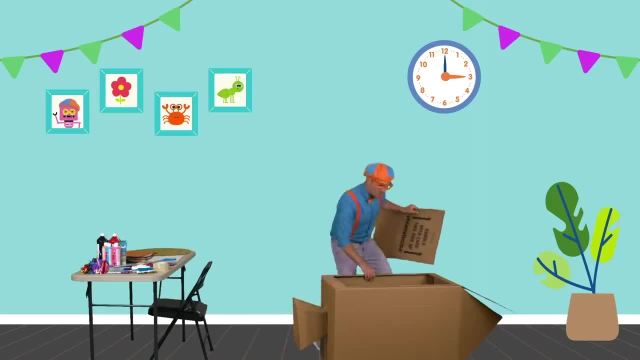 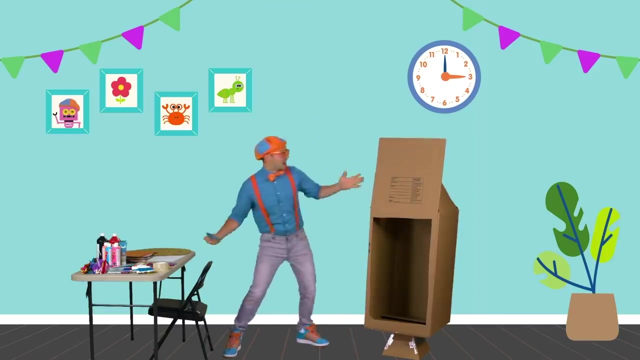 Whoa, Look at that. Wow, Ooh, Now I can sit inside it later. Hmm, Then we can explore outer space. I am so excited. Okay, Here we go. So now that I have my window, I can then put the cardboard box- well, it used to be a box, now it's a rocket ship- up. 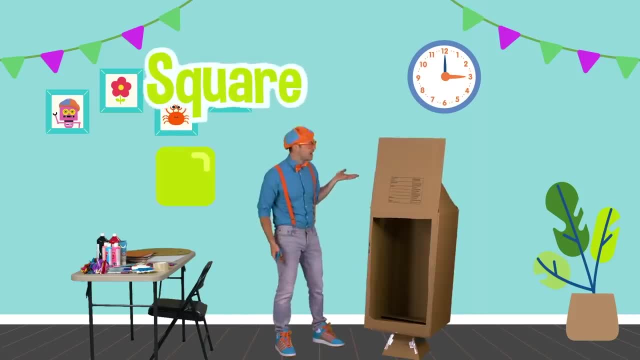 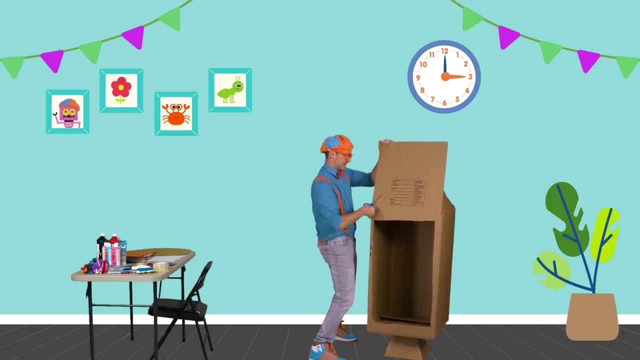 And do you see this? This is a square. Yeah, But we actually need to make it a triangle. So let's take our scissors. Yep, For your parents' grown-up supervision, You can cut this nice and carefully. Okay, One side is done. 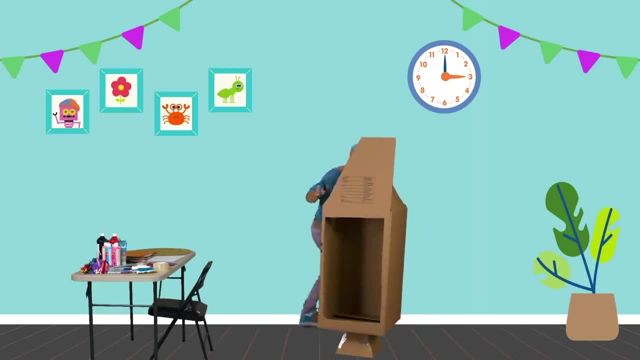 Now we need to do the other side. Here we go. Ooh, Look at that, It used to be a square, but now it's a triangle. Okay, Now we need some tape to then tape it to make the top of the rocket ship. 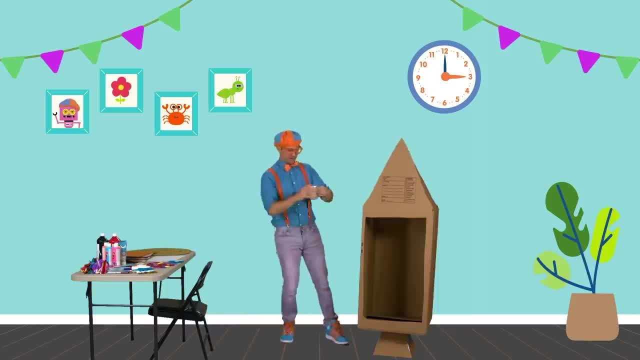 Okay, Here we go. Let's grab the tape, Pull off a big piece of tape, Whoa, All right, Let's give it a little slice. Okay, There we go. Whoa, Okay, Put that there. I love making things out of cardboard boxes. 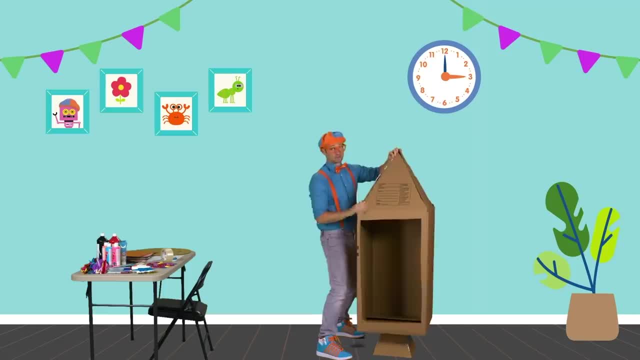 You can make so many things. Today we're making a rocket ship, But one time I made a monster truck. Another time I made a dolphin And I named that dolphin. Uh, what was that name? I think it was Dolphy. 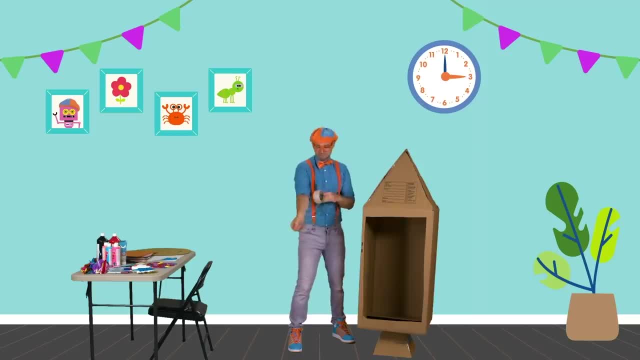 Whoa Whoa. Sometimes the tape gets stuck, but that's okay, We got it All right. There we go. Give it a little slice And then tape up the other side. Wow, Here we go. I am so excited to go into outer space. 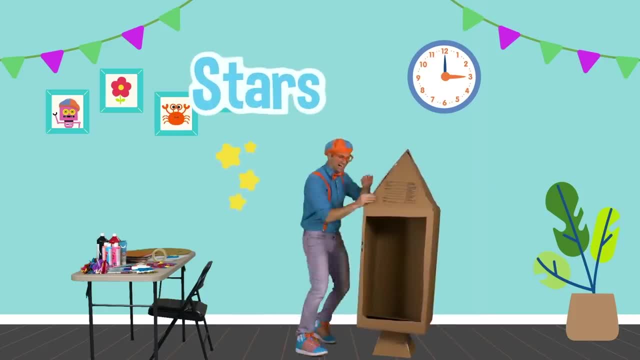 Have you ever seen the stars at night? Yeah, They're so bright. And the moon- I love the moon. Have you noticed that the moon sometimes is a full moon? Yeah, Sometimes it's a half moon And sometimes it's a new moon. 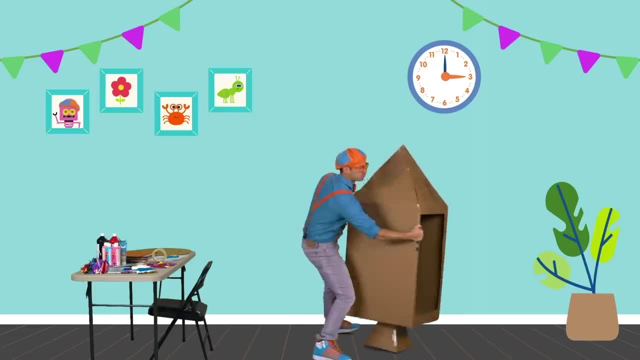 Yeah, Okay, Let's give this a little twist. Now it's time to design our rocket ship. I am so excited. This is one of my favorite parts. So the first step to design is to have a plan. Let's take this white piece of paper right here and let's draw the rocket ship. 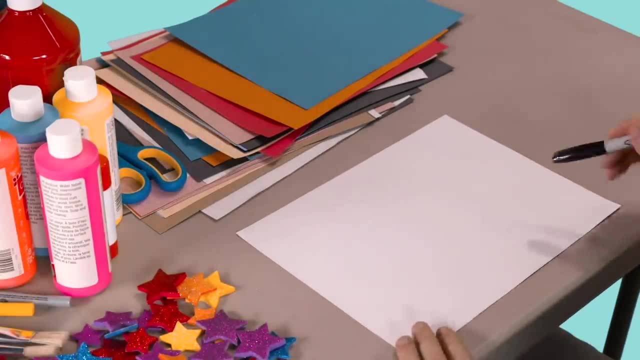 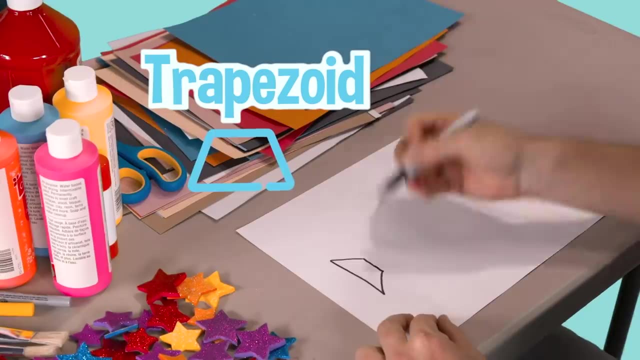 So the first thing you need to do is plan. Plan how the rocket ship is going to look. So let's draw the rocket ship. So we have a trapezoid over here, Then we have a big rectangle for the body of the rocket ship. 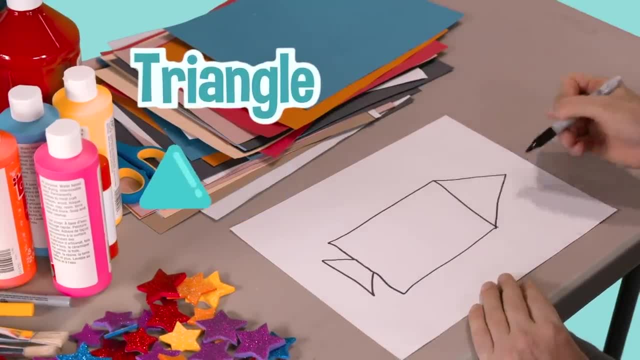 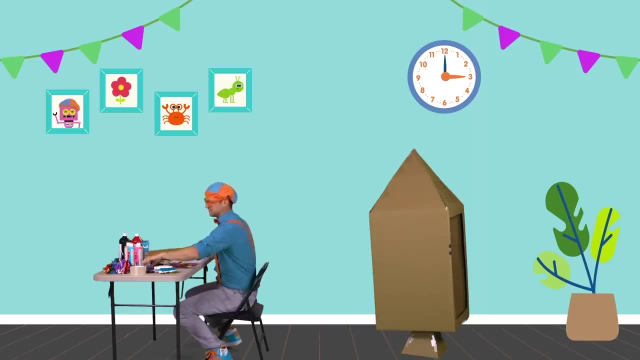 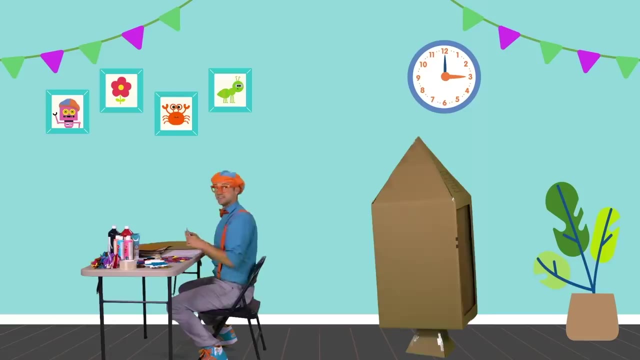 Then we have a triangle for the cone of the rocket ship And obviously I want a lot of color. So first let's take some orange- Perfect, I love orange. Then let's take some blue, So let's color it in. 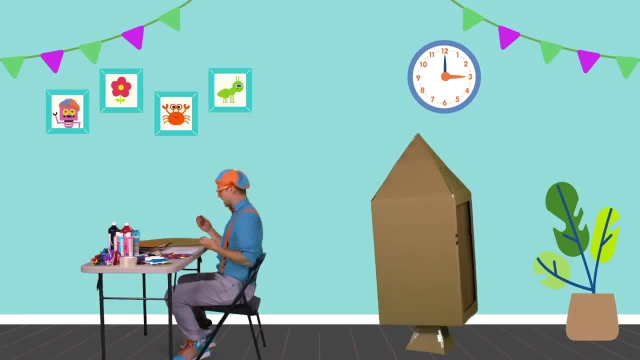 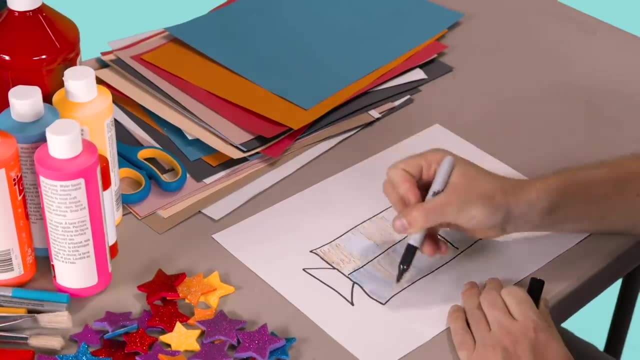 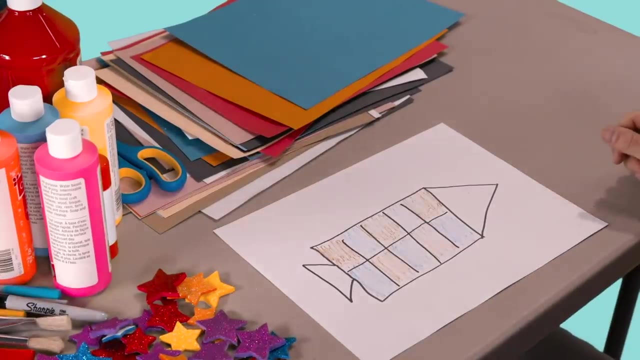 I have a plan. I'm going to use colored paper for that, So I'm actually going to use this black marker to symbolize that these are pieces of paper. We will do that later, All right, Oh whoa, There's a lot of stars here. 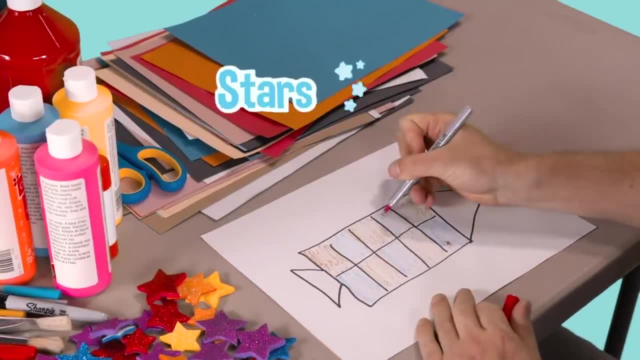 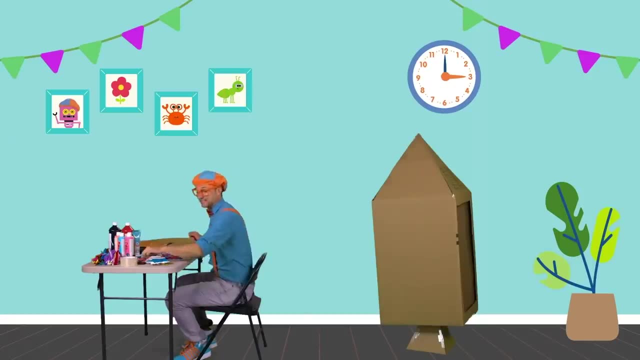 So let's actually, you know, make some stars right here. Yeah, Yeah, I love stars because you see them at nighttime when you look up at the sky And they twinkle. Yeah, Kind of like twinkle, twinkle little star. 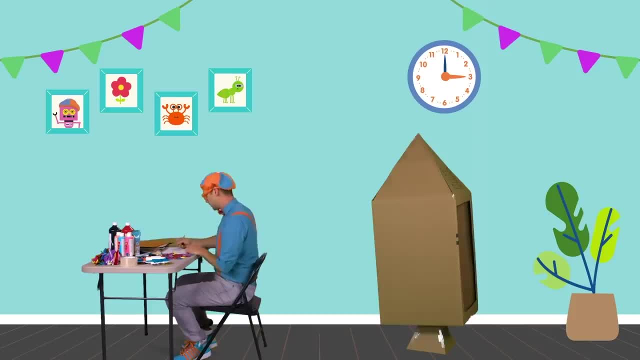 How? I wonder what you are. You know that song. I like that song too. Oh and yellow. Yeah, That's a beautiful color. Wow, Our rocket ship is looking so good. All right, I think I have a really good idea. 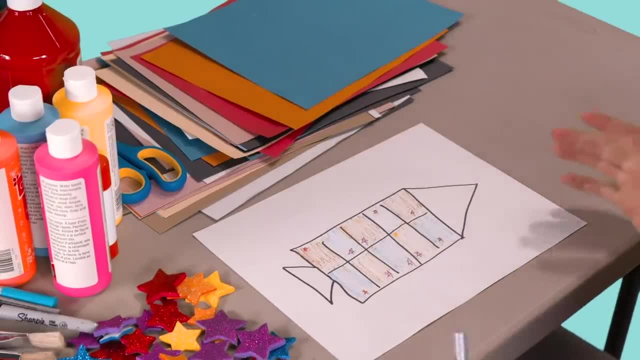 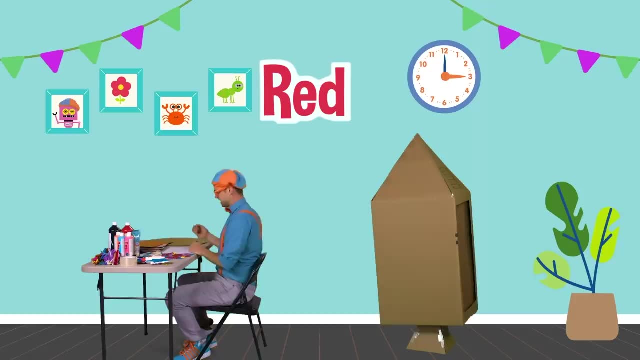 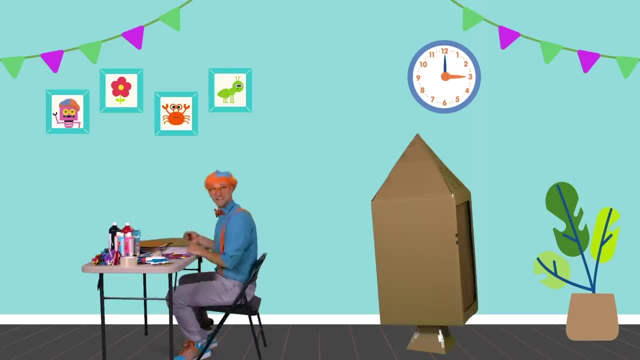 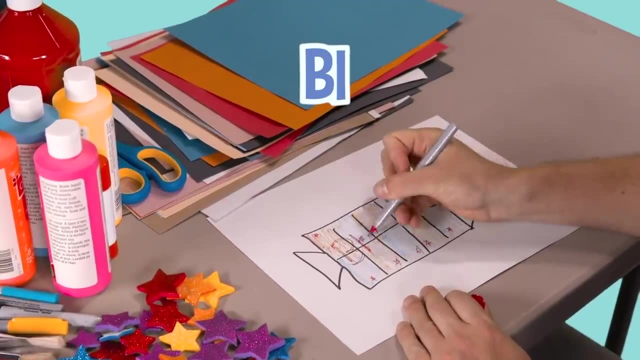 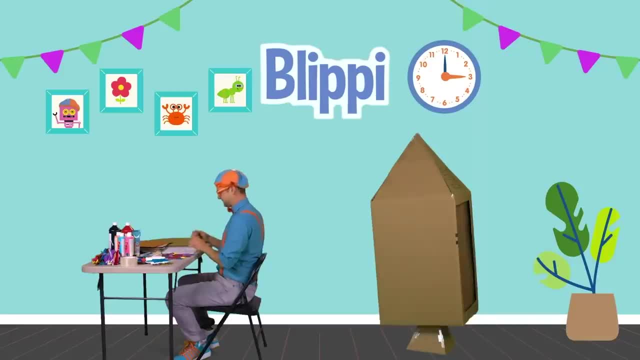 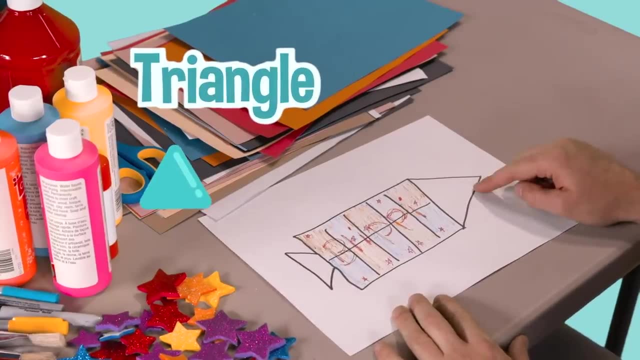 All right, That looks perfect. Can you say my name with me? Ready, E-L-I-P-P-I, Flippy, Perfect. All right, So that is the plan. Oh, looks like this triangle, the top of the rocket ship. 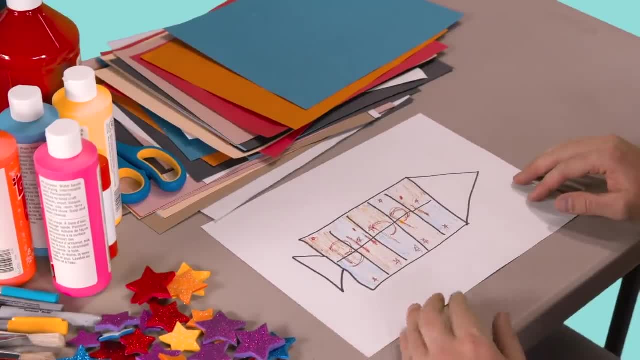 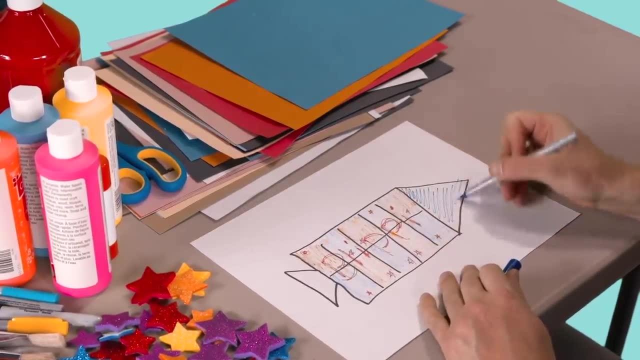 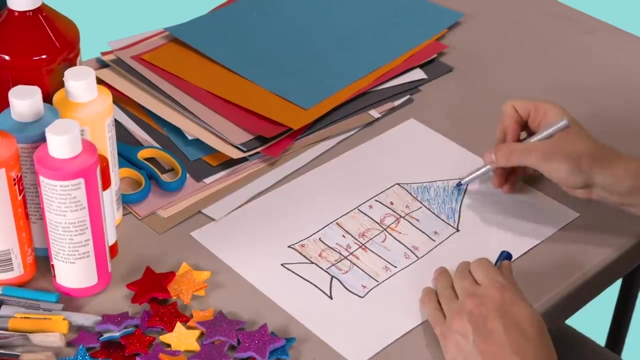 Yeah, We could color it. How about we color it? Yeah, blue, I like blue And we actually have a lot of blue paint on here, so we can actually just use blue paint for this part. Wow, perfect, I think, if we can make this rocket ship in real life. 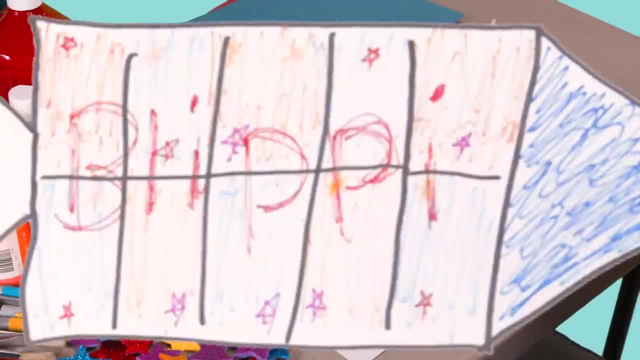 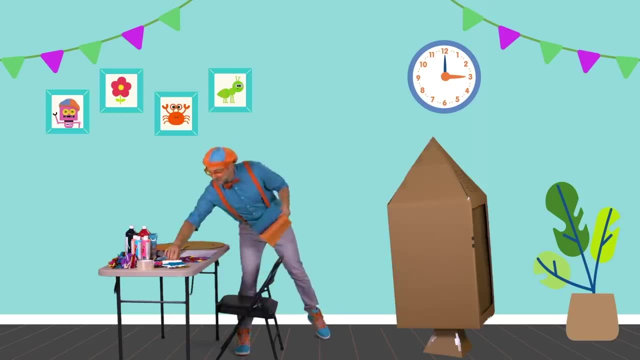 it's going to be so good, All right, here we go. All right, like I said, first thing we have to do is use the blue and orange colored paper to put on the side, just like this. So let's take the glue stick. 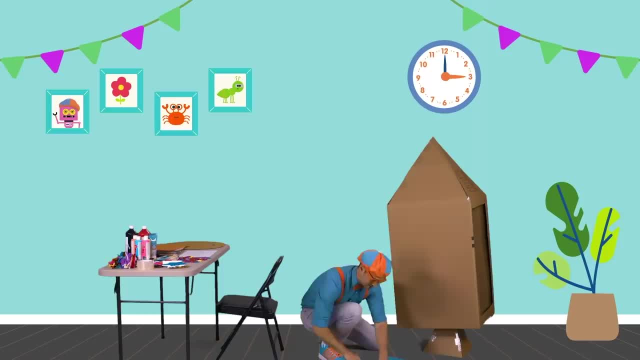 Yeah, yep, Put a lot of glue right on the backs, just like that. Okay, there's two pieces, Okay, there's one, And here's the second piece. All right, there's one, two pieces of paper. 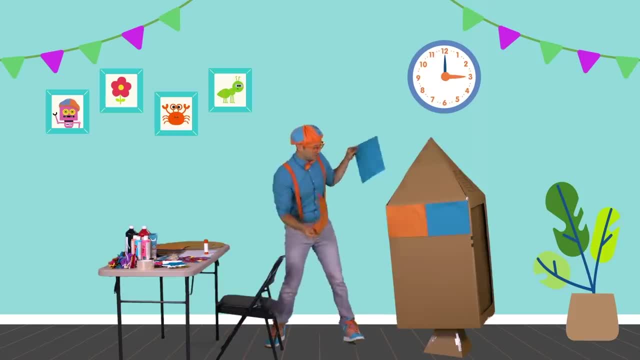 And we've got to do two more, Yeah, which will make one, two, three, four pieces of paper. I'm going to put the glue on them right over here. Okay, now we have four pieces: One, two, three, four. 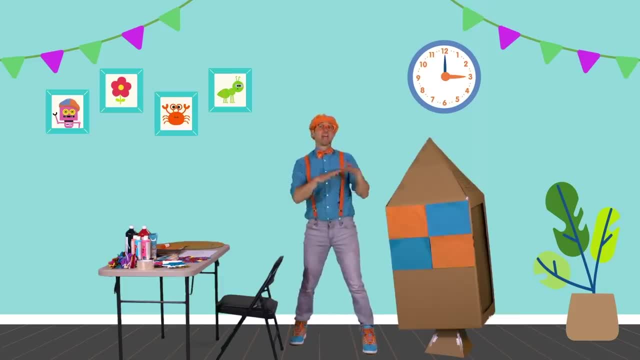 So let me finish the rest, and then we'll see how many we have in total after I'm all done. all right, Whoa, It's falling apart. Well, sometimes things fall apart, You just have to fix them. Okay, here we go. 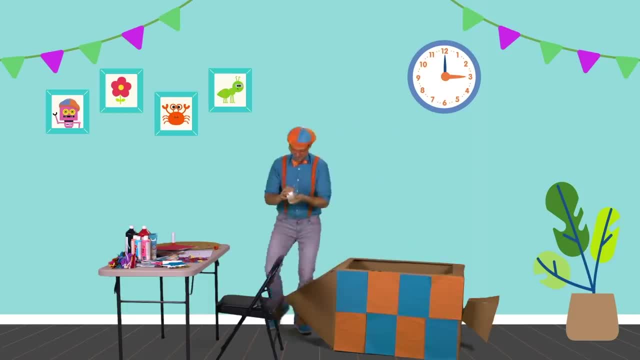 And after we fix this, then we can count all of the colors. So let's take our tape. All right, now the rocket booster is all fixed. Yep, there we go. Okay, now let's count all of the colored pieces. 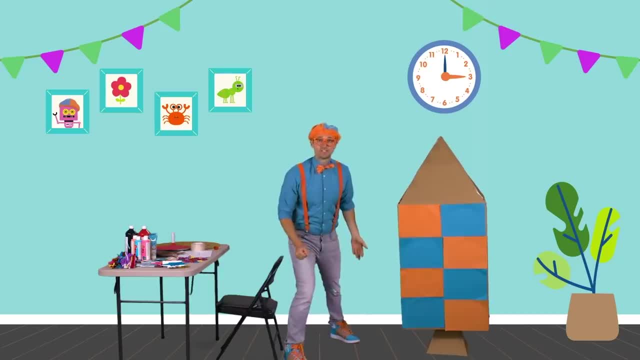 Yeah, the blue and the orange. Ooh and the orange pieces. Those are my two favorite colors. Okay, there's one, two, three, four, five, six, seven, eight, Eight pieces of paper. Good job. 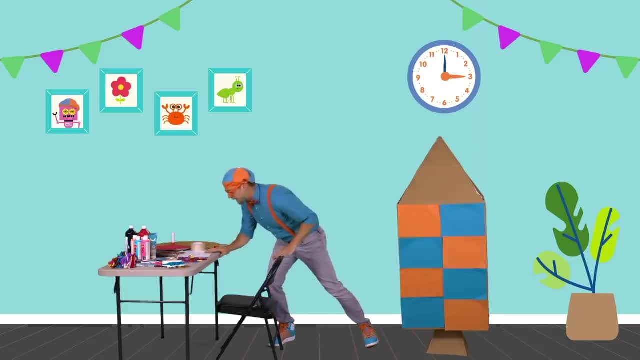 Okay, what else did we have on our piece of paper over here of our initial plans of our rocket ship to go to outer space? We had stars. Yeah, remember We had yellow stars, Yellow star, Another yellow star. Wow, They're so bright. 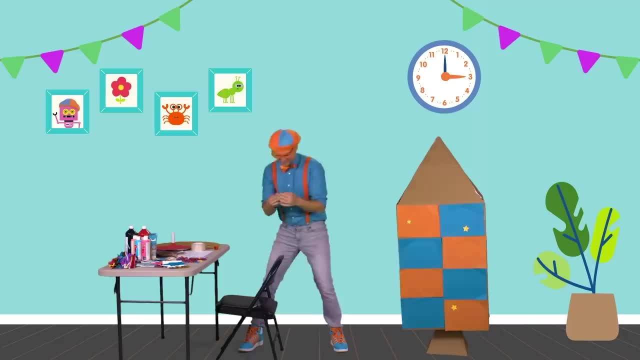 And they twinkle just like the real thing. Okay, and let's put some blue stars on there. Can you think of anything? that's the color blue My shirt. What about the big, vast blue ocean? Yeah, Here's another blue star. 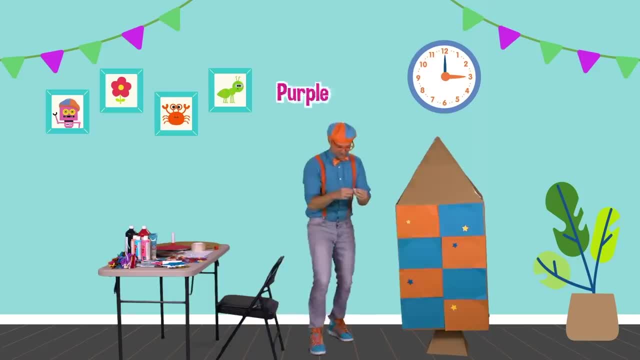 There we go. What about a purple star? A purple star, Yeah, I like the color purple Right there. And, last but not least, another purple star Right there. Perfect, That looks so cool. All right, So, as you remember, we have to spell my name on it. 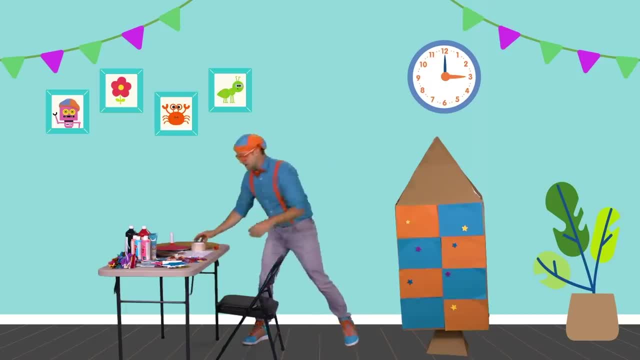 because that's what was on the plans. But before we do that, let's do the top of the rocket ship. Remember what color I said I was going to paint it? Yeah, the color blue. Okay, let's take some blue paint and my painter's palette. 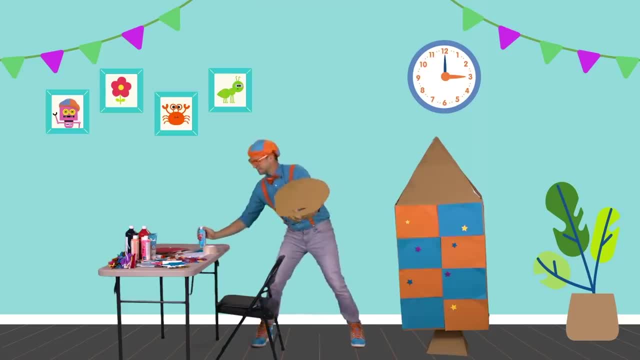 I'm an artist And let's take a paintbrush. Ooh, I love painting. Okay, let's squeeze some blue paint right on top. Whoa, Whoa, Whoa. That's so much fun. Okay, let's give it a little dab. 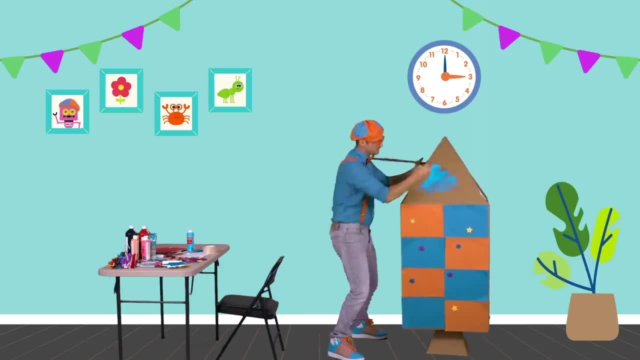 Let's do some painting. There we go. Wow, This is such a pretty blue. Wow, Whoa, Whoa. there we go. Have you ever used paints before? They're so fun. You can use a paintbrush and you can even use your fingers sometimes. 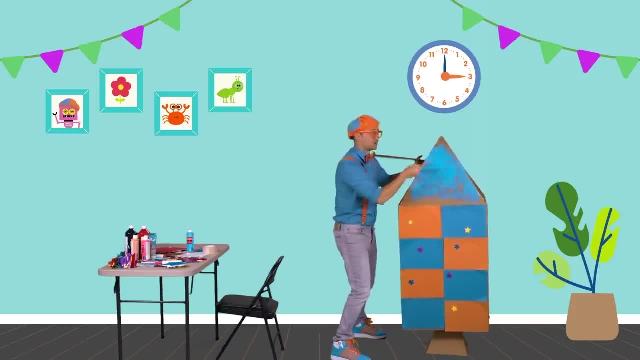 We won't do that today, but that art technique is called finger painting. There we go. How does that look? Do you like that? Yeah, I do too. Okay, let's put this away. You need to stay nice and clean and organized. 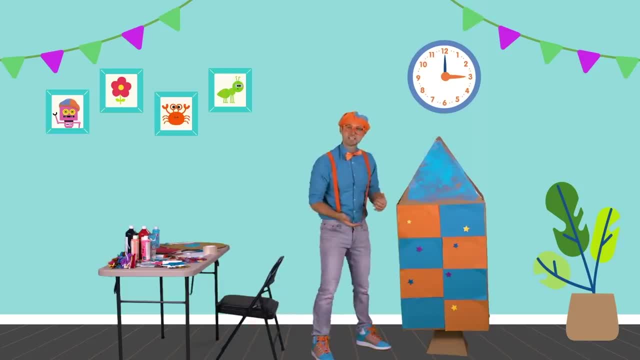 There we go And remember the last thing we needed to do. We needed to spell someone's name. Oh yeah, my name Blippi. Will you spell it with me? B-L-I-P-P-I, Blippi, good job. 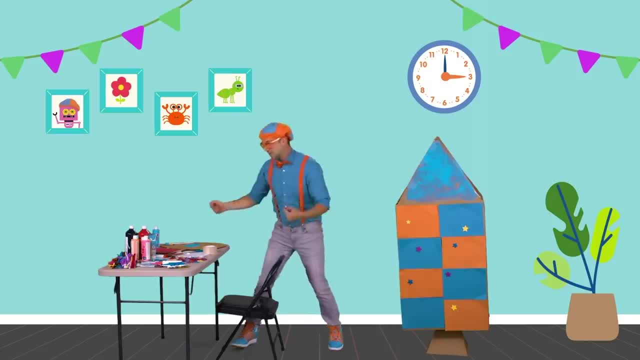 And do you remember what color? Yeah, the color red. Okay, so let's use a new paintbrush, Yep. And then we need to make sure we don't mix the red and the blue, because then it won't be red anymore. 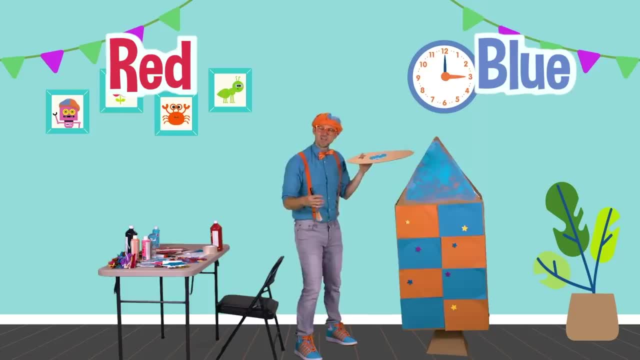 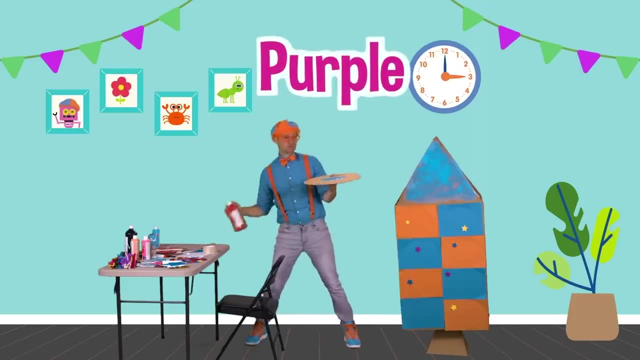 And it won't be blue. Do you know what color you get when you mix blue and red? Yep, purple, But we're going to keep them separate, So let's take this cap off. Oh, there is so much paint in here. 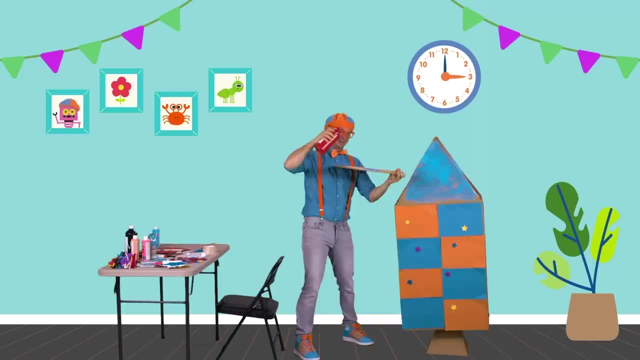 And I like to use a lot of paint. Whoa, There we go. Wee, Wow, a little bit more. All right, there we go. Okay, before we paint it, we should probably lay it down sideways, because we need to write my name. 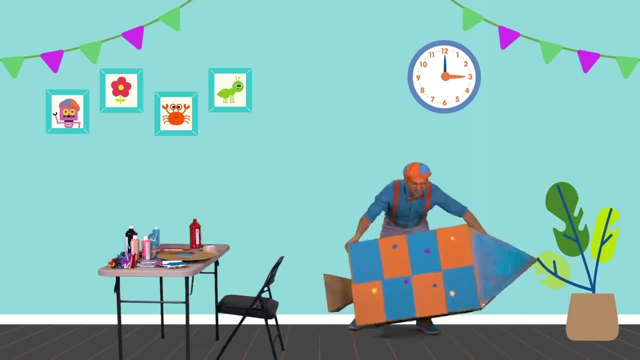 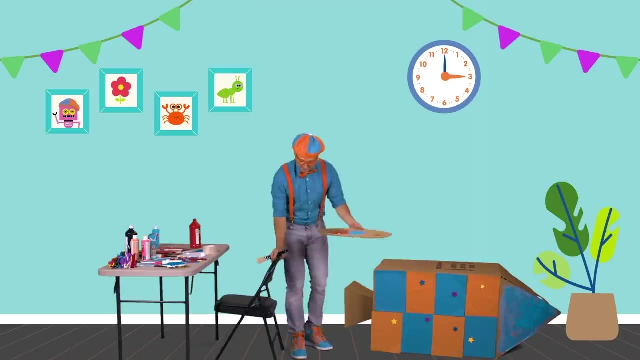 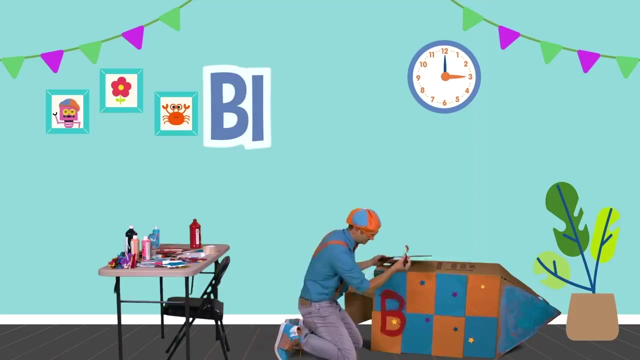 which is sideways. Yeah, there we go Like that. That's how we write sideways. Okay, let's take our paintbrush and let's put the letter B right here. All right, now that we have the letter B. the second letter is the letter L. 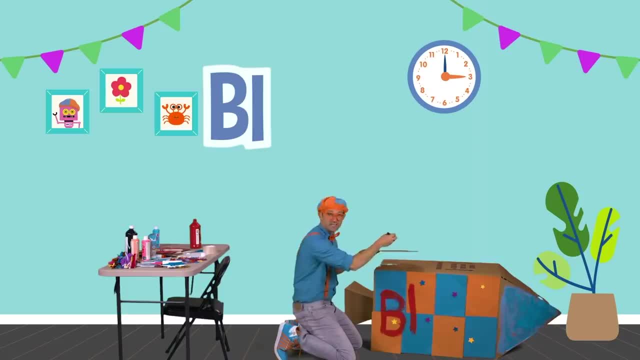 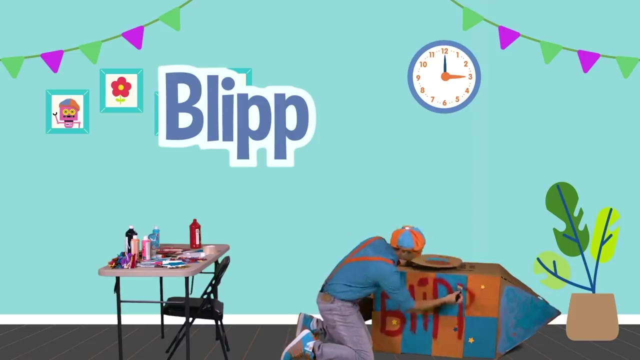 Yeah, just like that. The third letter is an: I Ready. Okay, there we go. B-L-I. You know the next letter, A P, yeah, B-L-I-P. All right, B-L-I-P-P. Yeah, here we go. 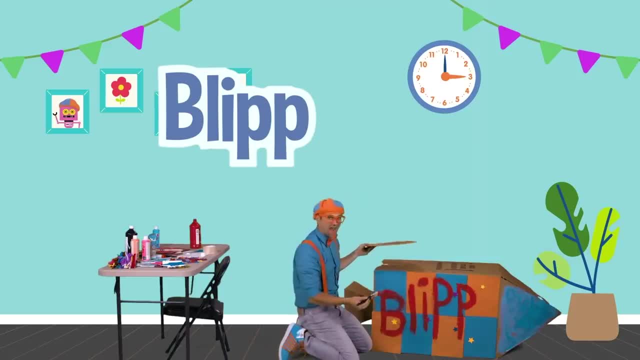 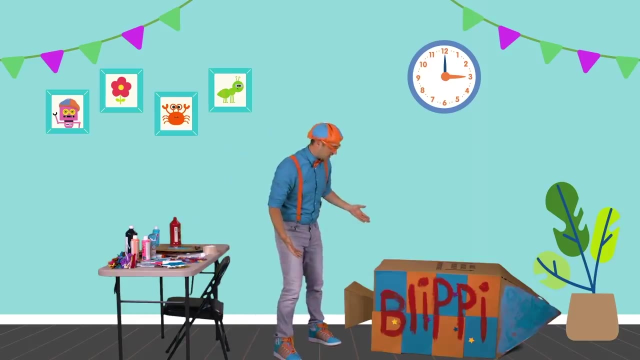 All right, one last letter: B-L-I-P-P-I Blippi. good job, There we go. We just completed the rocket ship, so now we got to get inside. Oh no, Do you see what I did? We're so silly. 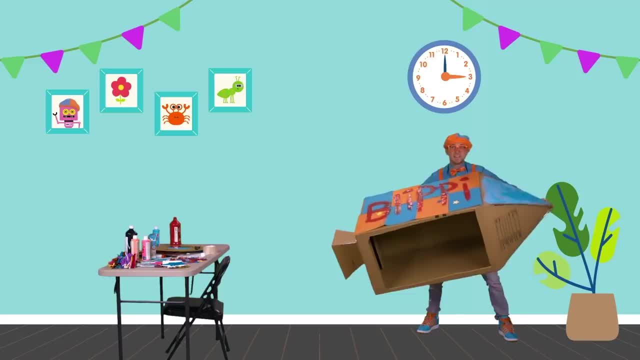 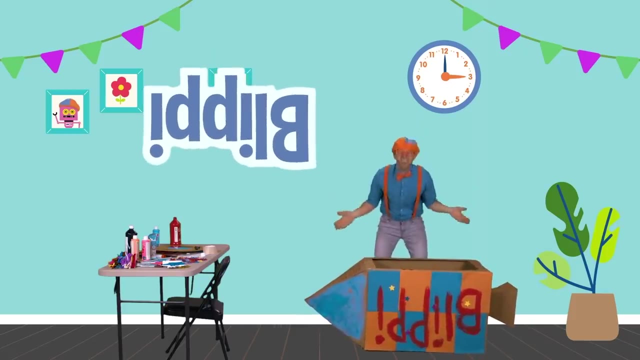 Check this out. The window is right there. Yeah, That means we have to twist it this way, See, And now my name is upside down. That's okay, though We're going to fly through outer space in this new cardboard rocket ship. 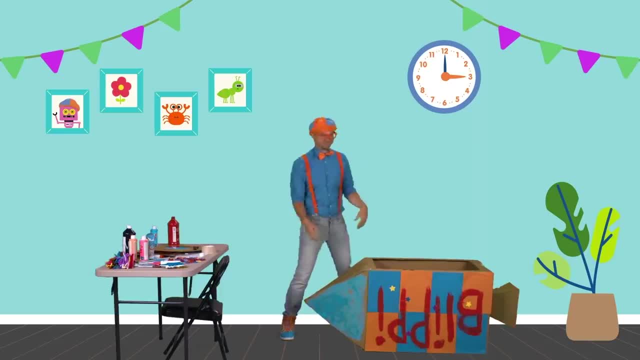 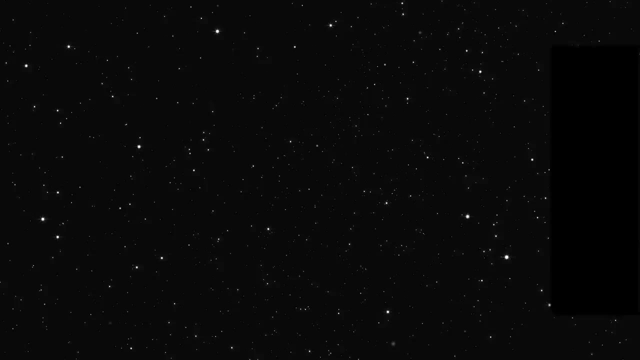 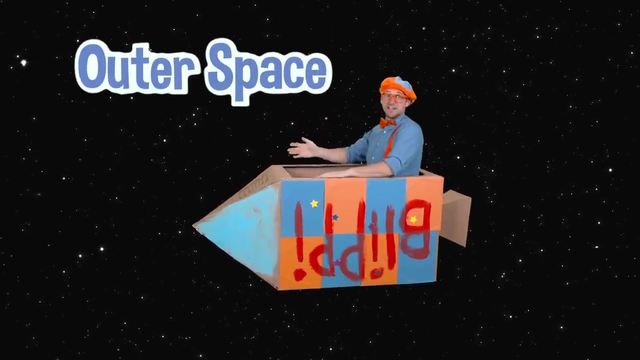 I am so excited with my name being upside down. So, silly, Are you ready, Because I sure am. Here we go, Whoa, Whoa, Whoa. Hey, I love outer space. Good job building the rocket ship with me. 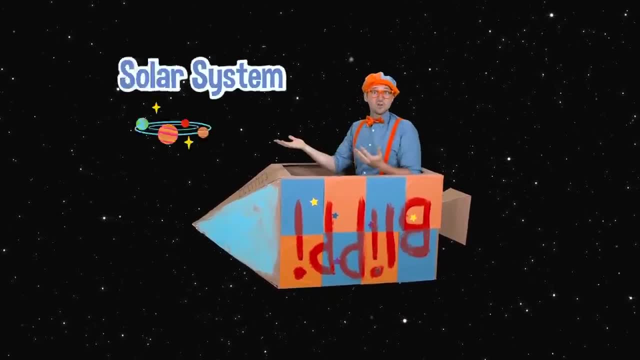 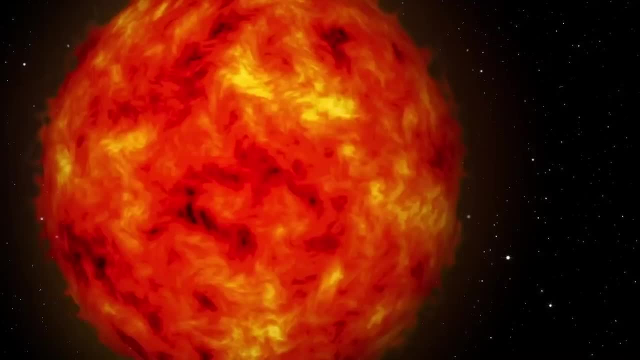 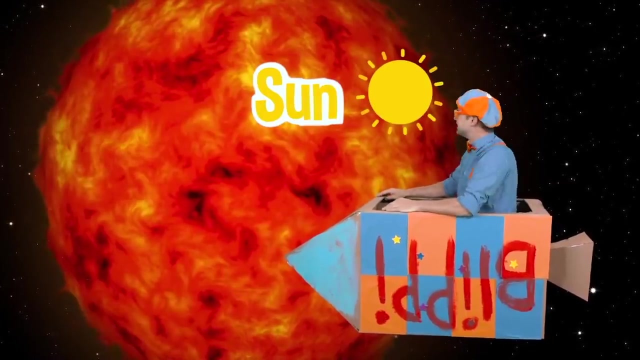 Now that we're in outer space, I think we should explore our solar system and learn all about it. All right, here we go, Whoa, Whoa, Whoa. Look at that, That is our sun, And its name is called the sun. 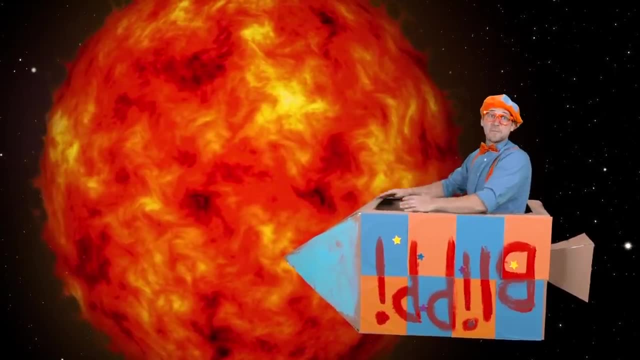 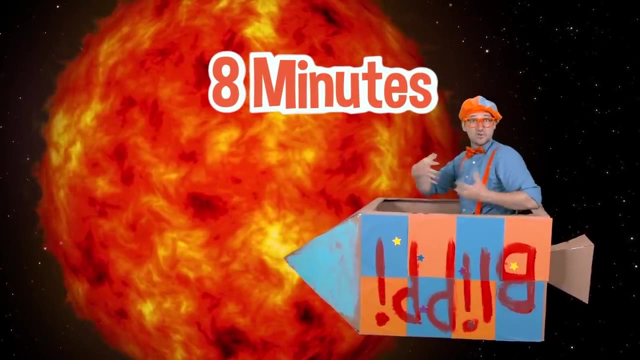 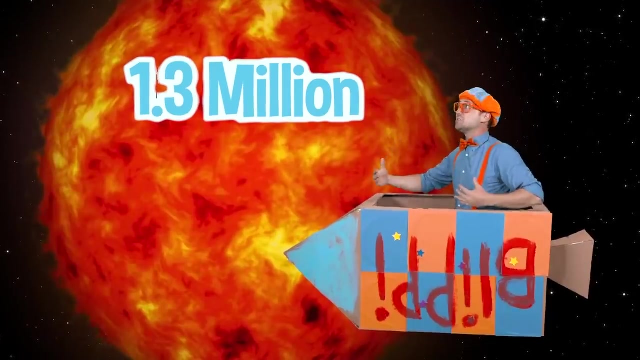 How original. Our sun provides all the light in our solar system And that light takes eight minutes to go from the sun to our planet Earth. And the sun is so big: there's 1.3 million Earths that can fit inside of it. 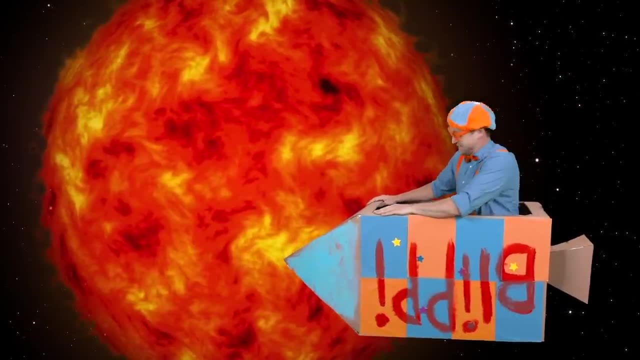 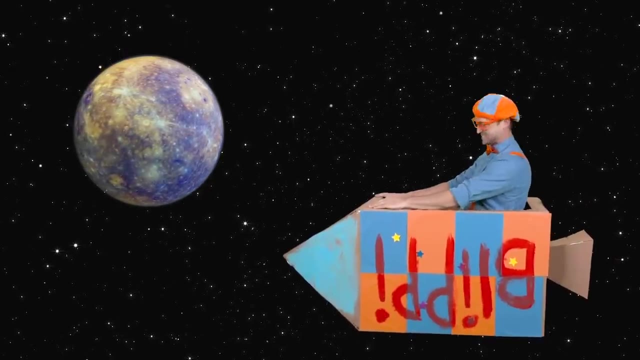 Whoa, That's a lot of Earths. Here we go, Woo-hoo, Whoa, Whoa. Outer space is so much fun. Oh, look at that planet. That planet is Mercury. Wow, That planet is really rocky. 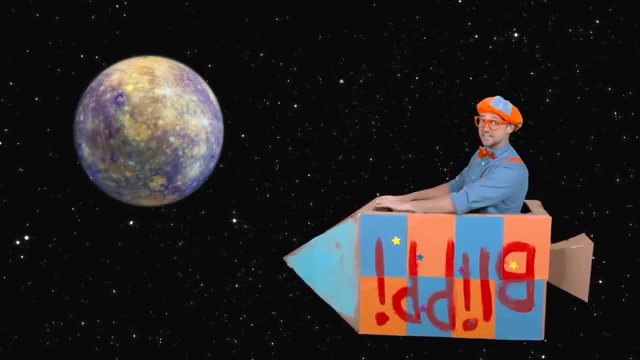 And there's so many craters on it And actually, since it's the closest planet to the sun, one rotation around the sun is super fast. It's only about 88 days on Earth. Whoa, Whoa, Whoa. 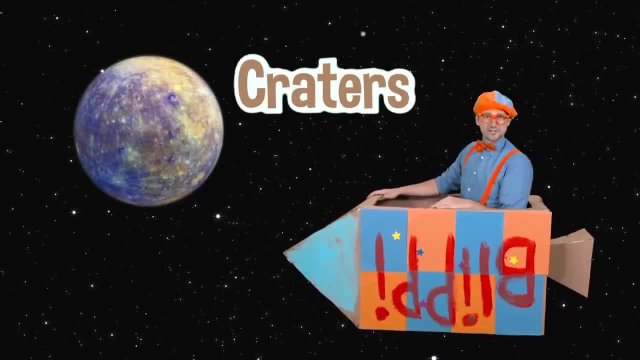 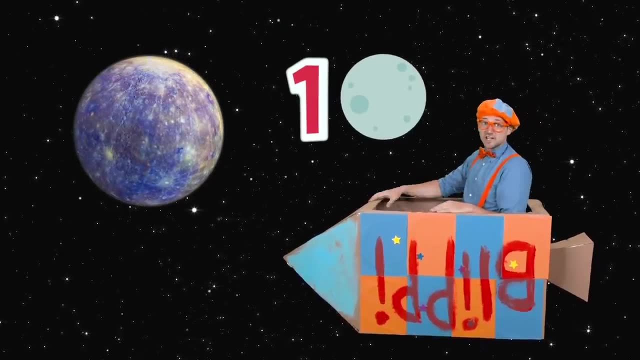 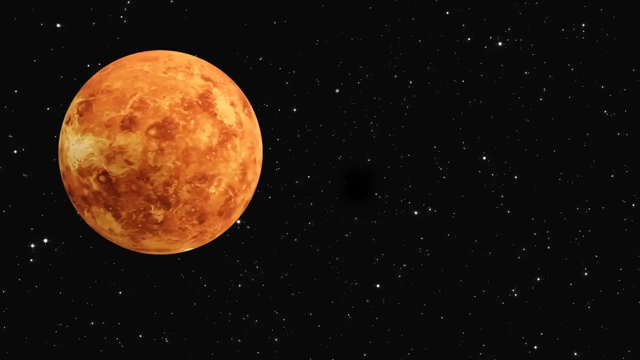 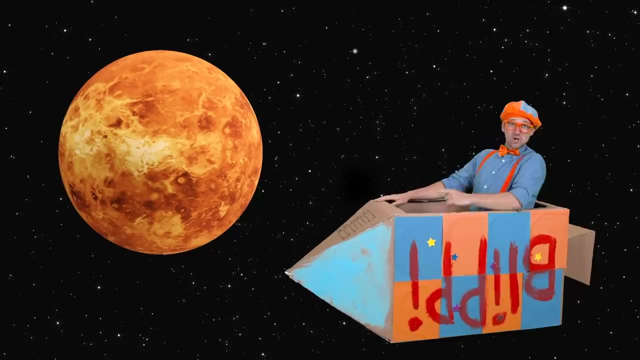 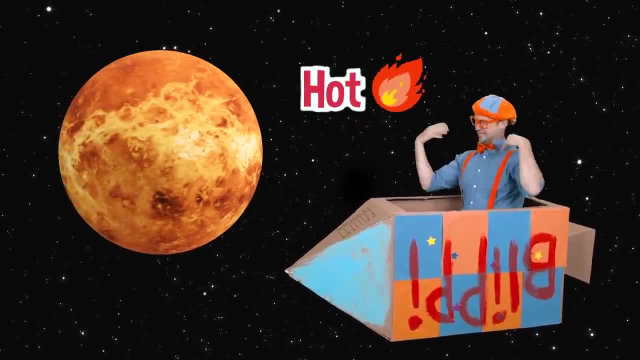 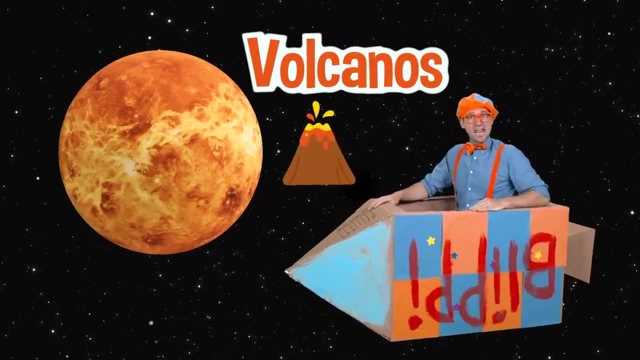 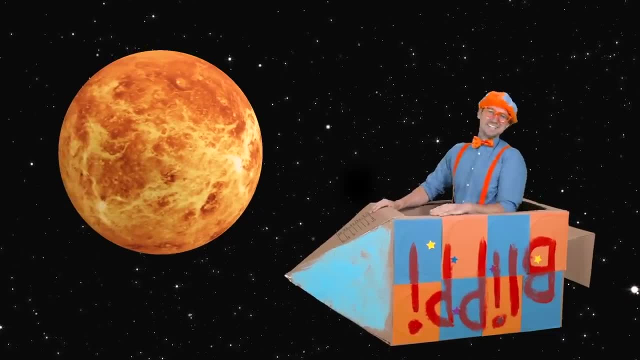 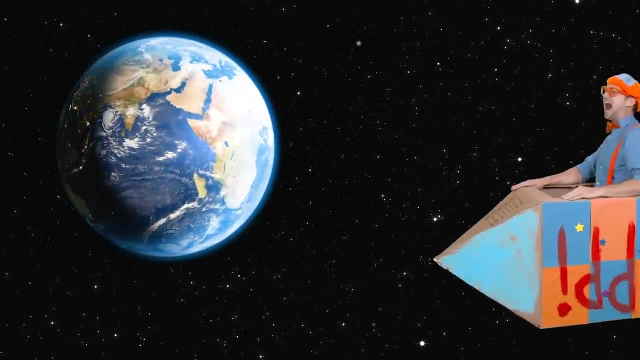 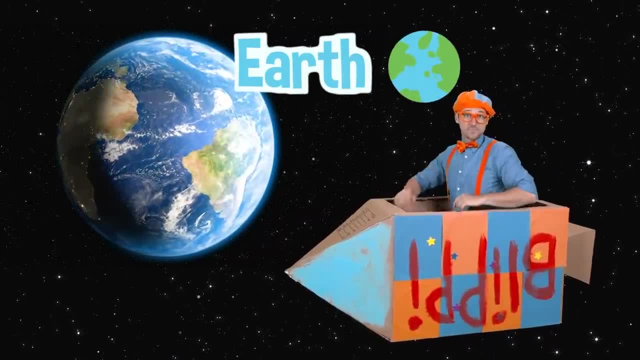 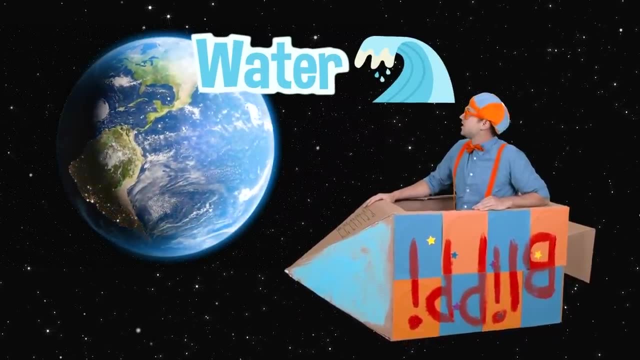 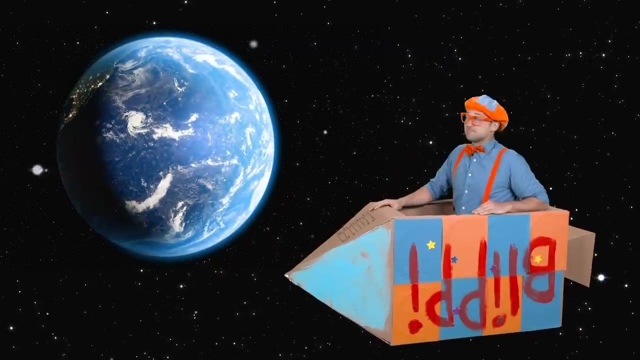 Whoa, Whoa, Whoa, Whoa, where you and i live. wow, what a beautiful planet. there's so much water there, and then there's a lot of trees and mountains. whoa, and our planet earth. yeah, we have one moon. let's head there now. 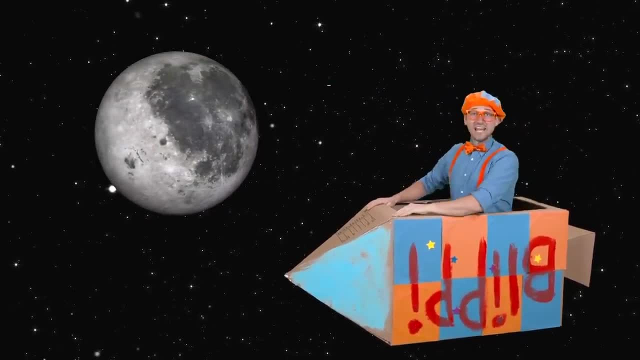 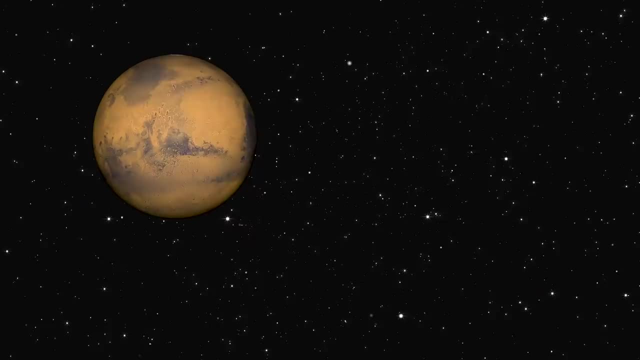 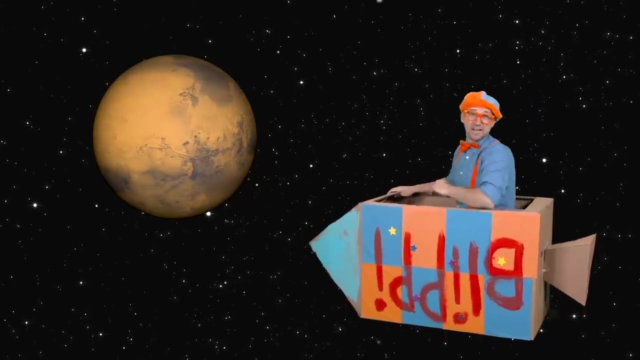 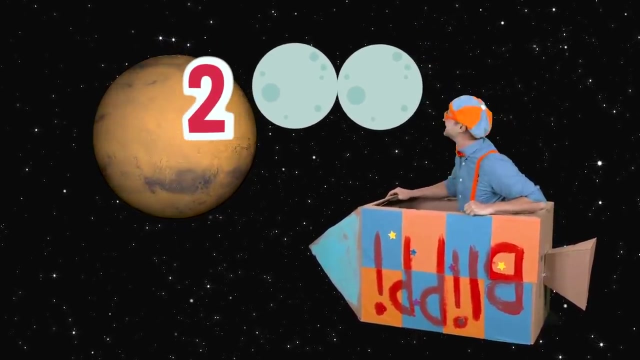 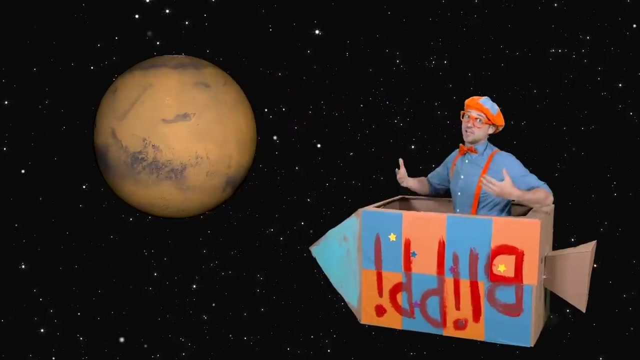 hey, moon, thank you so much for lighting us up at night. another planet, yeah, oh, that planet is the planet mars. whoa, it has two moons. wow, what a lucky planet. well, we've actually sent robots and rovers to mars. that is awesome. us humans have yet to land on mars. 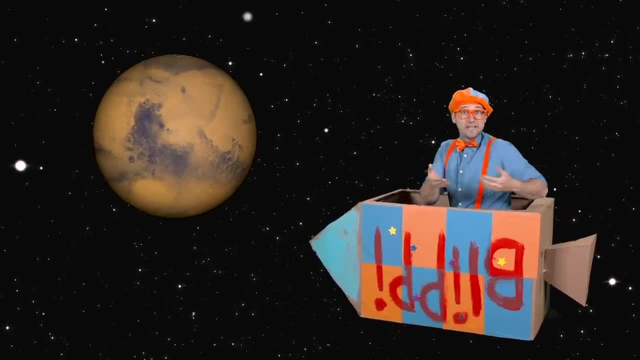 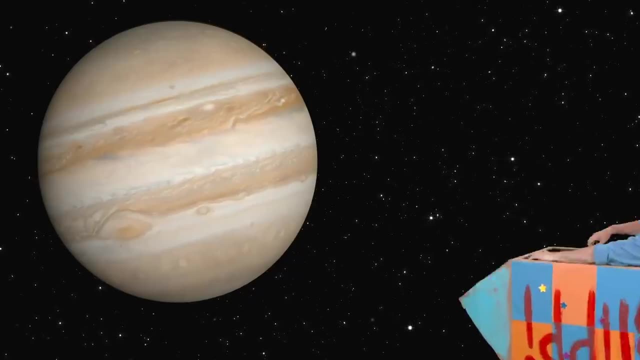 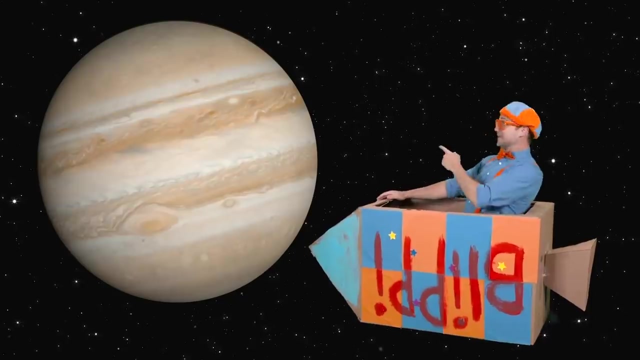 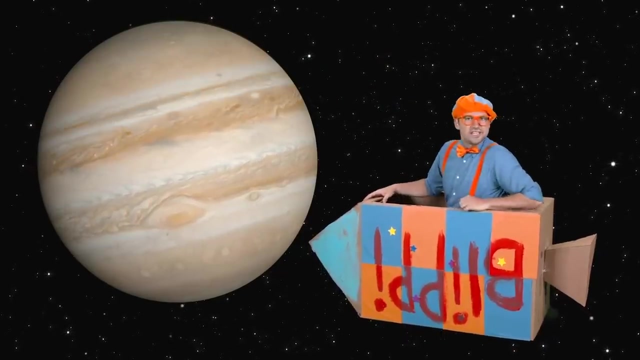 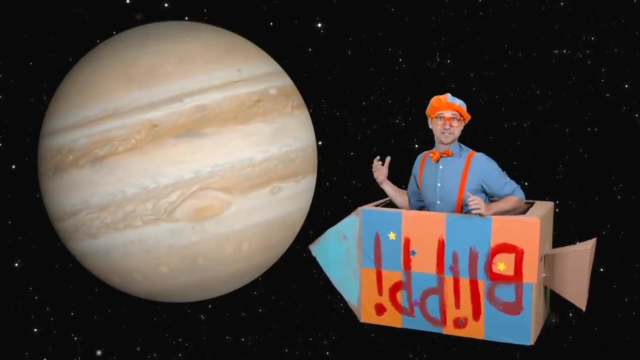 ourselves. but maybe someday soon, maybe you'll be that astronaut. yeah, here we go. that asteroid belt was so intense, whoa. and look at that. that's our planet, jupiter. it's the biggest planet in our solar system. and do you see that big red dot? that is a storm, whoa, that's a big storm. and 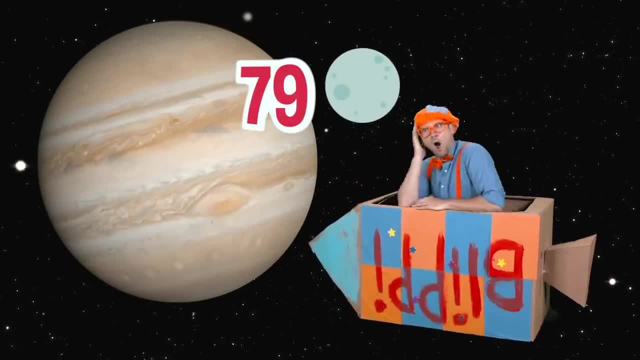 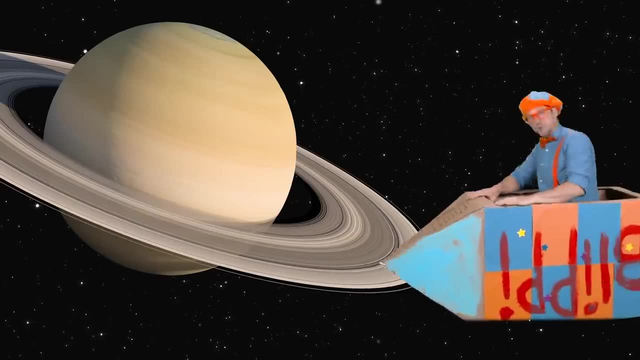 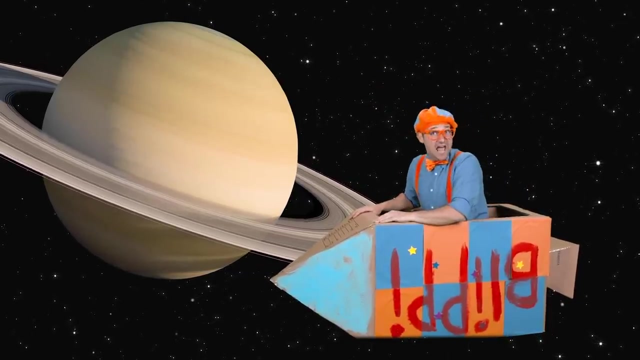 Jupiter actually has 79 moons. That's crazy. Whoa, Woo-hoo. See you later, Jupiter, Hello, Saturn, Check it out. This is our planet, Saturn. Whoa, what are those? Those are Saturn's rings. 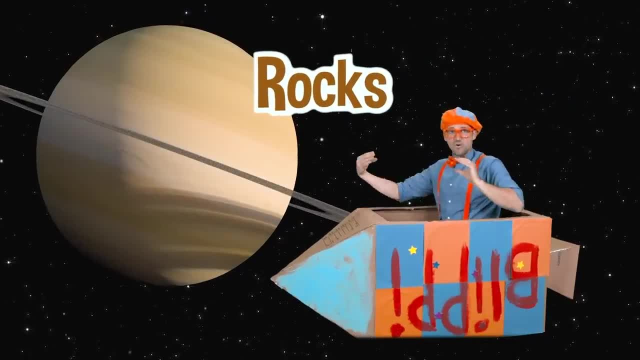 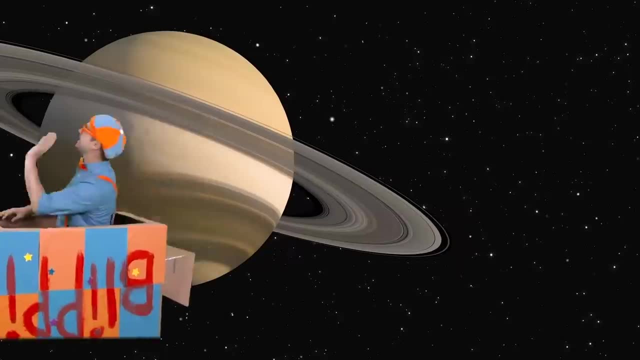 Wow, there's so much dust, ice and rocks that form those to make up those rings. Wow, what a cool-looking planet. All right, Saturn, see you later. Bye-bye, Ha-ha, Wee-hee. 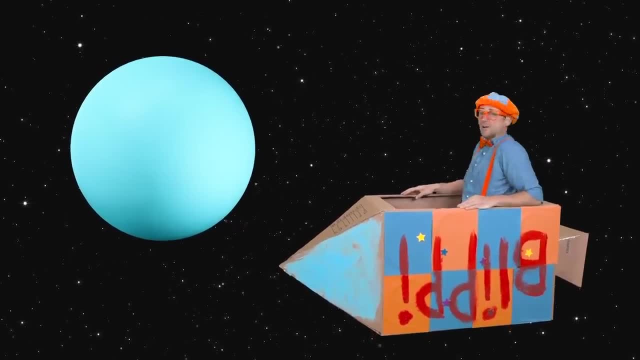 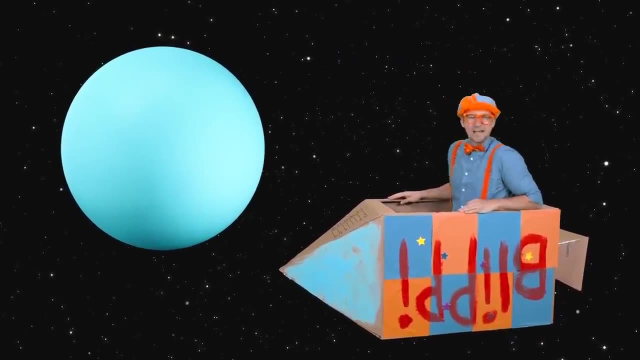 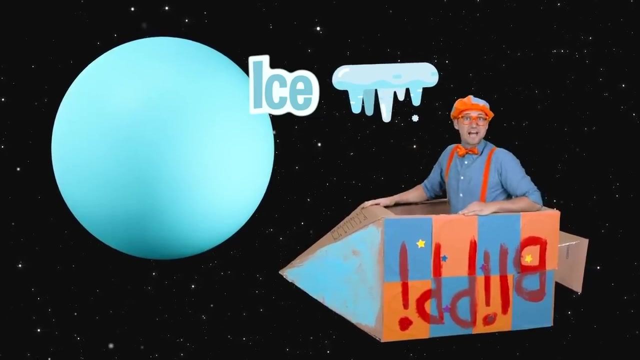 Ha-ha, Whoa. Oh, look Another planet That is Uranus. Yeah, what a cool planet. Wow, it's kind of blue-looking, huh. Yeah, that's because there's so much ice on it. It's known as the Big Ice. 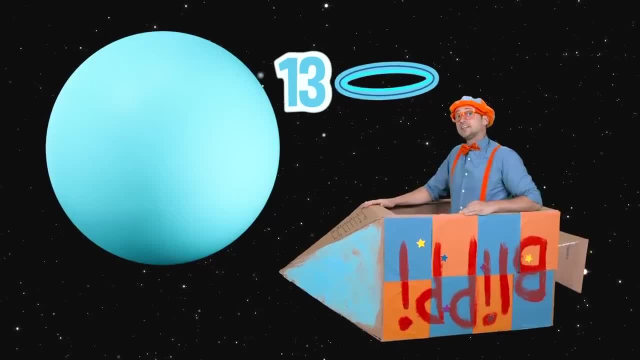 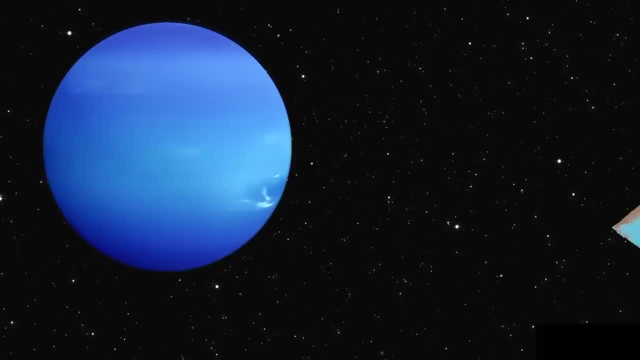 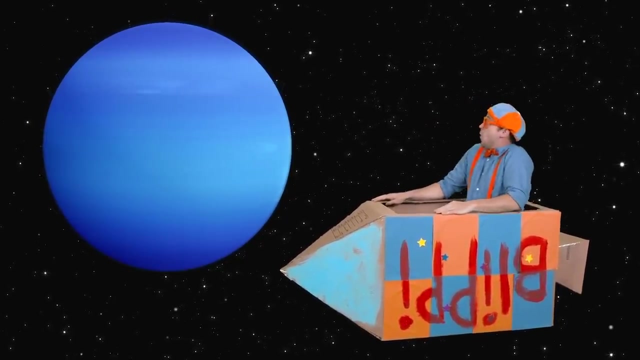 Whoa, it has 13 rings and 27 moons. All right, see you later. Uranus, Bye-bye, Whoa, Whoa. Yeah, This has been so much fun. Whoa, look at that planet. That planet is the planet Neptune. 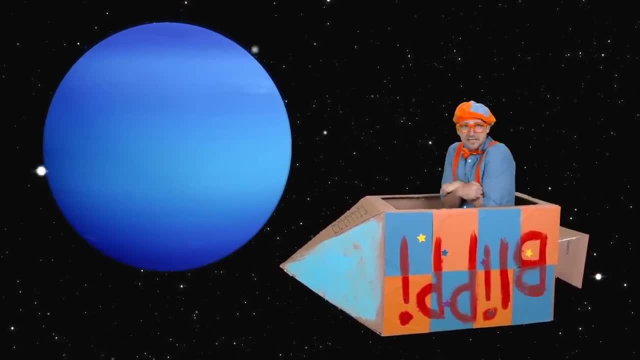 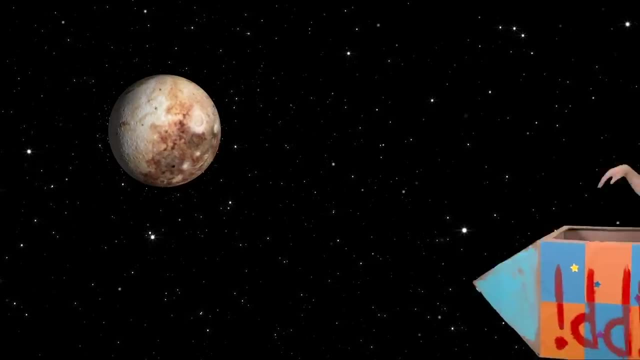 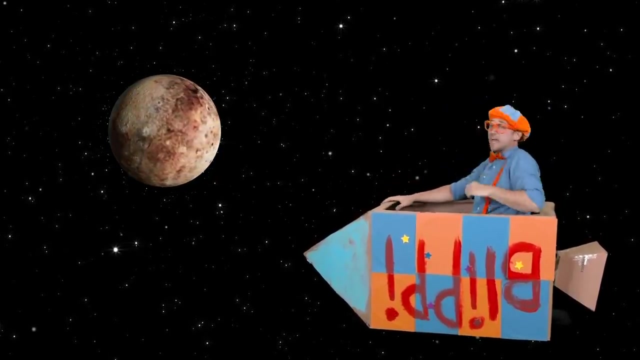 It's so dark, cold and windy on that planet. Whoa, Whoa, Let's get out of here. Whoa, Whoa, Woo-hoo-hoo. The last planet on our solar system. Look at it, It's really small. 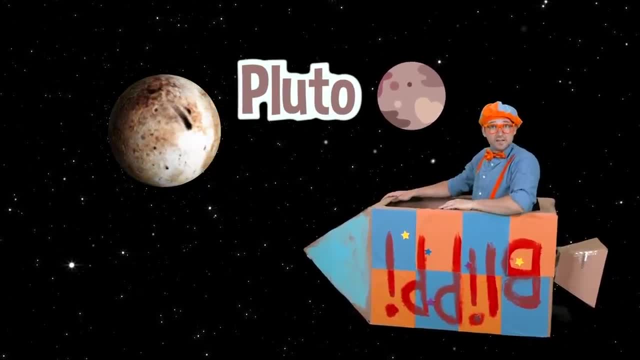 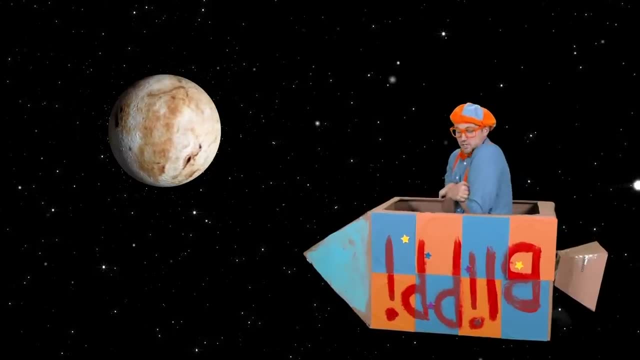 That is Pluto. It's so small, it's a dwarf planet, Wow, and it's really cold. I love Pluto. Ha-ha-ha, Brr. It's really chilly out here, though Let's turn around and count all of the planets. 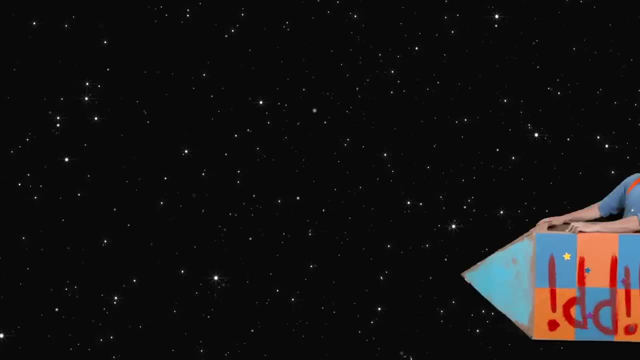 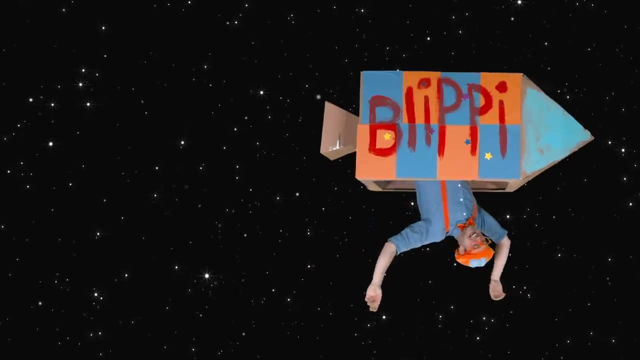 Shall we? Whoa, Woo-hoo, Yay, Whoa-o-a-a-a-a. Oh, whoa, I'm upside down, But now look at my name. Woo-hoo-hoo, Ha-ha, Whoa. 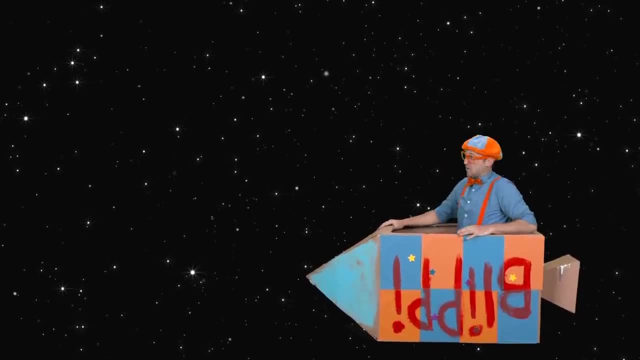 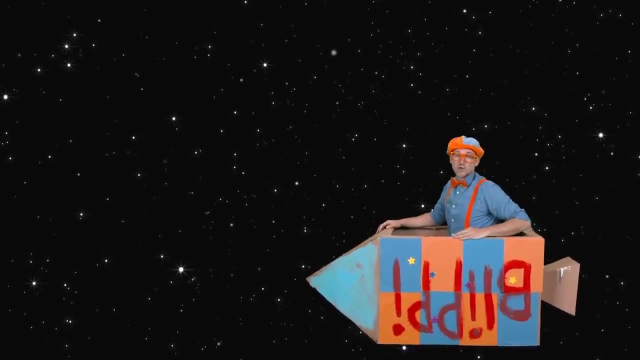 Whoa, That was so much fun learning about all of the planets in our solar system together. Hey, I think we should count all of them, Okay, Okay, The sun isn't a planet. The sun isn't a planet, Okay. 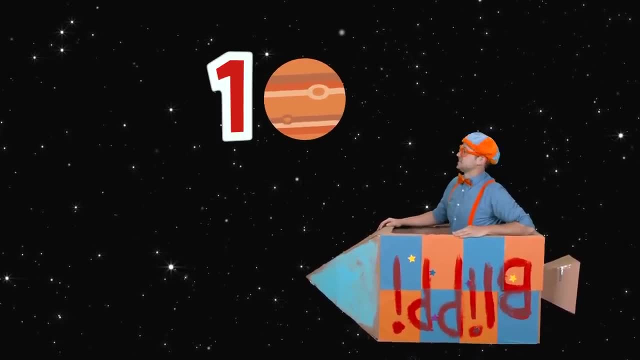 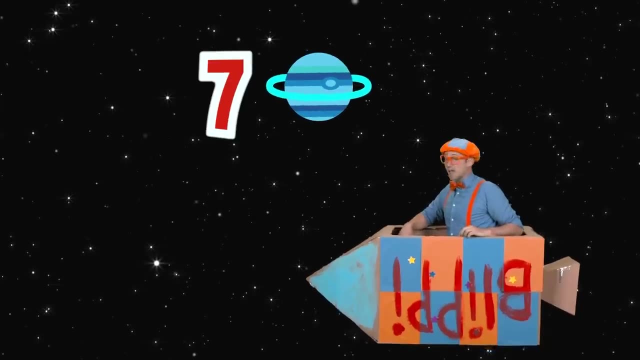 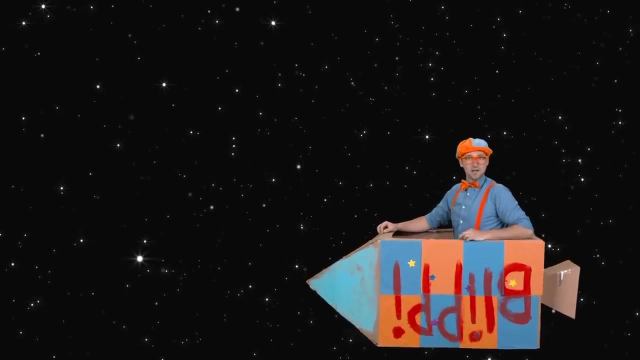 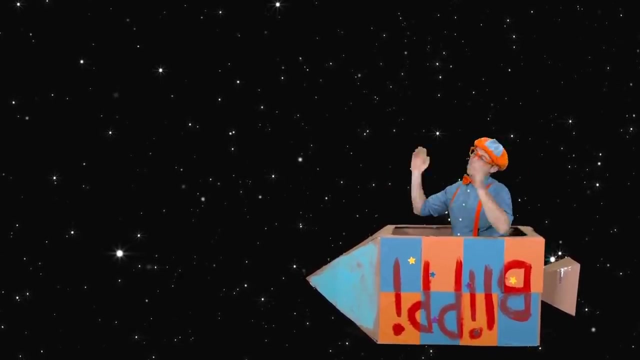 Okay, planet. so let's count the planets: 1, 2, 3, 4, 5, 6, 7, 8, 9. oh wait, a second, 8, 9, ah, who knows? some people say Pluto's not a planet, but I don't know. it's all up in.